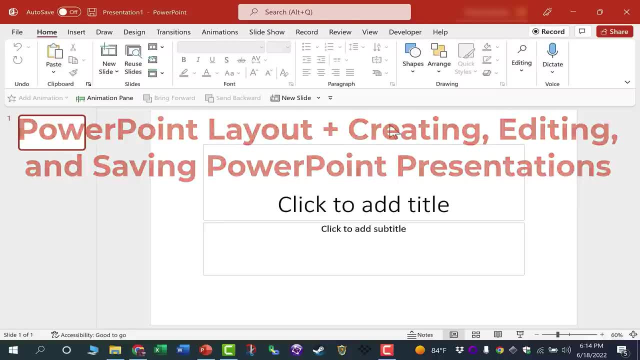 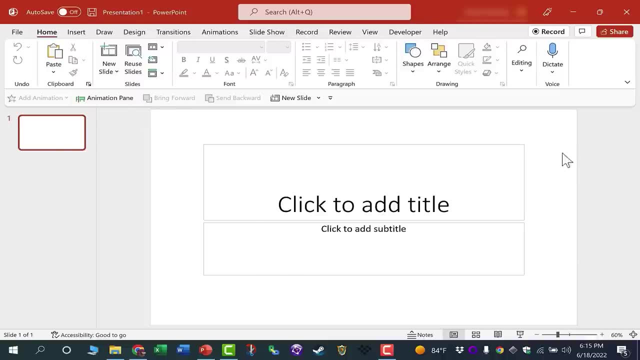 add slides to a presentation and how to save your presentation. The first thing we need to cover is the layout in Microsoft PowerPoint. So when you're in PowerPoint, what you're looking at here toward the center of the screen is your title slide, your first slide. This is a bigger view of it. 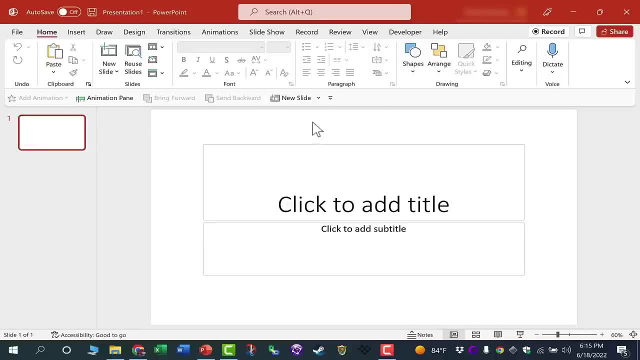 and then over here at the left we have a thumbnail version of the same title slide, And those two things put together take up the majority of the screen space that we have in PowerPoint. But let's look at the rest of the layout because it's really important In PowerPoint. 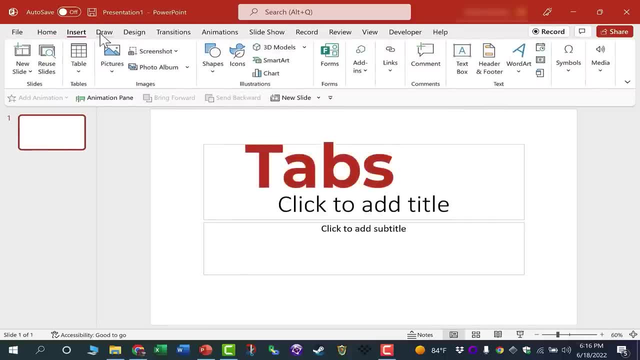 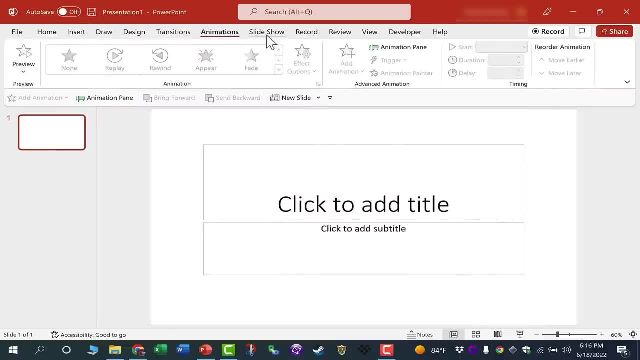 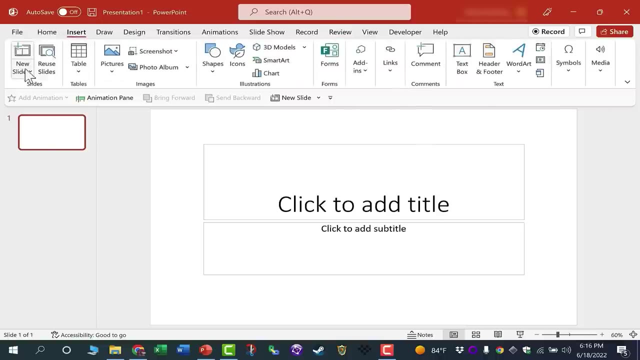 if you look at the top of the screen, you'll see that we have several tabs. We have the Home tab, which is one of the most commonly used tabs. We have the Design tab, Animations tab, Review tab and more, And when you click on a tab, the tools that you see here change. This area of the layout is. 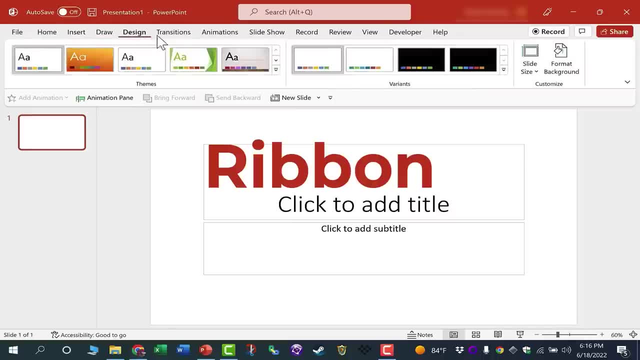 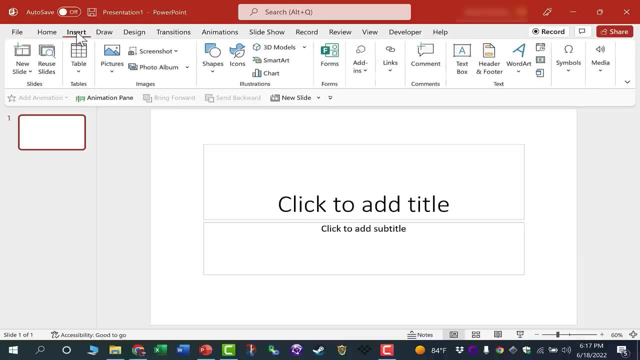 called the ribbon, and there are different ribbons that become visible when you click on a tab. So the terminology that we use in PowerPoint is that when you click on a tab, let's say the insert tab, then the insert ribbon becomes visible. 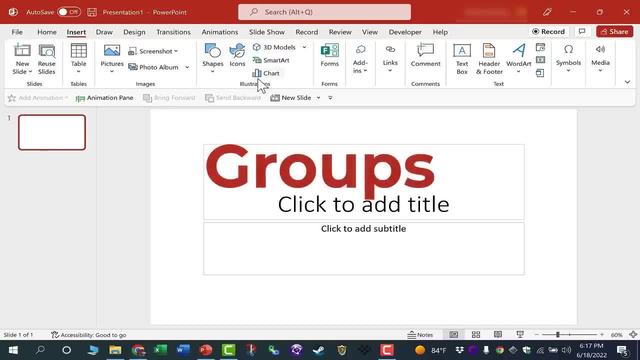 and the insert ribbon is divided up into groups. So we have an illustrations group, we have an images group, tables, slides, comments, text and more. Now, in some cases, Microsoft wasn't able to fit all of the options into the small space provided here. 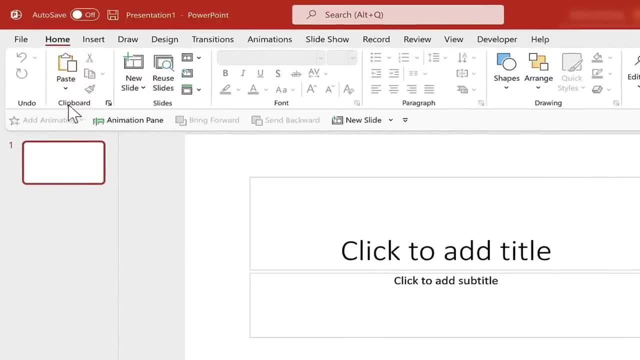 on the ribbon and in these individual groups, So for example in this clipboard group, there's only just a little bit of space provided, so Microsoft hid some of the additional options in this button here. This is called the clipboard dialog launcher. I like to just call it the launch button. 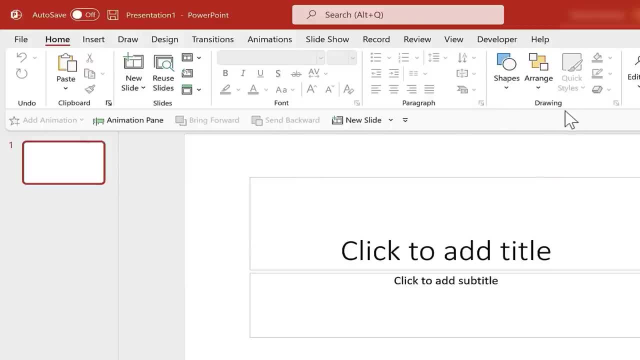 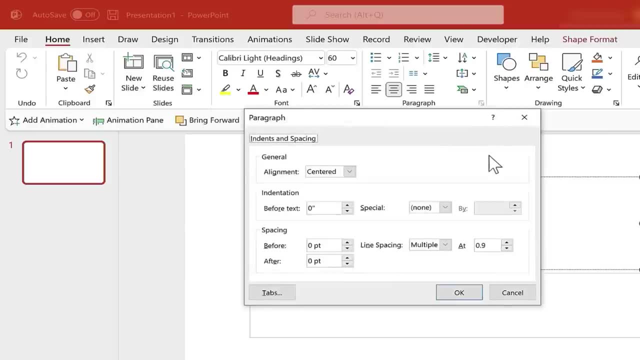 And you can see over here, the paragraph group also has a launch button. so does the drawing group. Whenever you see a launch button and it's black, you should know that you can click on it to get additional options that don't fit in the provided space on the ribbon. 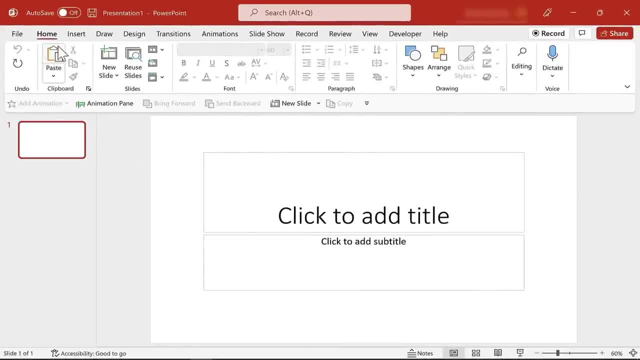 In addition to my title slide and its thumbnail here at the left, and the tabs, the ribbons, the groups and the launch buttons, it's important to also be aware of a few other layout features Notice. here in the upper left we have a quick save button. 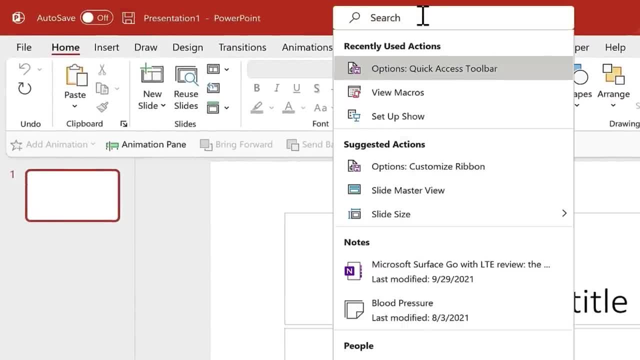 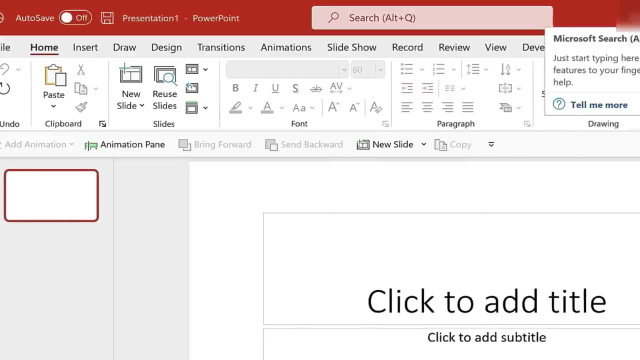 Here at the top we have a search bar or search button and we can use that search to search for options, settings and for other help in using Microsoft PowerPoint. Over here in the upper right corner we have the close button. You can click this to close out of PowerPoint. 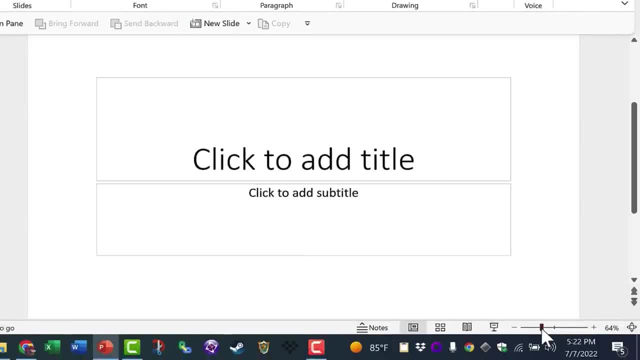 when you're ready to stop using it. In the lower right corner we have a zoom slider. You can click and drag this slider bar to the right to zoom in on a particular slide. You can click and drag it to the left to zoom out. 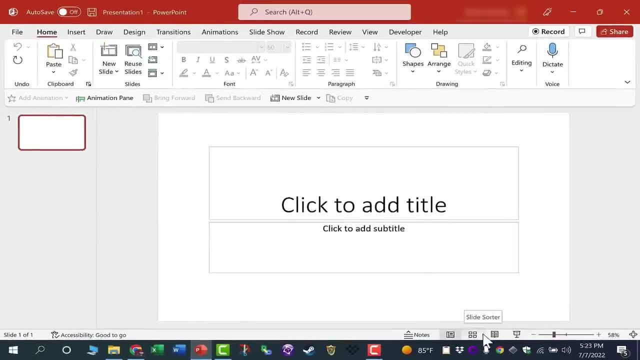 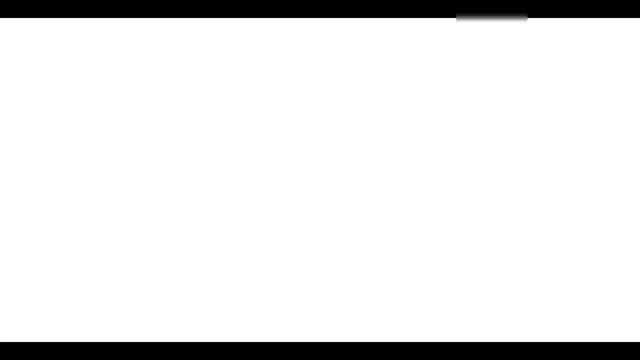 Just to the left of the zoom slider. we have different views that we can use in Microsoft PowerPoint. This view here is slideshow view. When you click that- the presentation page, the presentation begins. I'm gonna tap escape on the keyboard to get out of presentation mode. 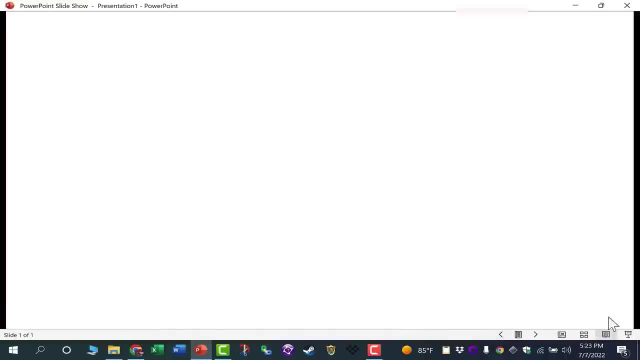 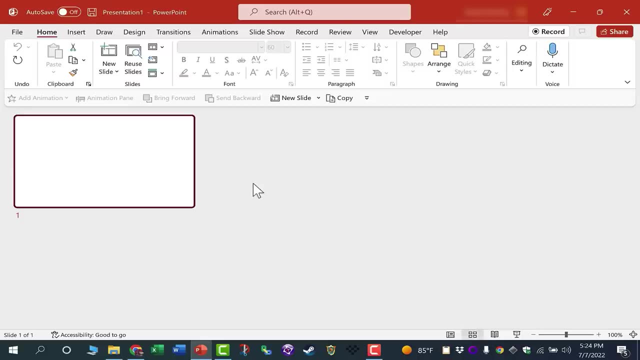 Just to the left of that we have some other views. We have reading view that focuses just on helping us read the text in the PowerPoint. We have the slide sorter view that helps us to get the big picture of our presentation, to see each slide and maybe to reorder those slides. 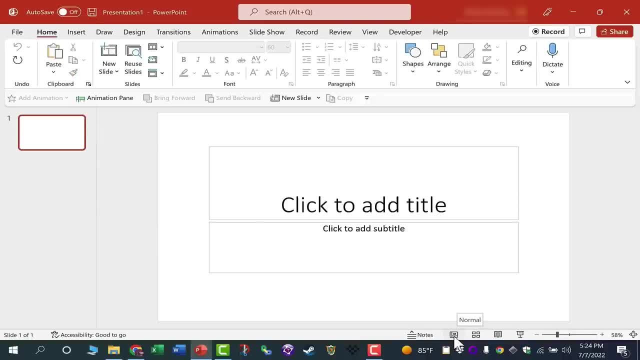 And then, finally, we have the normal view that most people use when creating their PowerPoint. Just to the left of that, you can also click on notes and it lets you type in presenter notes. Only the presenter will be able to see those notes once the PowerPoint is started. 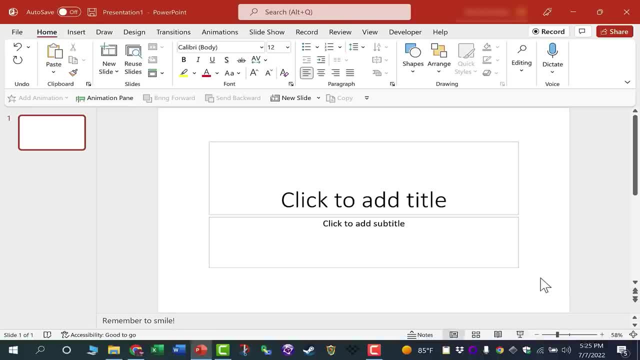 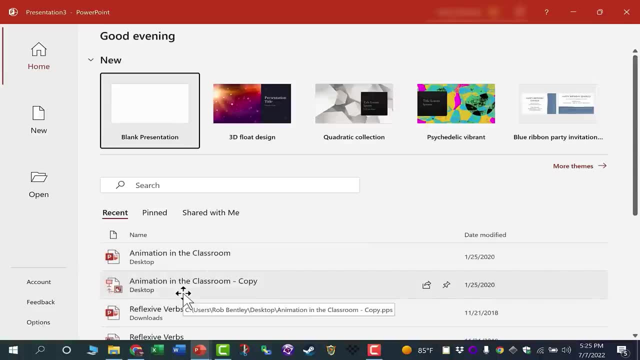 Now that you've learned the layout in Microsoft PowerPoint, let's look at how to create a new blank presentation. Whenever you open up Microsoft PowerPoint, you're taken to a screen that looks something like this. Here I have a list of documents that I've recently used. 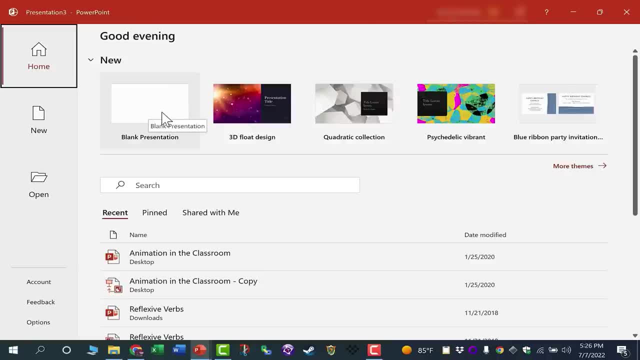 Up here at the top, I have a button that I can use to create a brand new blank presentation, and that's what I'm going to do, but I also want you to be aware that there are some pre-made themes that you can use. 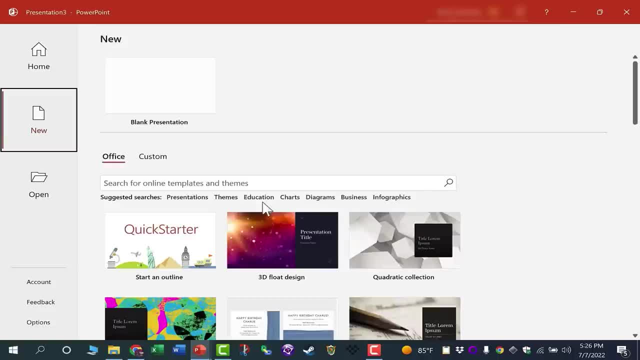 kind of like templates, and you can click here to get even more themes and also to search for some online themes. So that's definitely worth checking out. You can just take those themes and adapt them for your own uses. But for now I'm just going to click on blank presentation. 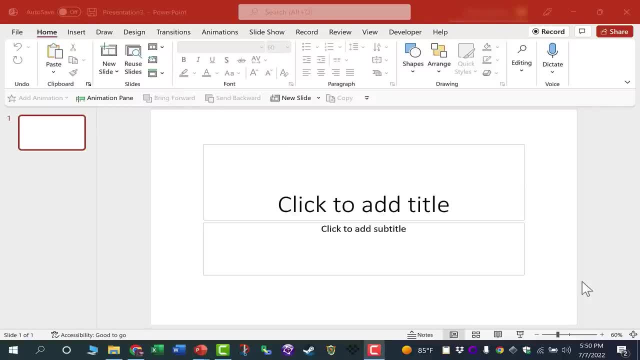 to open up a brand new blank PowerPoint presentation. And let's say that I'm a Spanish teacher and I want to create a presentation for my students about the country of Chile. I'll just click here where it says click to add title, and I'll type in Chile. 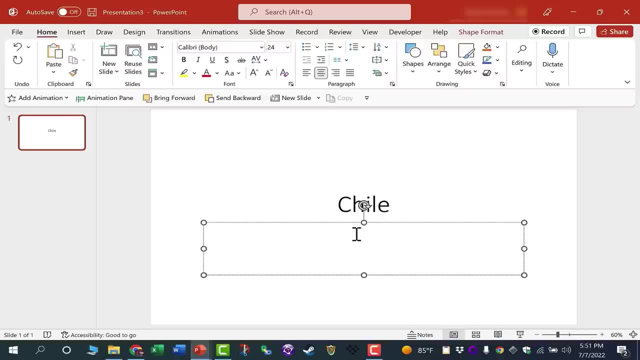 Underneath that I can click to add a subtitle. In many cases people will put their name here and type something like by so-and-so. In my case I just want to put a subtitle: Chile, country of poets. So now I have a simple title slide for my presentation. 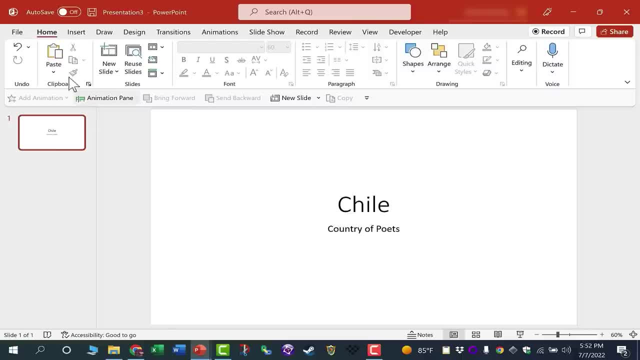 Now I'm ready to move on to my first content slide. If I go here to the home tab, here on the home ribbon in the slides group, I have a button that will give me a new slide. Now, if I click that, it does give me a new blank slide. 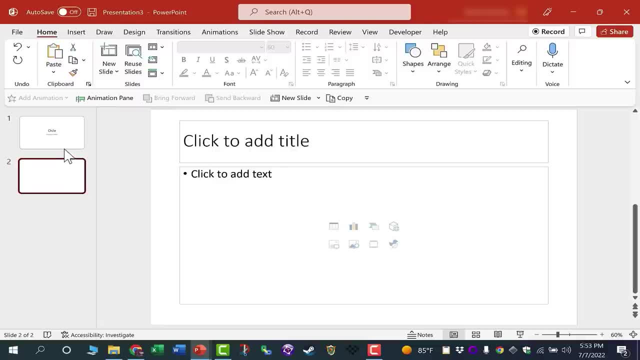 I can see the thumbnail for it here at the left. So now I have two thumbnails and two slides. If I want to go back and edit my first slide, I can click here on its thumbnail and then edit the slide here. For now I'll go back to my second slide. 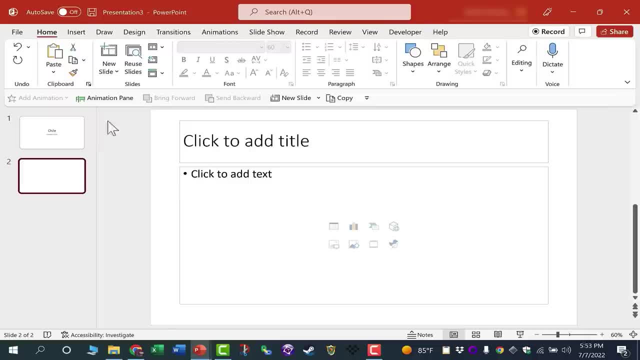 by clicking on my second thumbnail. Now, if you want to, you can specify the kind of new slide that you'll get. Instead of clicking here on the top half of this button, I could click on the bottom half, and it gives me a variety of options for this new slide. 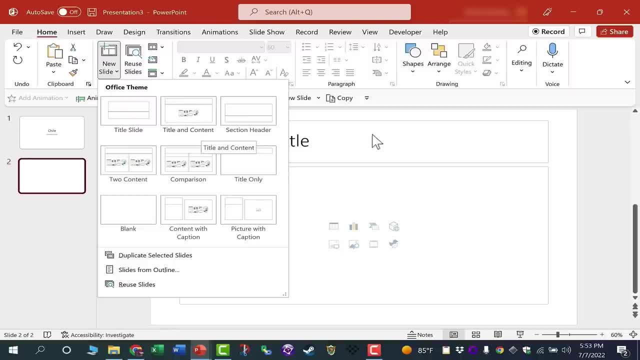 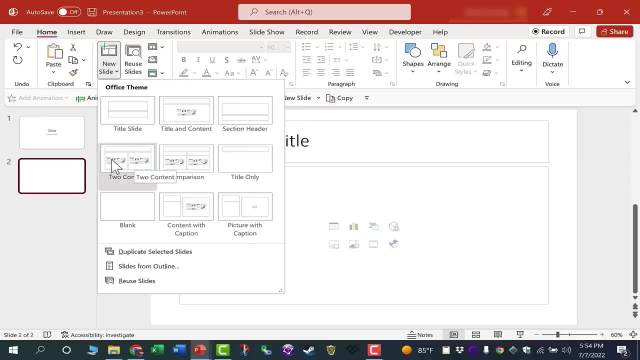 The default option is this: title and content. You can see it here: title and content. But if I prefer, I could just get a section, header or two items of content, one at the left, one at the right. I could get a new slide that is perfect for comparison. 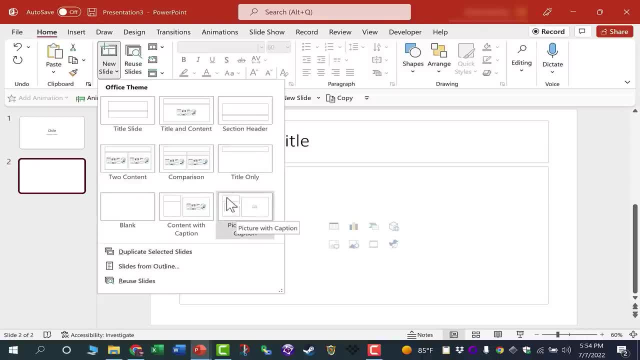 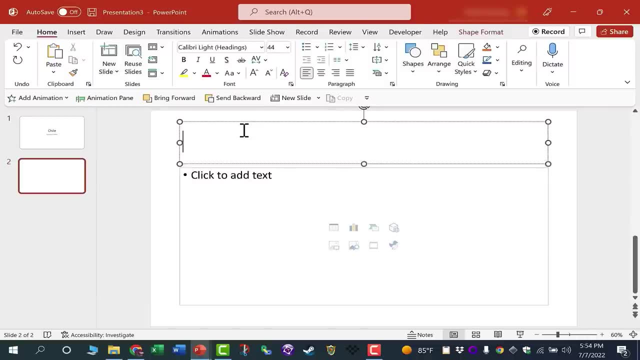 between the two, and you can see the other options here below. In my case, title and content is exactly what I wanted, so I'm happy. If I want to add a new slide, I'm going to click to add the title for this slide. 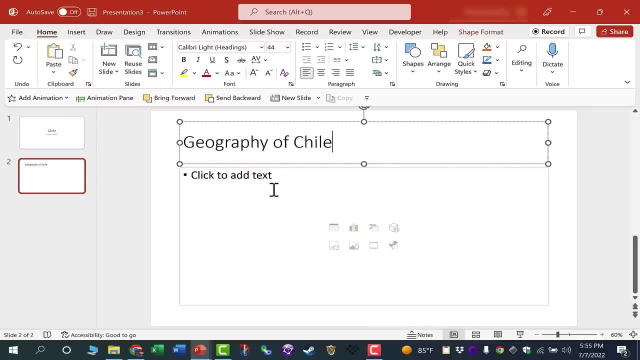 and I'll just type in geography of Chile. That's what this slide's gonna be about. Now, to add content to this slide, I can just click here. where it says click to add text, I can type in some information about the geography of Chile. 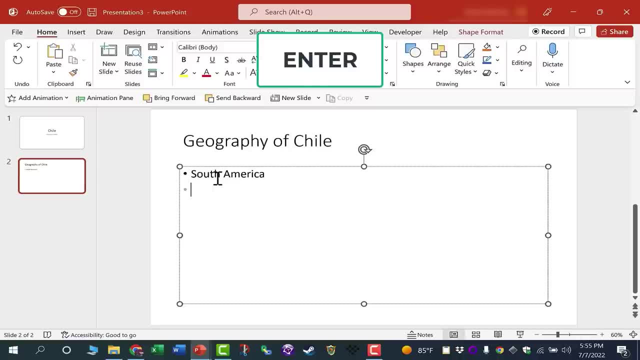 After typing in South America, I'll tap enter on the keyboard and I get a new bullet. If I want to, I can indent this bullet by tapping tab and I can continue typing and adding more information Now that I've done some work in my PowerPoint presentation. 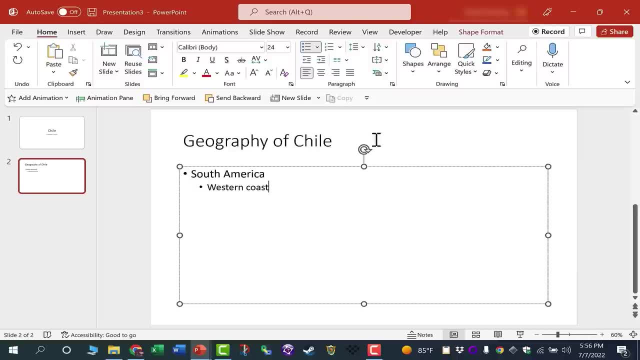 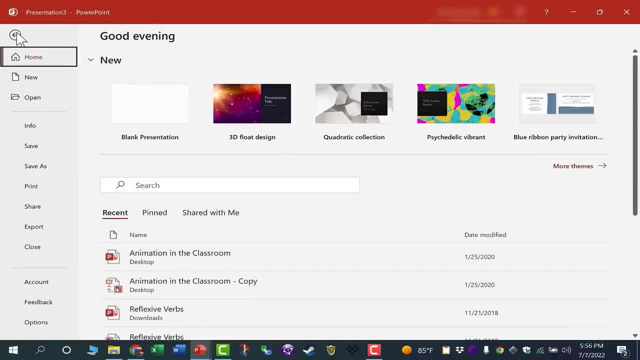 it's a good idea to go ahead and save this presentation. I could simply click this quick save button in the upper left, but I want you to see that there are other options. If I click here on file, it takes me to what's called the backstage view. 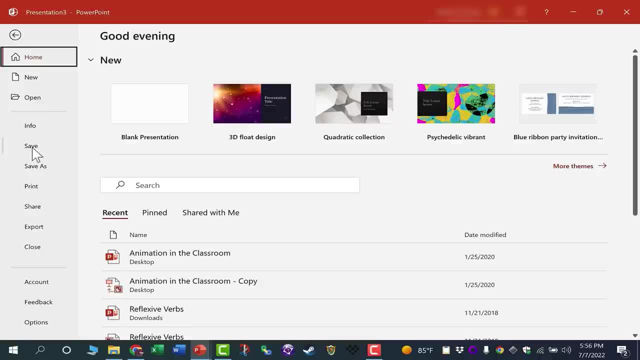 And here you can see that we have two main kinds of saves. We have just a regular save and we have a save, as In most cases when you save a presentation for the first time, it becomes a save, as Even if you click here on save. 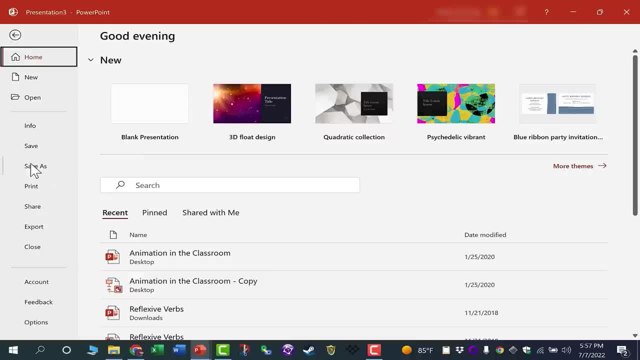 you can see that the presentation is saved. It will turn it into a save as. The reason why is because when you click save, as you're asked to provide a name for the PowerPoint presentation, You're also asked where to save it. So as long as you've done that once. 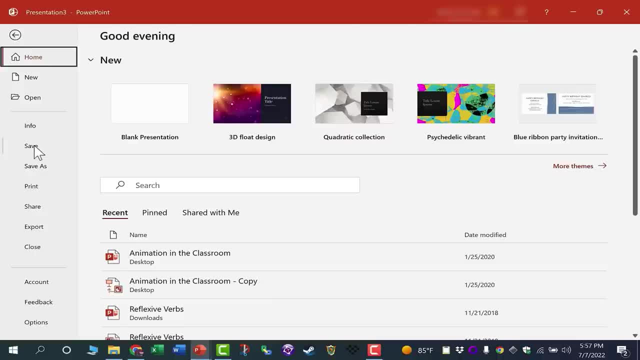 from then on, you can just click the regular save button and it will update the saved file. Now there are situations in which, even though you've saved as before and put in a name and a location for your presentation, there are situations in which you might want to save as again. 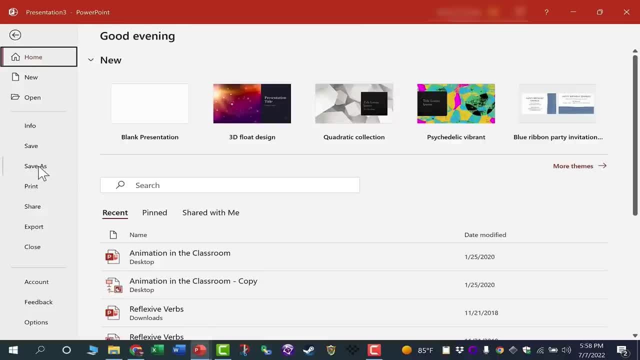 maybe to create a second version of a PowerPoint that you've made, So just try to be aware of the differences between the two. To demonstrate this, I'm going to click the regular save, but watch as it converts it into a save, as because I need to provide a name and a location. 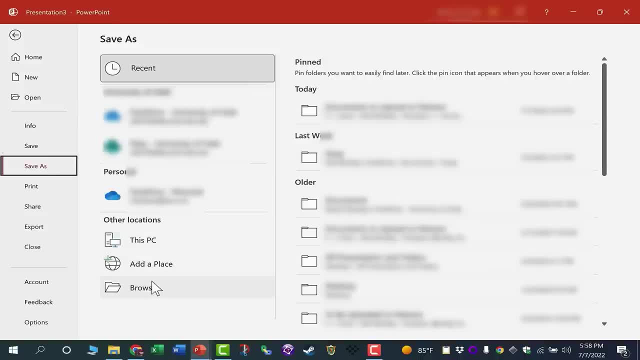 So it's become a save as and now I need to determine where am I going to save this presentation. In most cases, you'll probably want to save it to your computer and you'll probably need to browse, So I clicked on browse. It opens up this dialog box and I can see that it's saved as, So I'm going to click save as, and I can see that it's saved as, So I clicked on browse. it opens up this dialog box and I can see that it's saved as. So I clicked on browse. it opens up this dialog box and I can see that it's saved as. So I clicked on browse. it opens up this dialog box and I can see that it's saved as, And I can specify where on my computer. 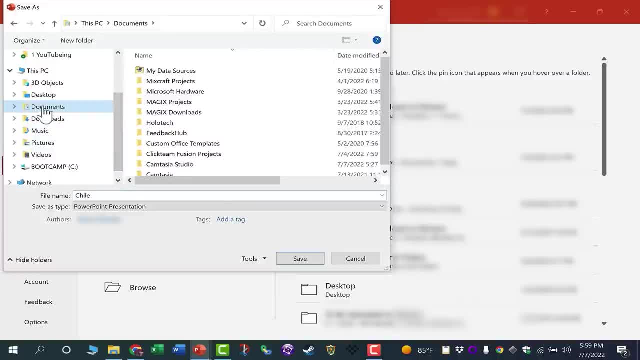 I'd like to save this presentation. In this case I think I'll save it in my documents. Notice that it put in Chile as the file name. PowerPoint pulled that from the title that I typed onto the title slide, So that's perfectly fine. 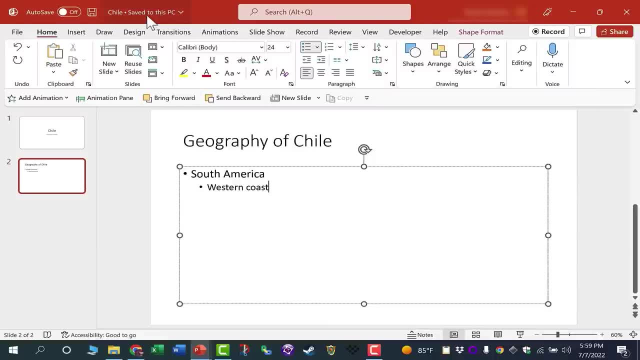 I'll go ahead and click save And now you can see up here on the title bar I now have a title for my presentation. So in this first segment of PowerPoint for Beginners Complete Course, we've looked at the layout in Microsoft PowerPoint. We've also looked at how to create a new blank presentation. 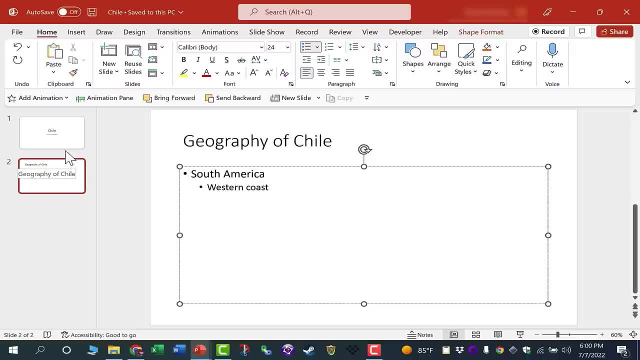 how to make some basic edits, how to add a new slide and also how to save your presentation. In this next segment of PowerPoint for Beginners Complete Course, we're going to look at how to open and edit an existing presentation, So I'm going to leave this presentation that I'm working. 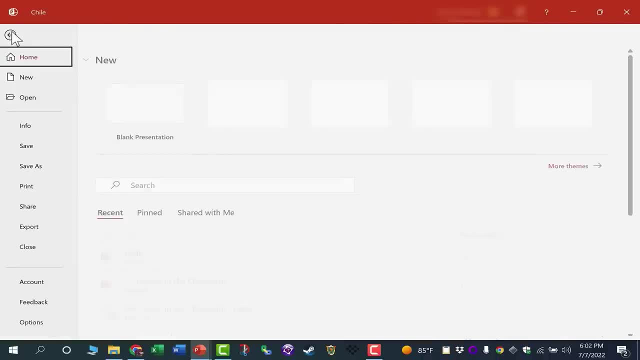 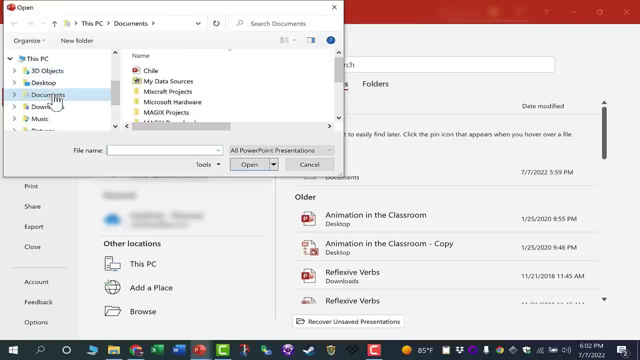 on open, but I'm also going to go here to the upper left corner. click on File and Open, and I'll click here on Browse. By default it took me to my Documents, but if it hadn't done so, I could. 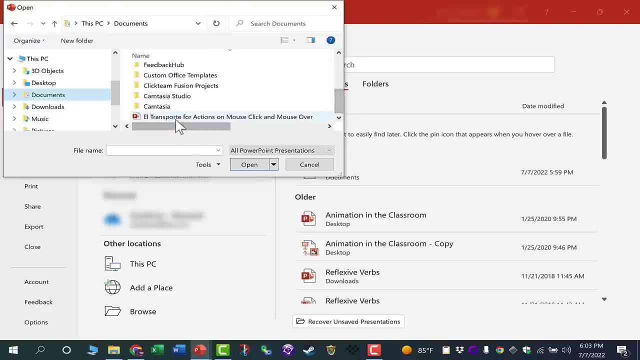 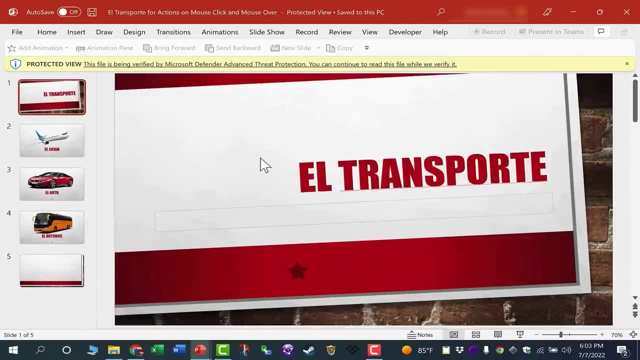 have clicked on Documents, and then I can browse through this list to find the presentation that I'm looking for. There it is, and I'll click on it and click Open. and now I'll have a second PowerPoint presentation opened up, And I want to just click this button Enable Editing. and now, 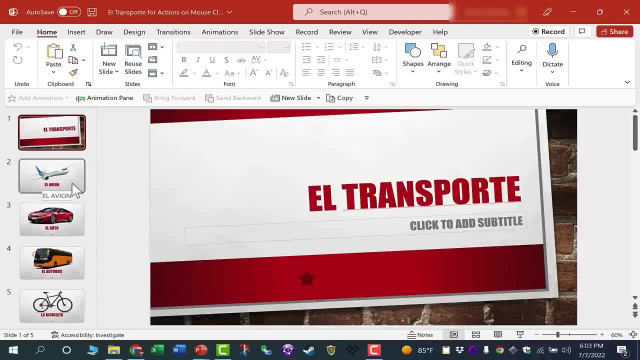 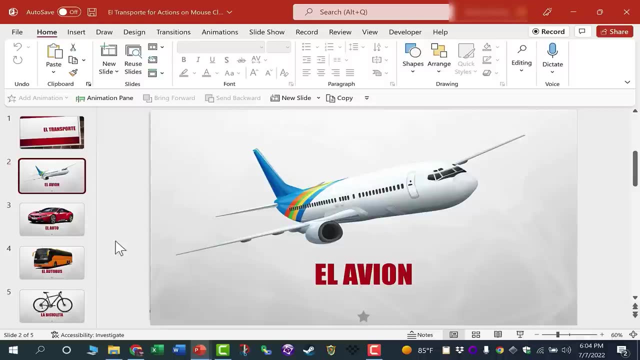 I have this pre-existing PowerPoint presentation opened up and ready to be used. As I hinted at in the previous segment, the way you navigate through a presentation is pretty straightforward. You simply click on the thumbnail of the slide that you would like to look at, and it's displayed here in the center of the 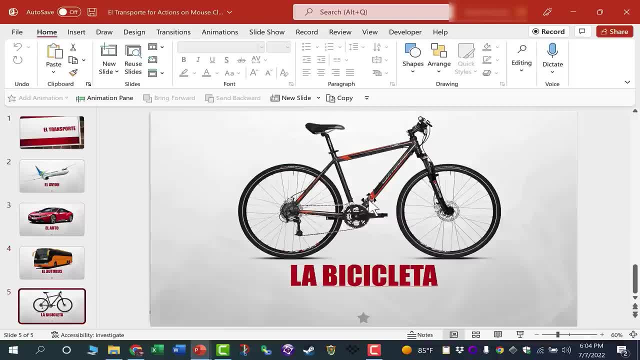 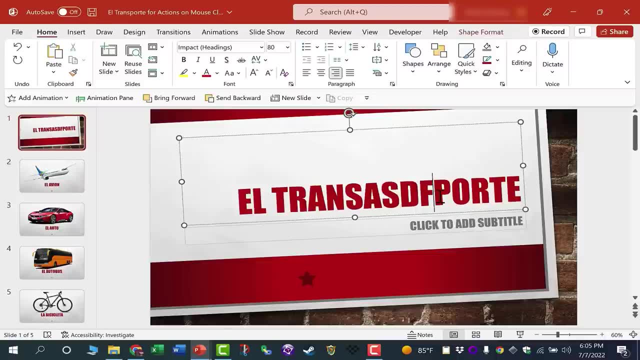 screen, So I can click here, click here, click here and the active slide is updated. Of course, I can edit any of this information, including the text. I can just click to add characters or to delete. I can triple click to select the entire paragraph or phrase, in this case, and then I could type over. 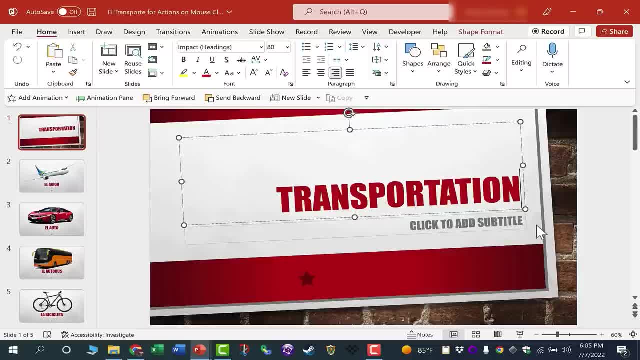 that, if I want to, And then any time I make a change, I can just click away and that change is recorded. I'm going to undo that holding Control and tapping Z. You can also undo here in the upper left corner using this button. 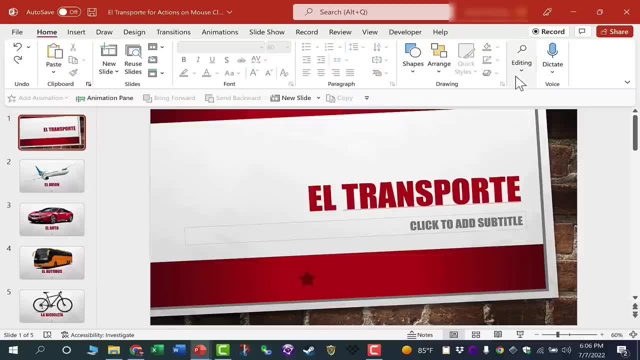 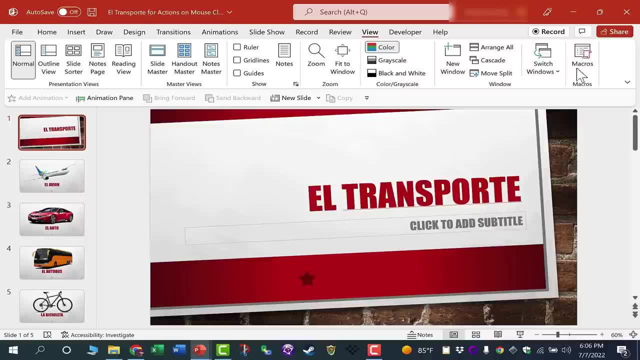 Now, as you work in Microsoft PowerPoint, you may need to switch the view of your presentation. So let's look up here on the View tab. When I click that, we get the View ribbon and you can see there are several different presentation views. I've already talked about some of these when I showed you these buttons here at the bottom. 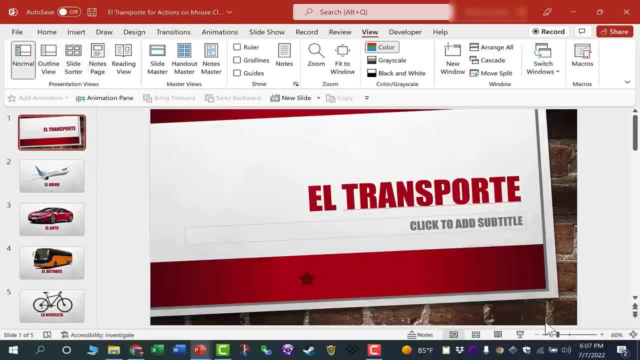 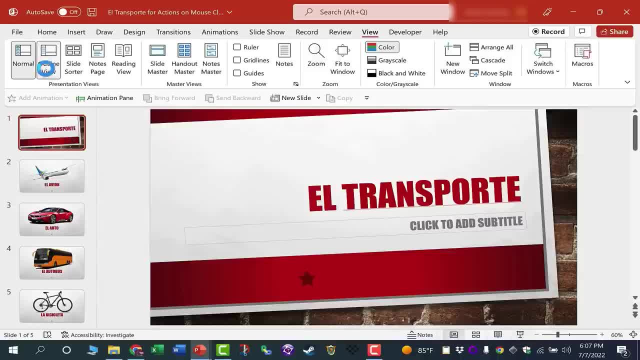 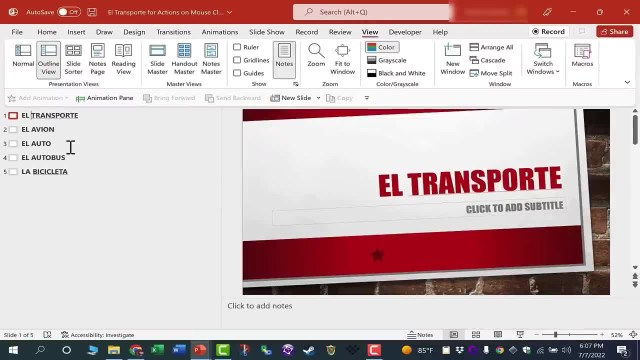 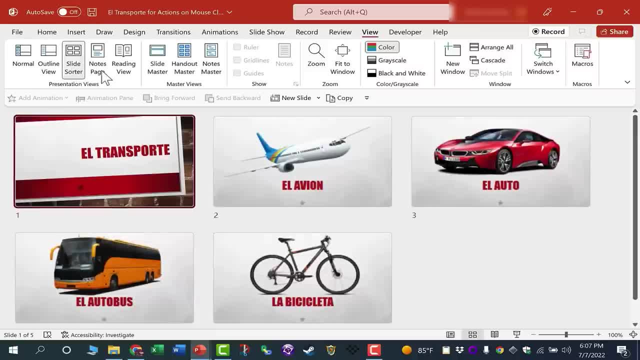 I do want to point out this view, the outline view. When you click on that, it gives you an outline overview of your presentation. Like I showed earlier, we also have the slide sorter. This makes it really easy and handy to click and drag and reorder your slides. 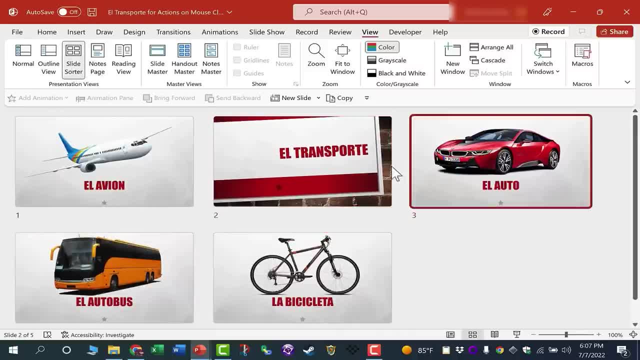 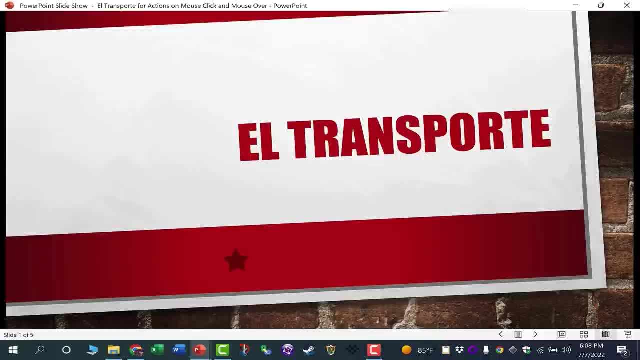 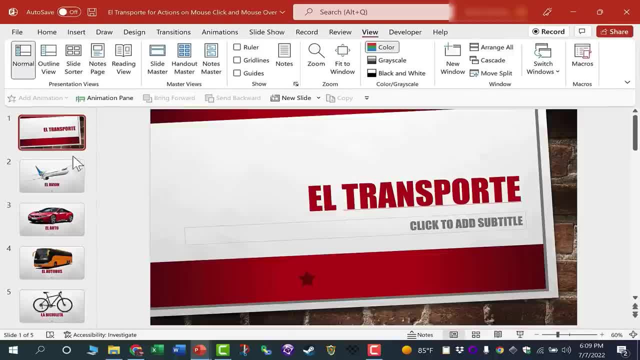 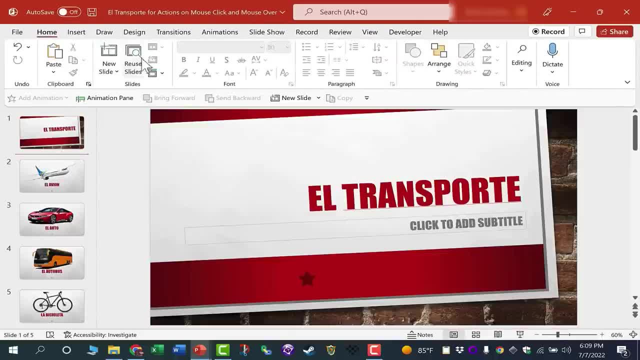 Like I showed earlier, we also have the slide sorter. This makes it really easy and handy to click and drag and reorder your slides. Like I showed earlier, we also have the slide sorter. This makes it really easy and handy to click and reorder your slides. 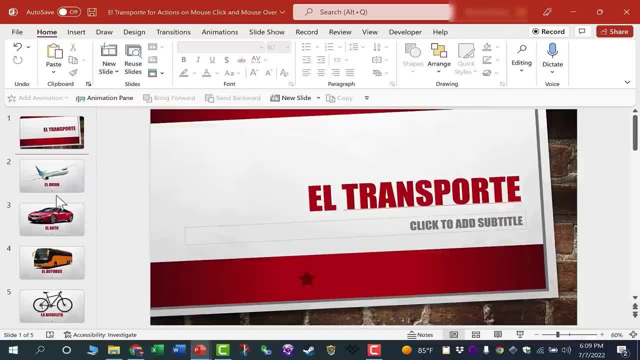 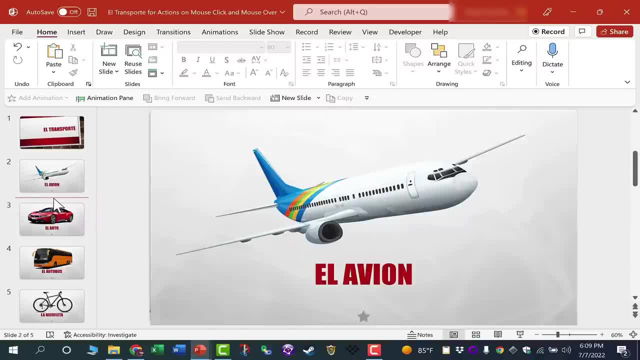 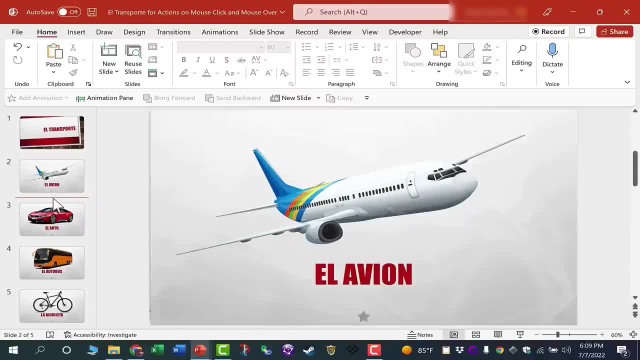 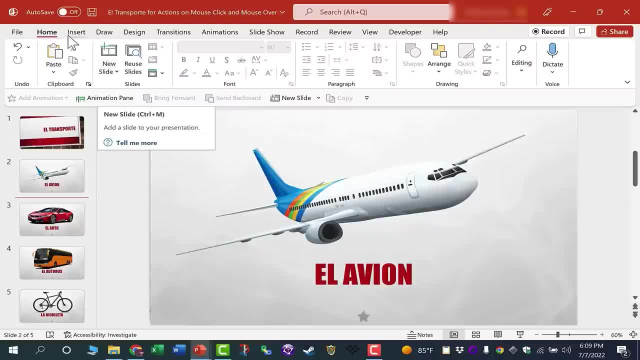 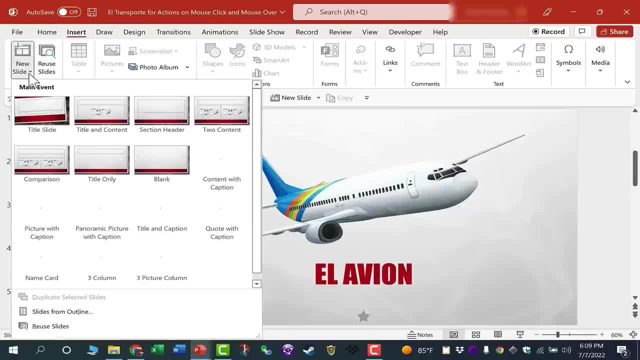 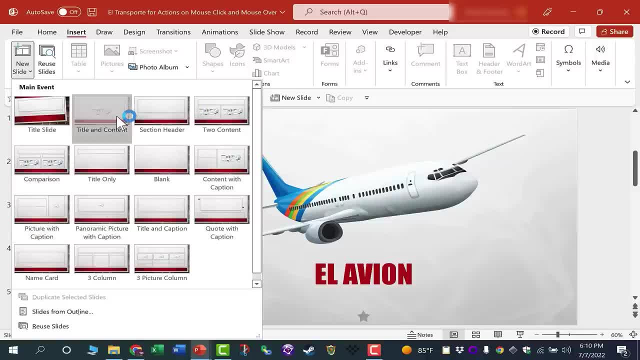 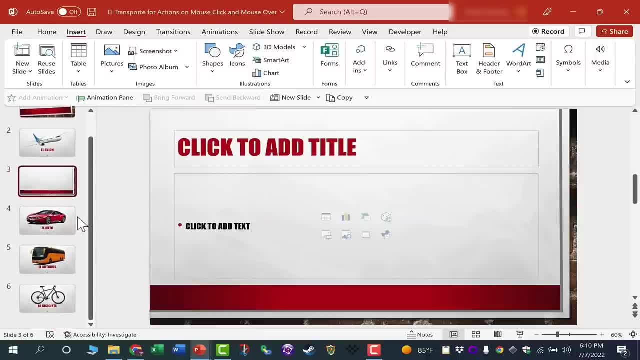 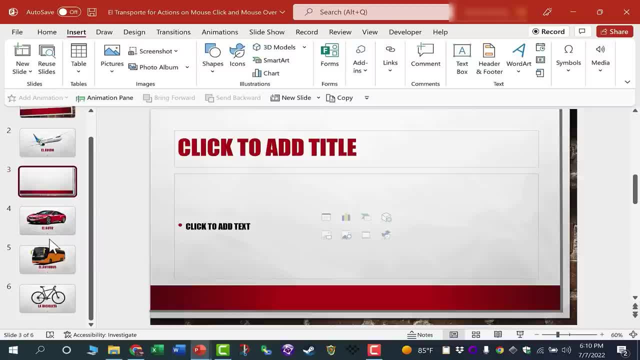 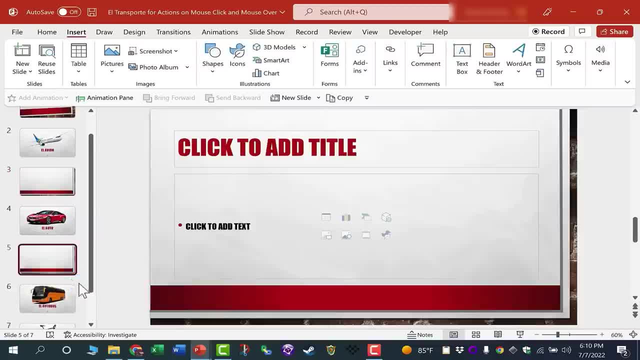 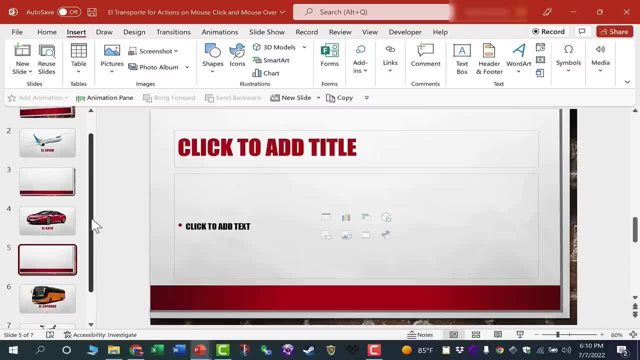 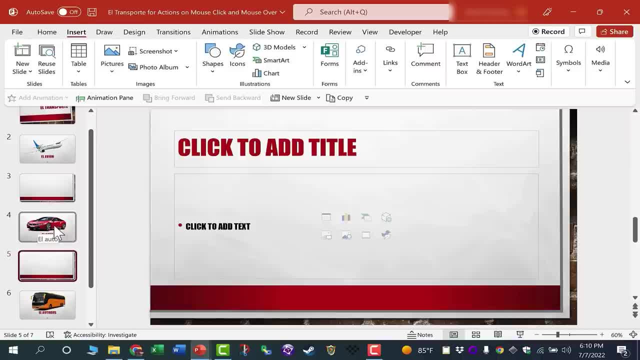 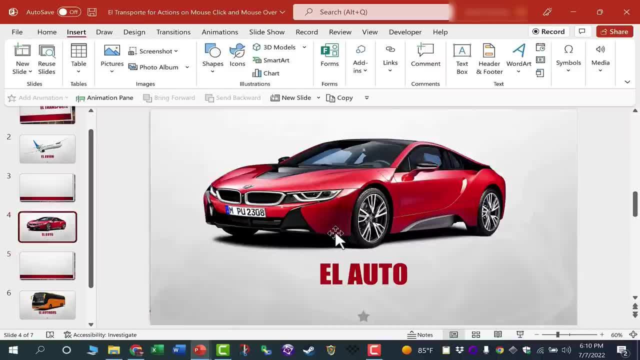 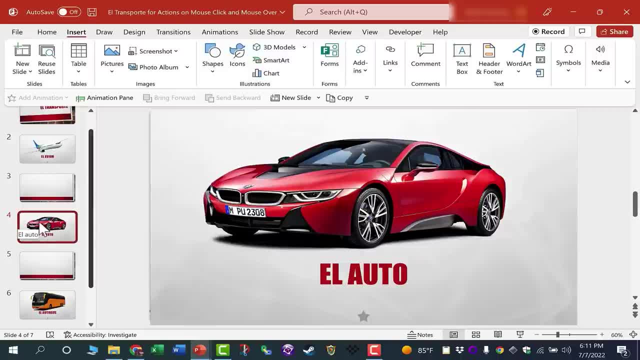 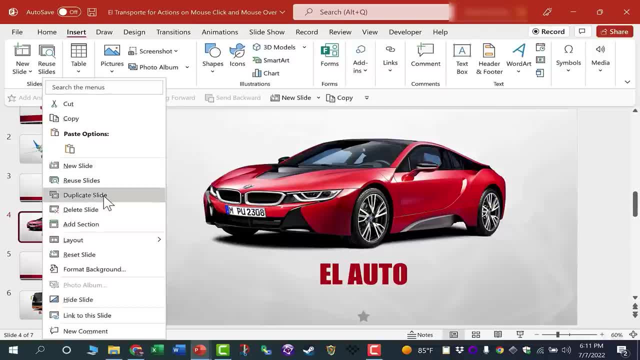 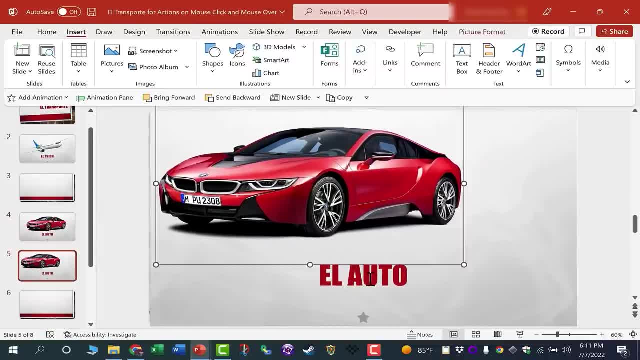 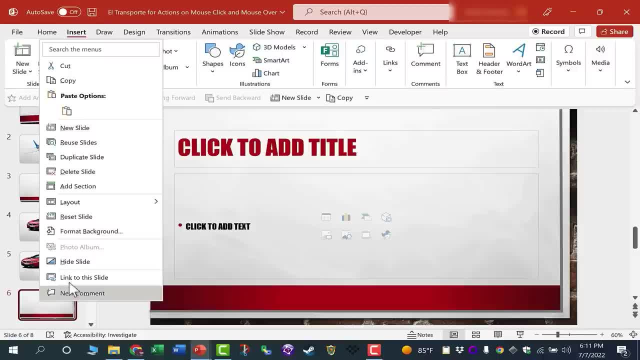 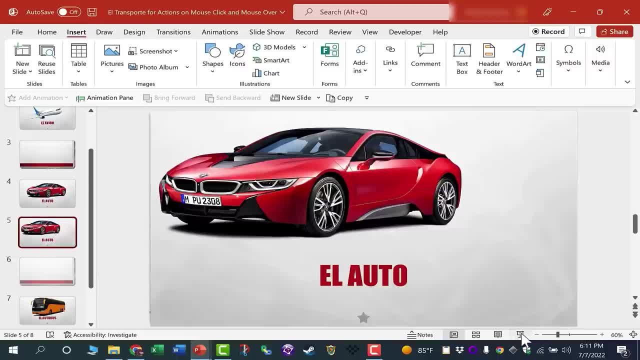 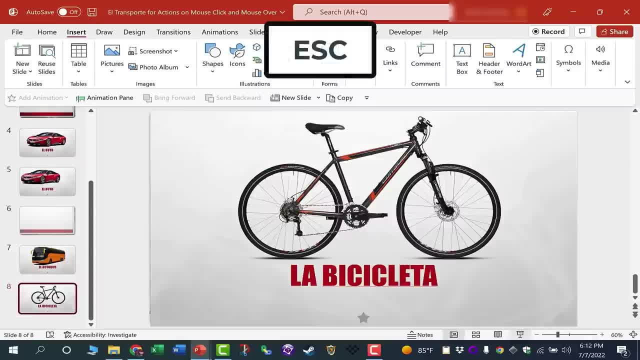 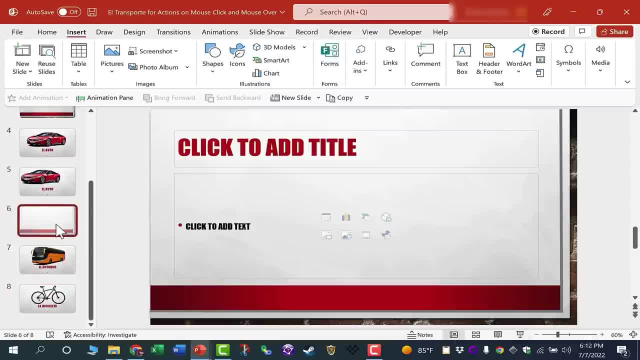 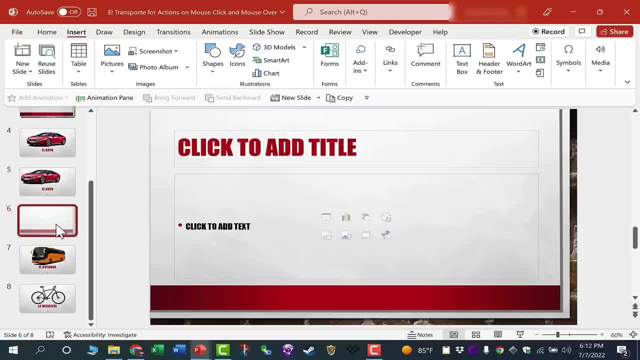 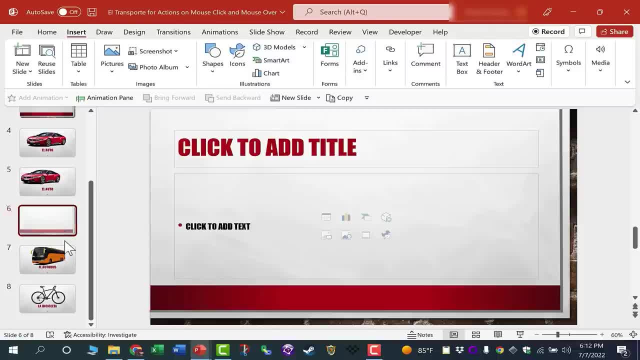 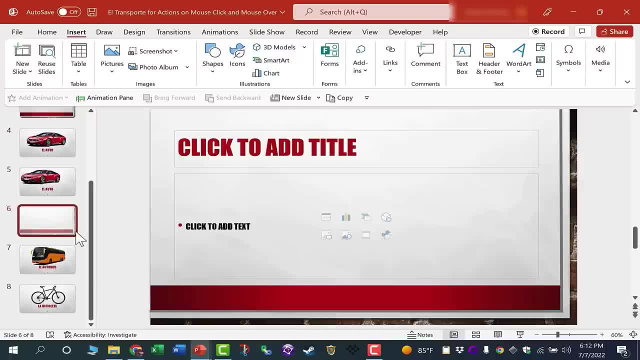 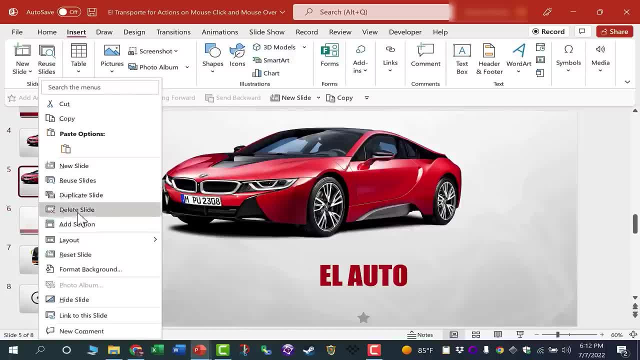 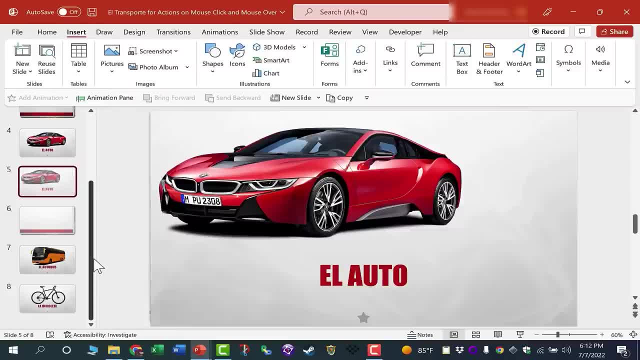 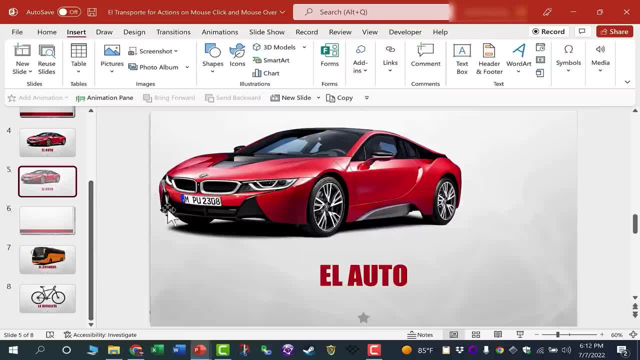 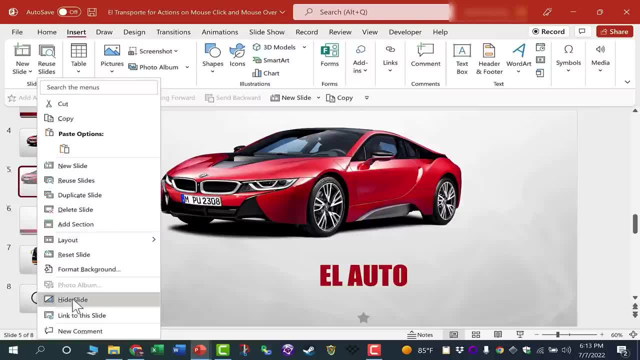 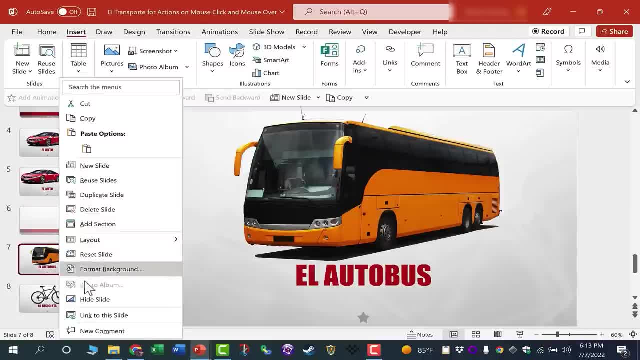 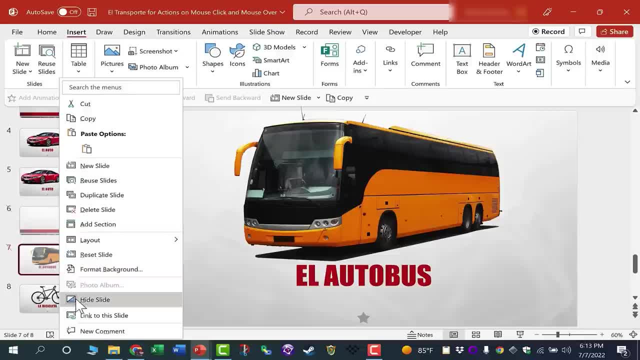 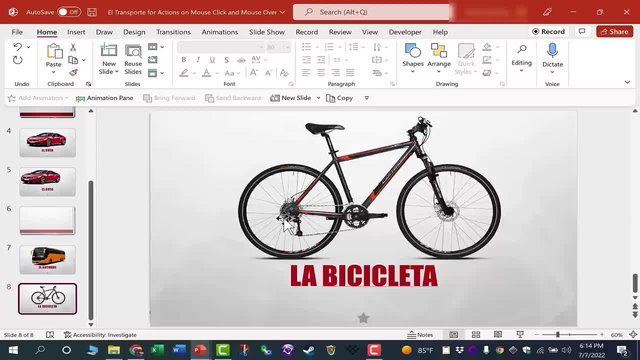 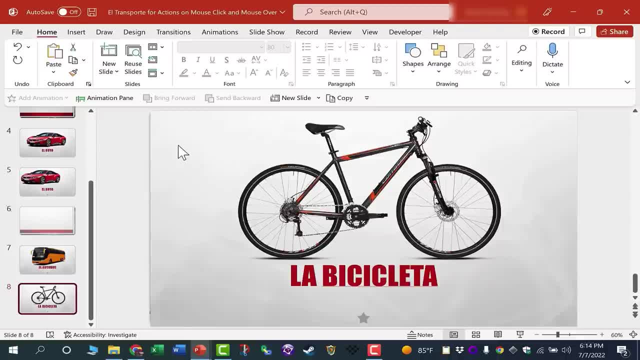 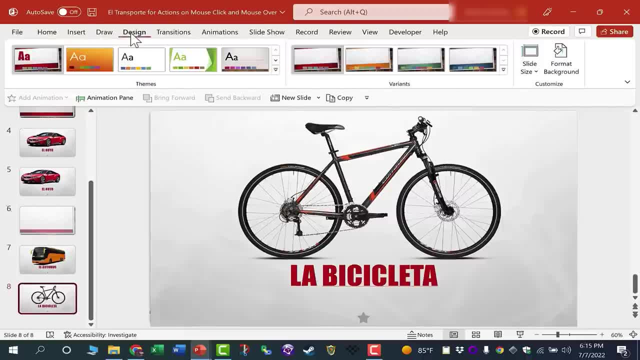 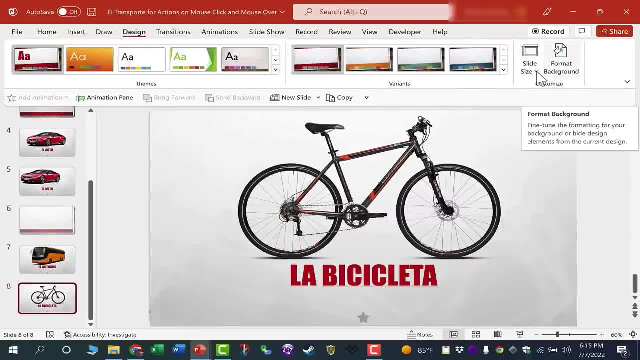 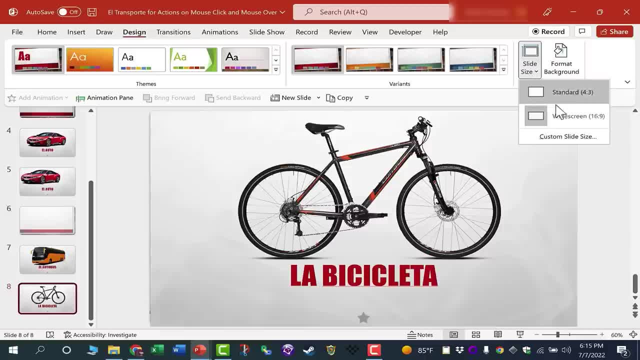 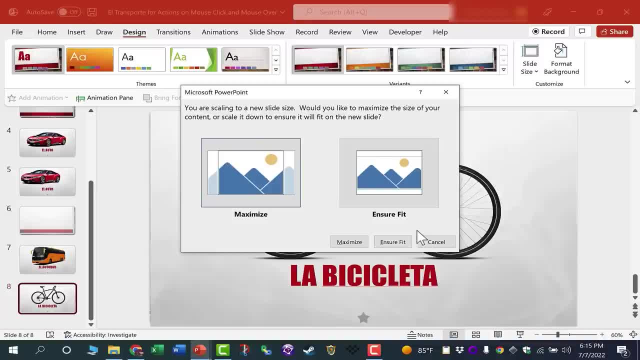 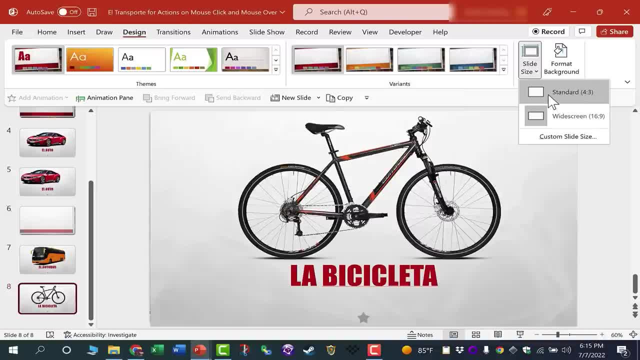 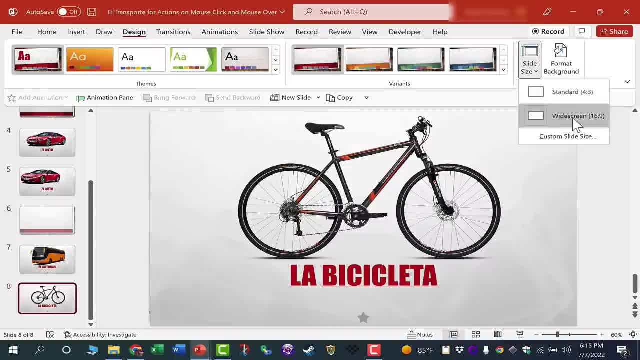 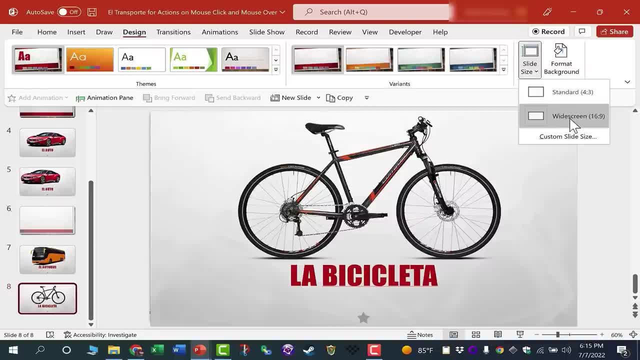 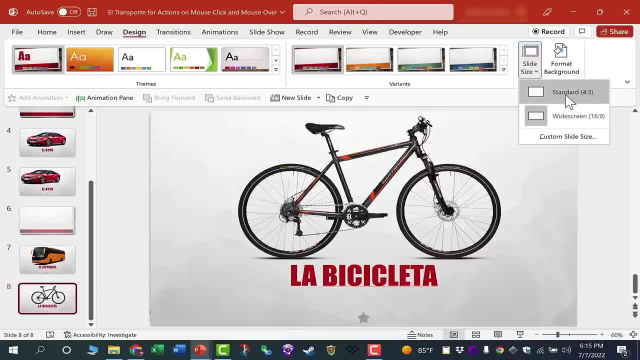 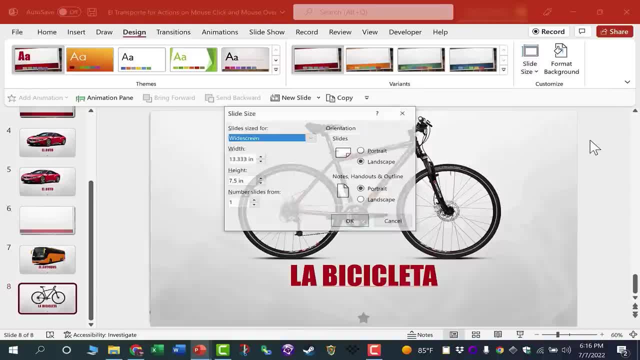 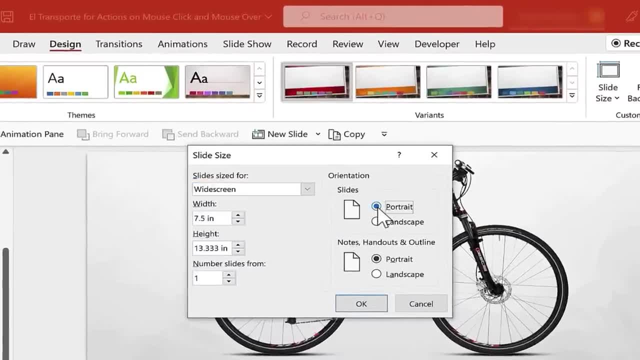 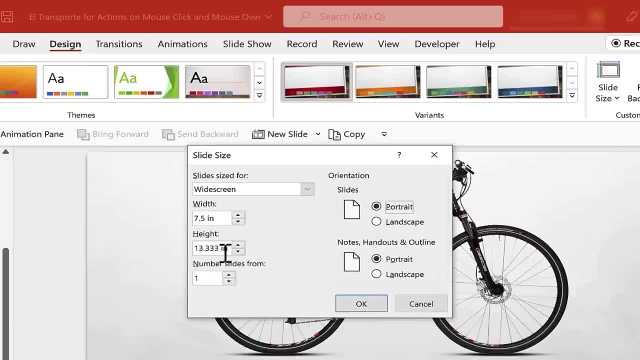 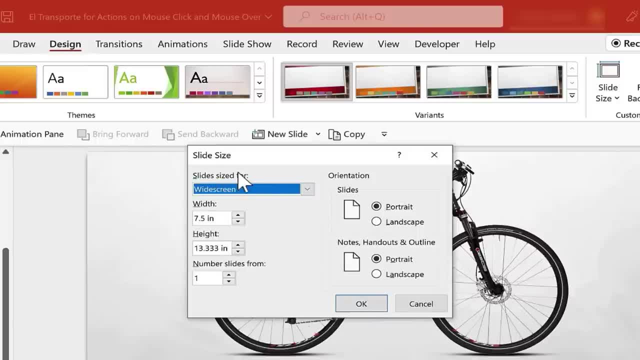 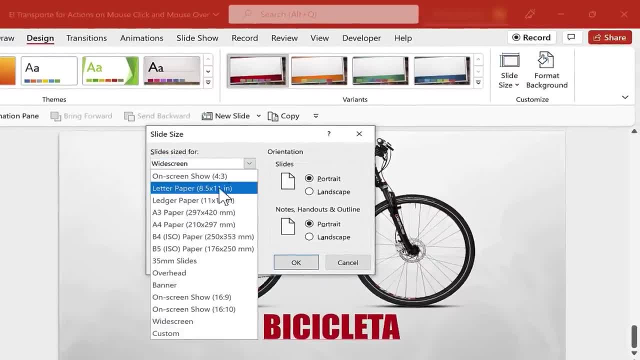 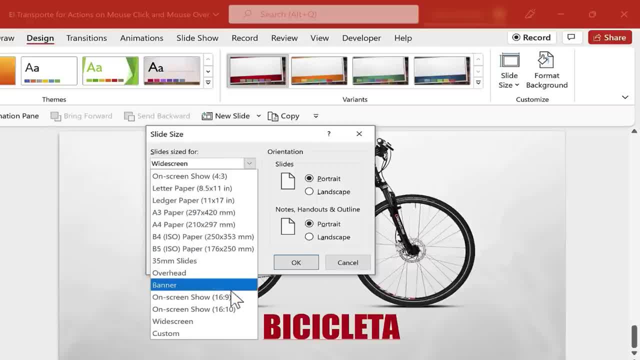 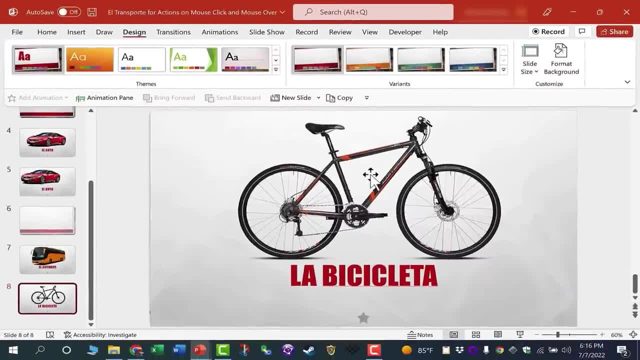 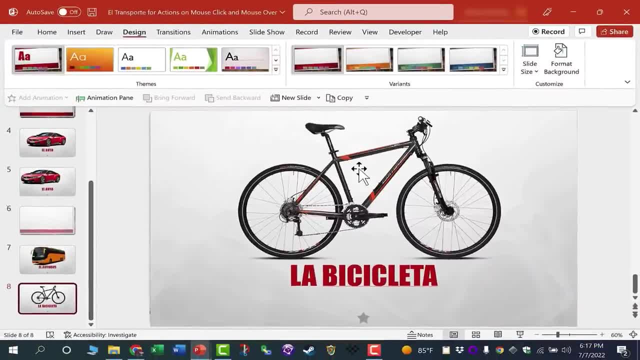 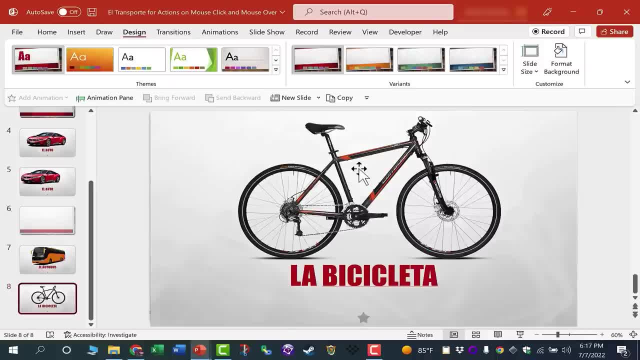 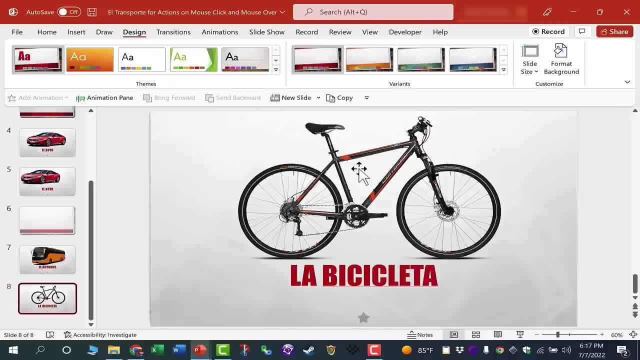 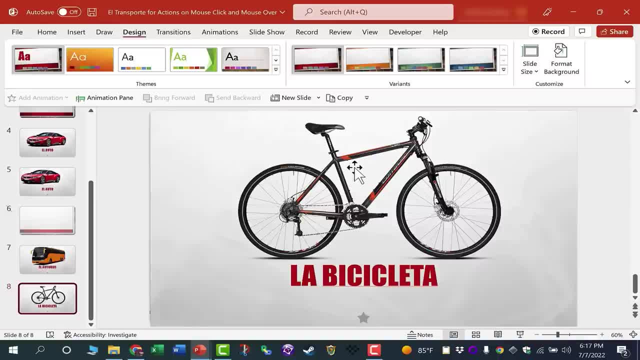 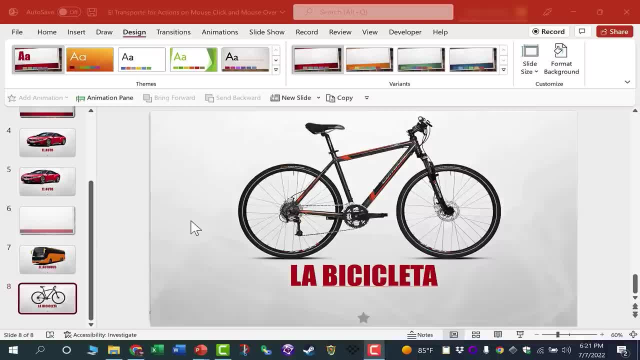 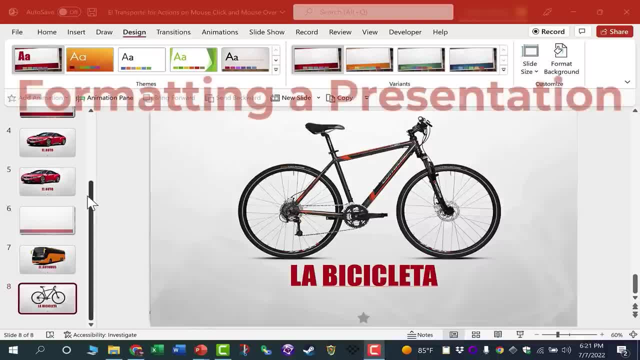 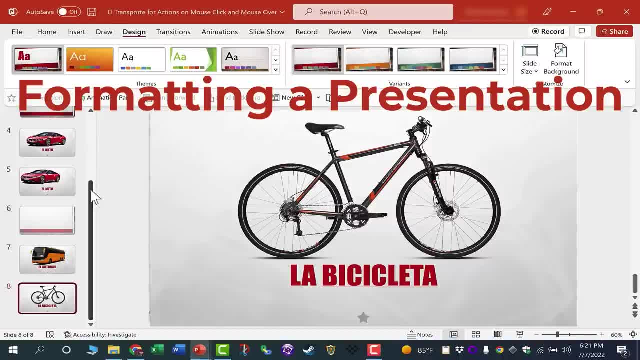 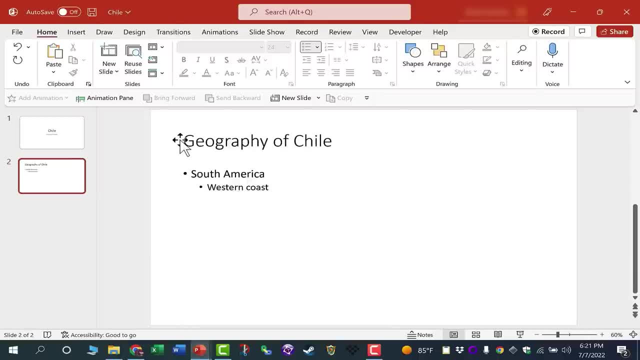 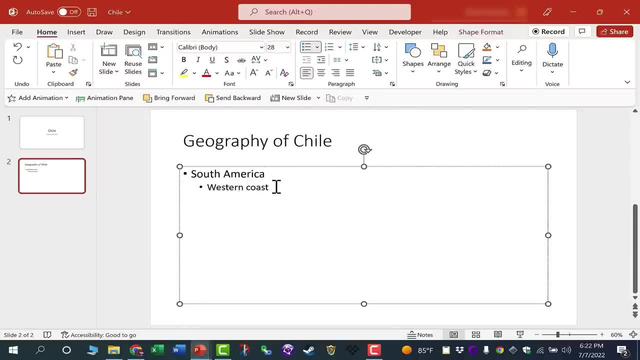 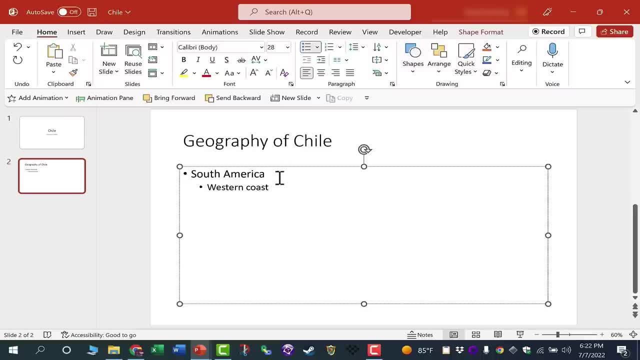 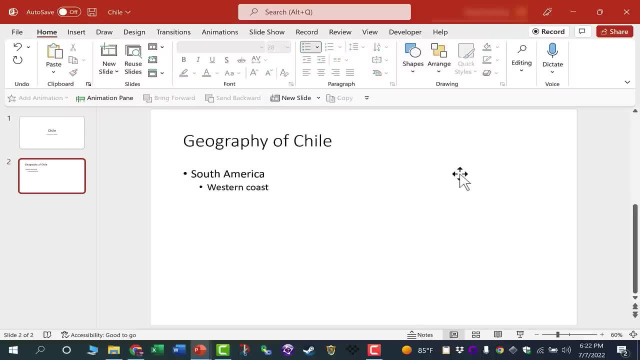 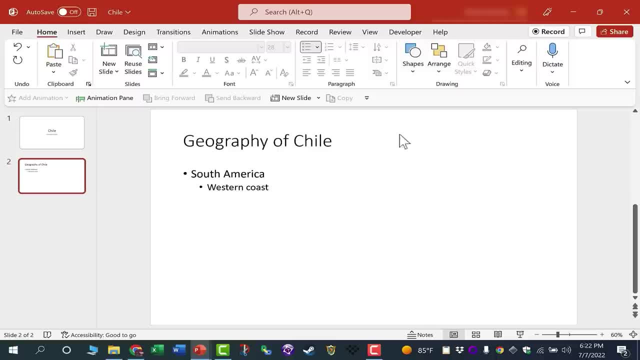 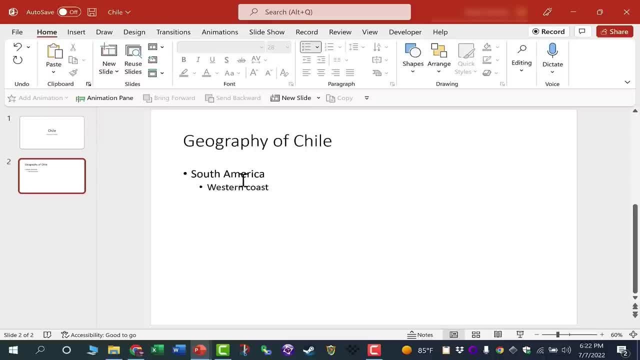 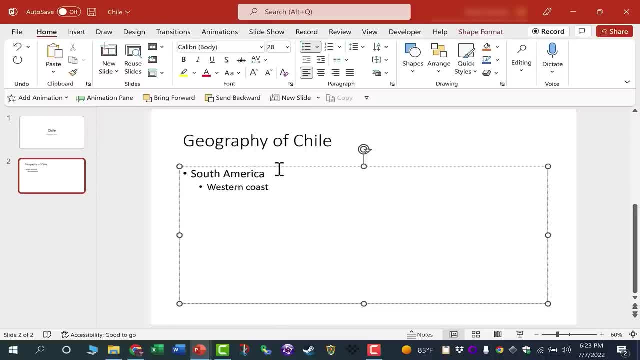 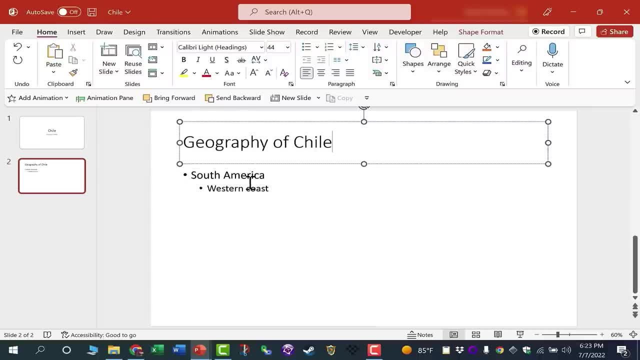 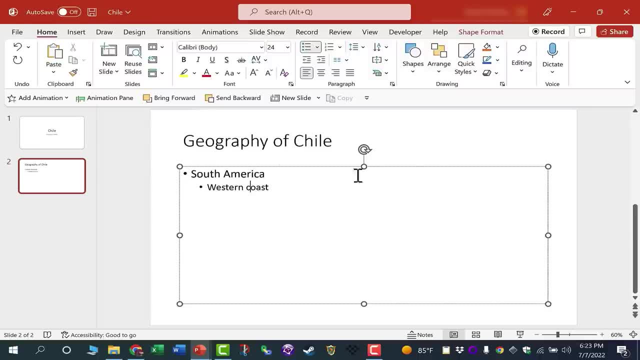 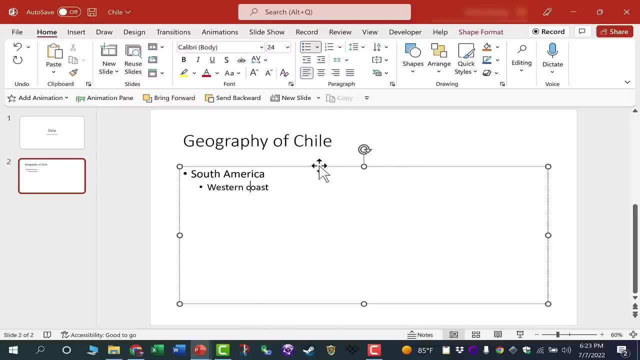 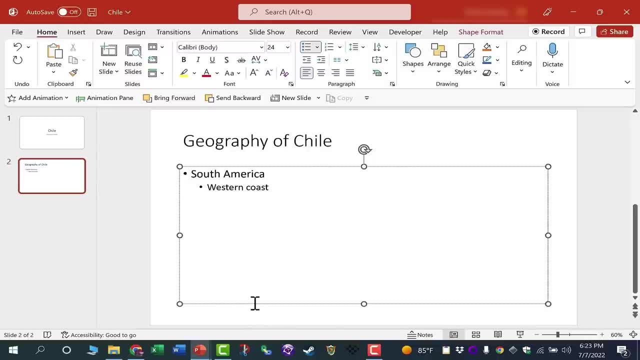 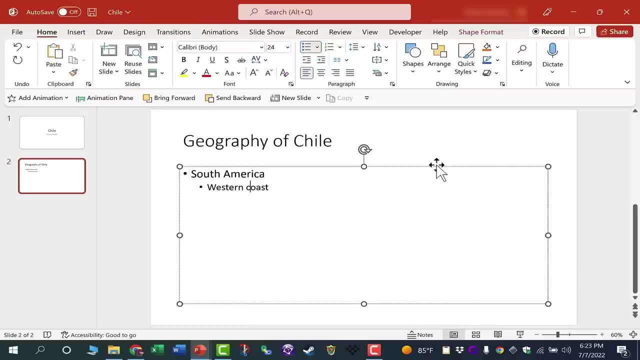 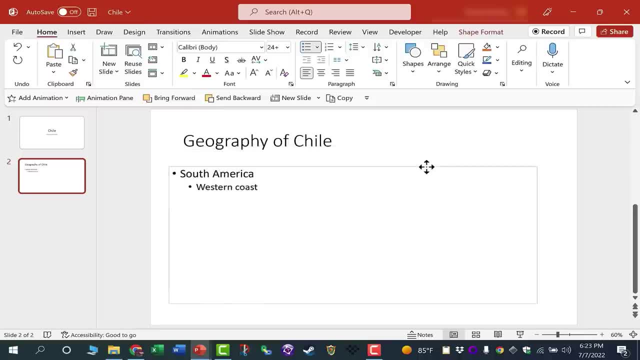 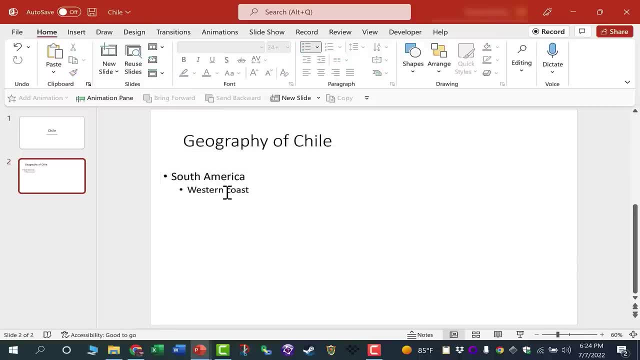 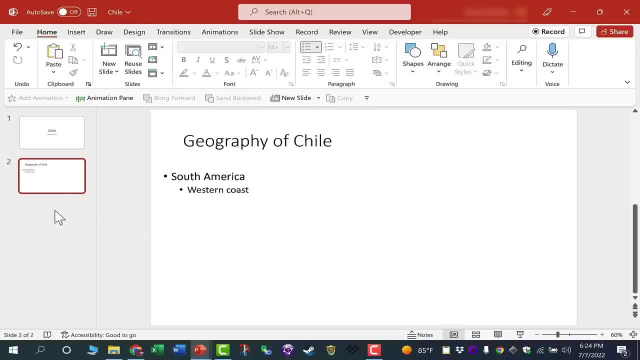 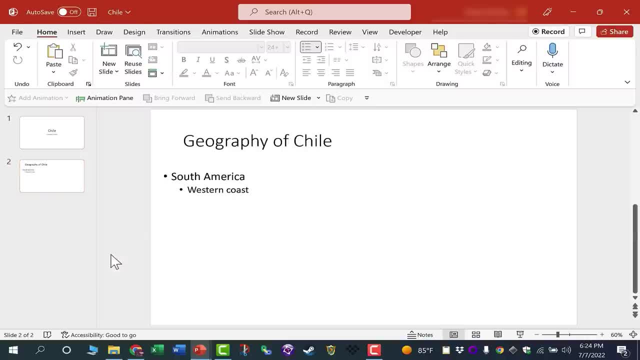 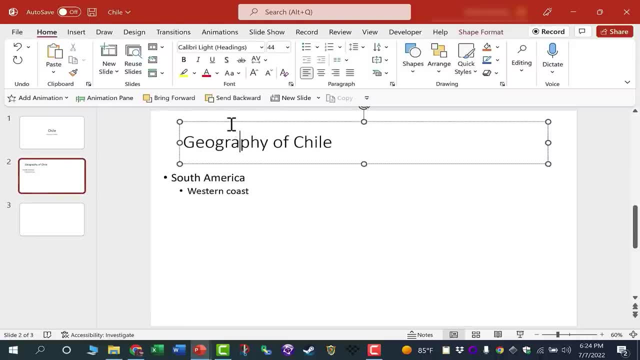 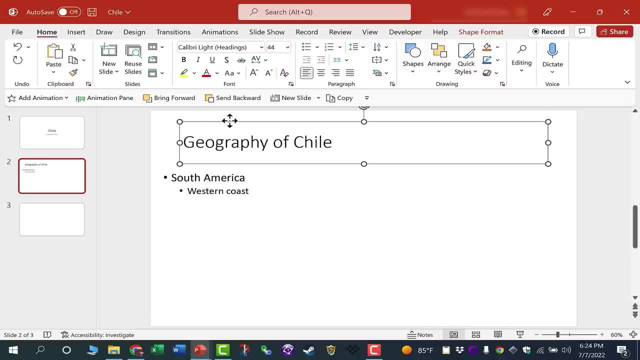 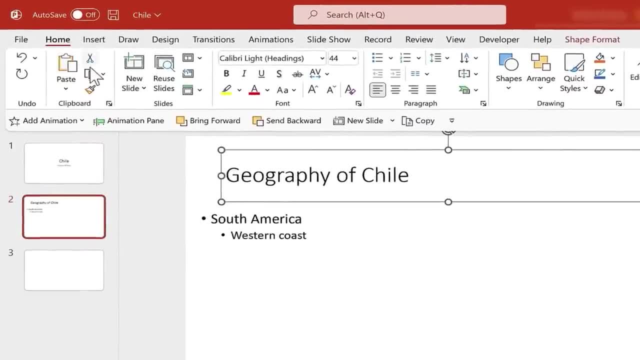 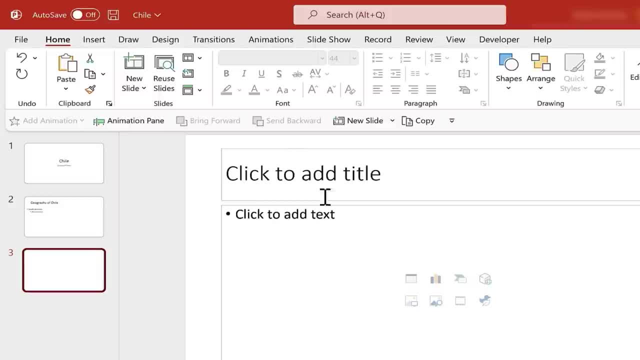 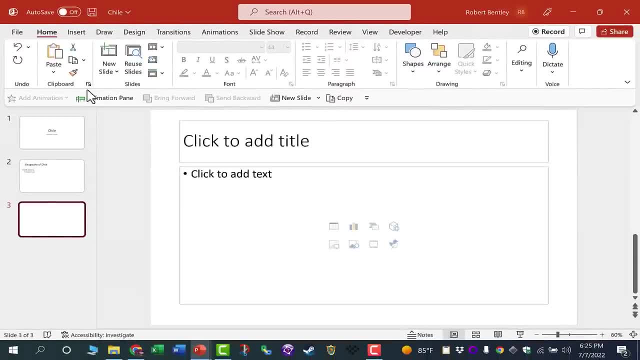 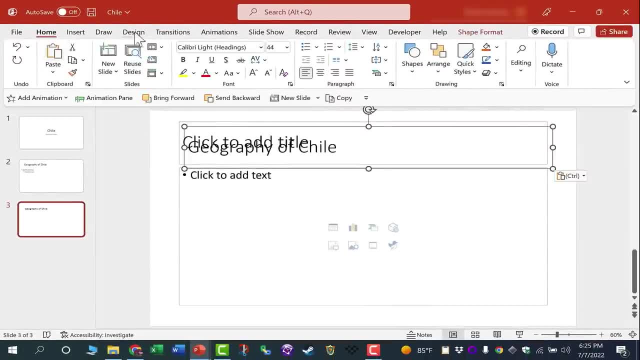 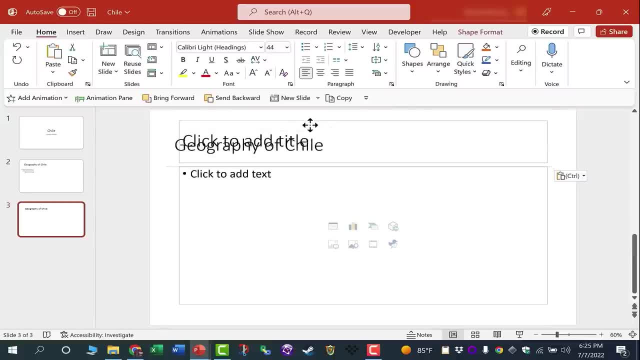 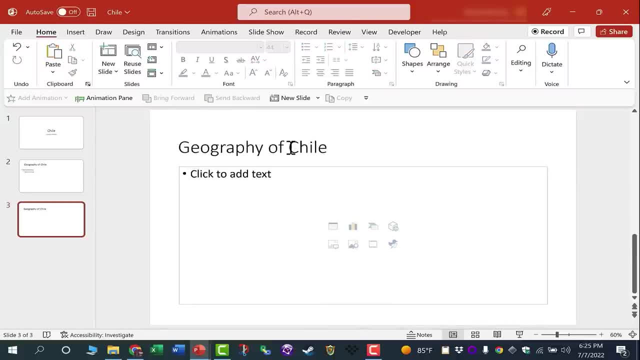 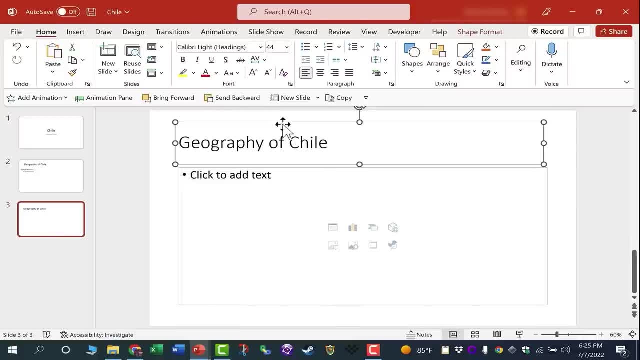 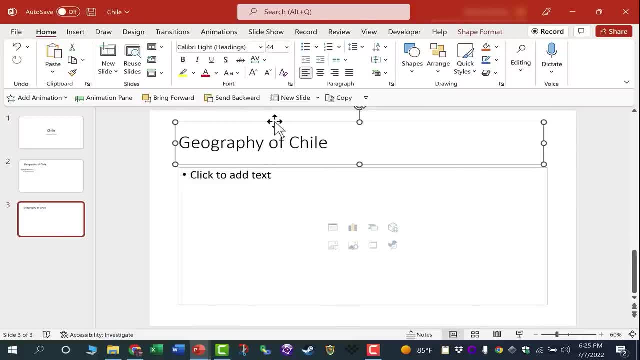 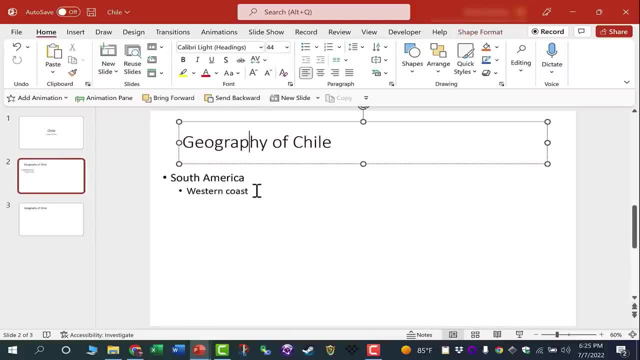 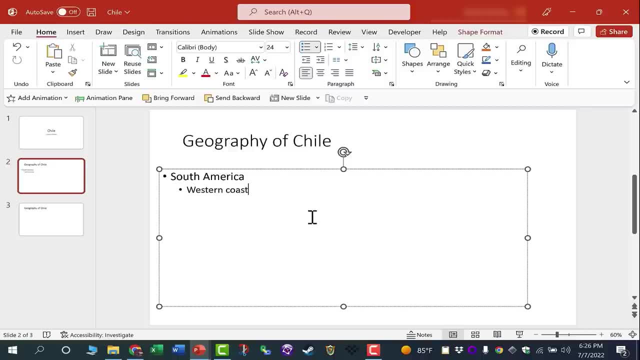 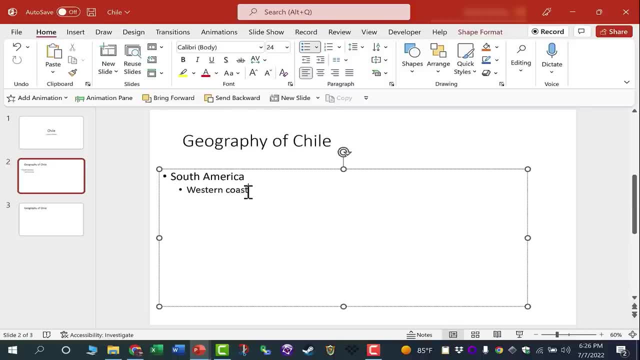 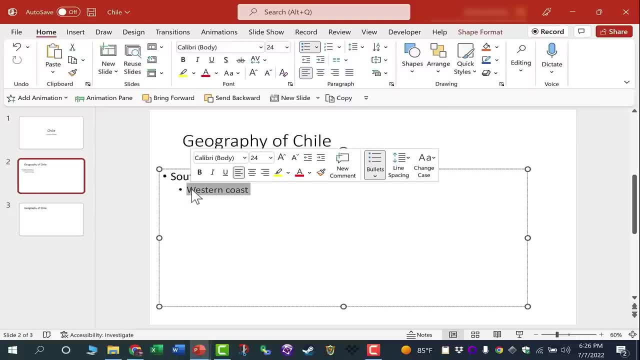 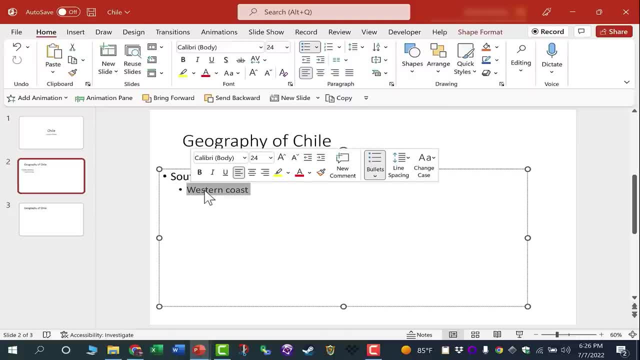 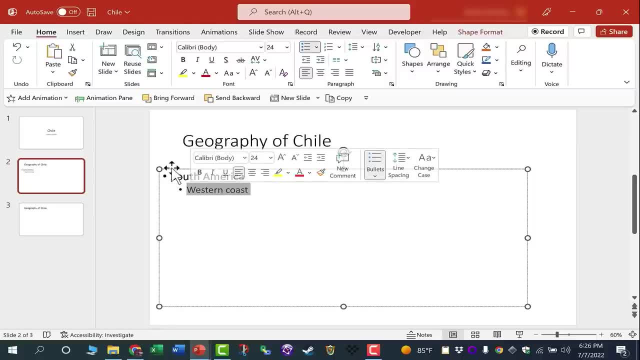 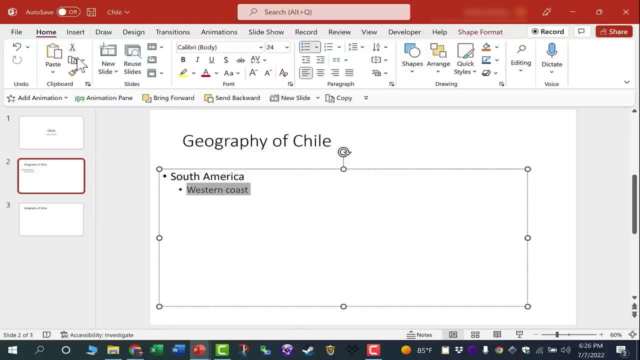 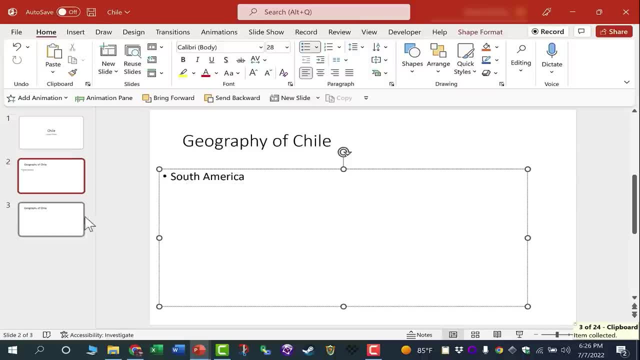 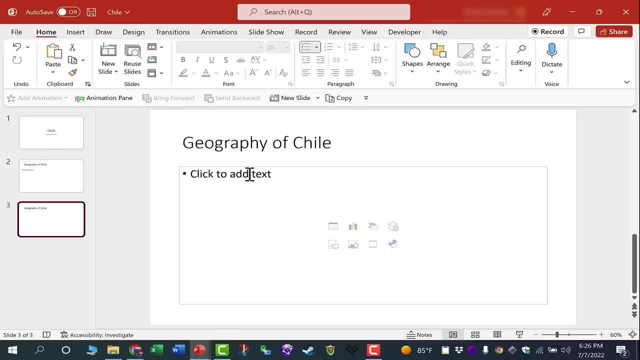 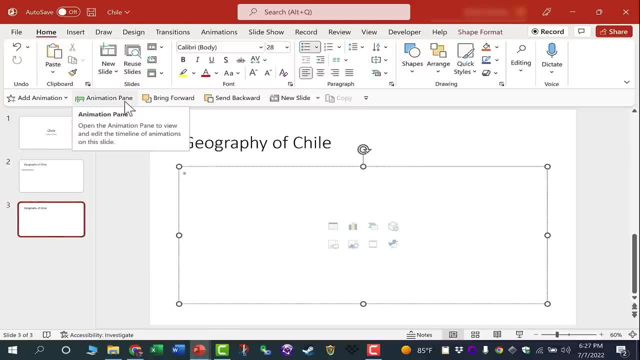 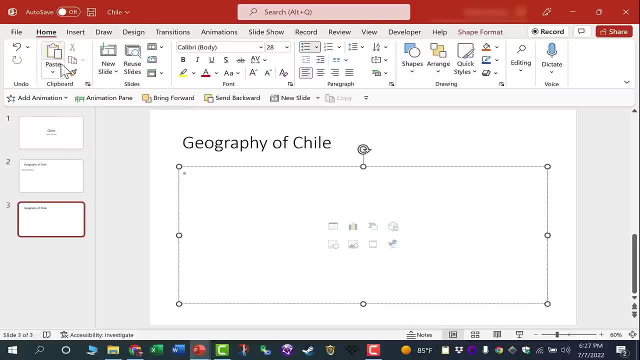 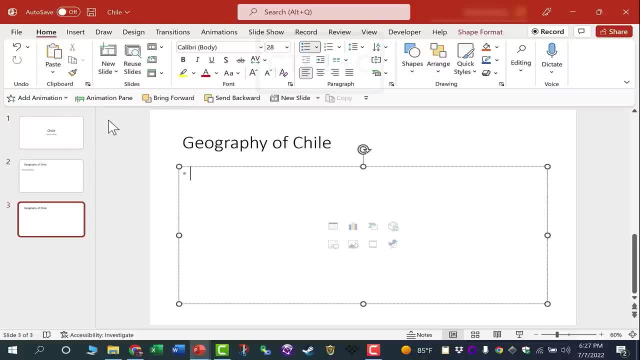 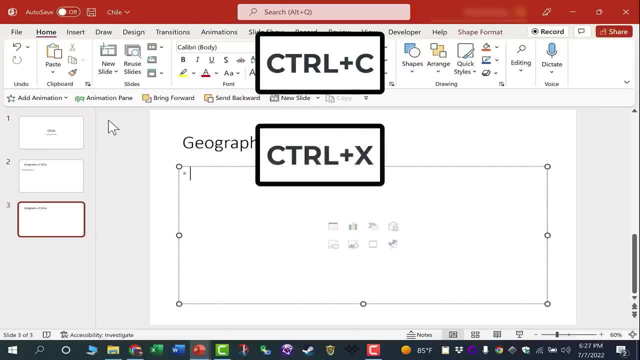 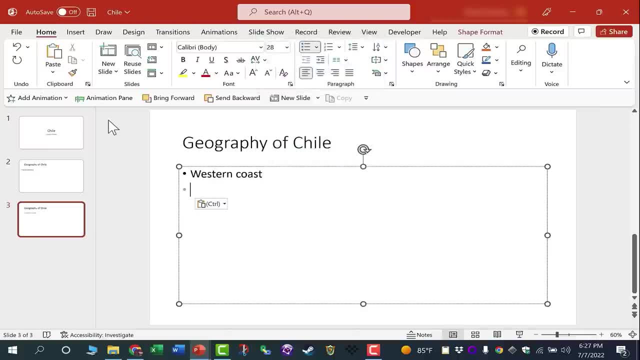 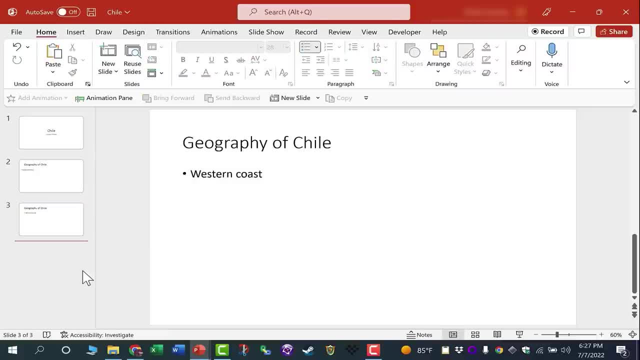 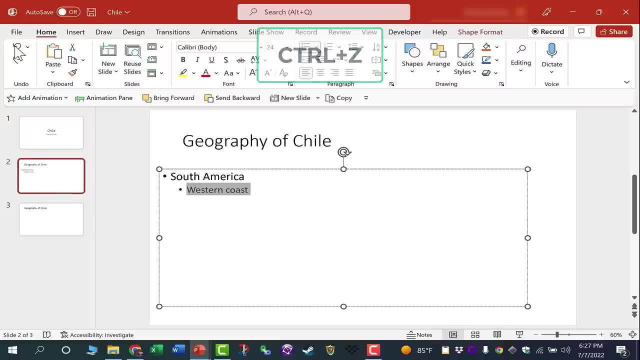 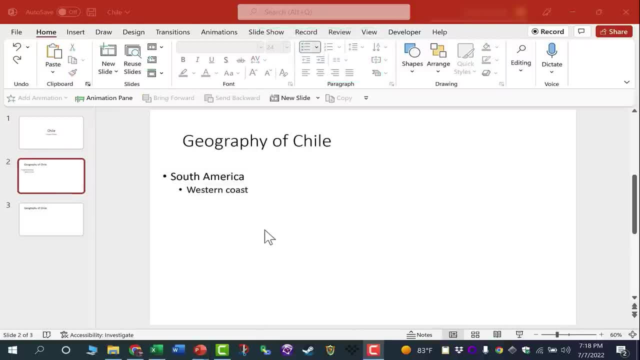 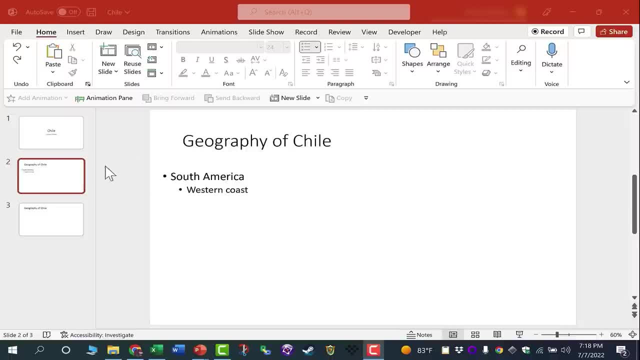 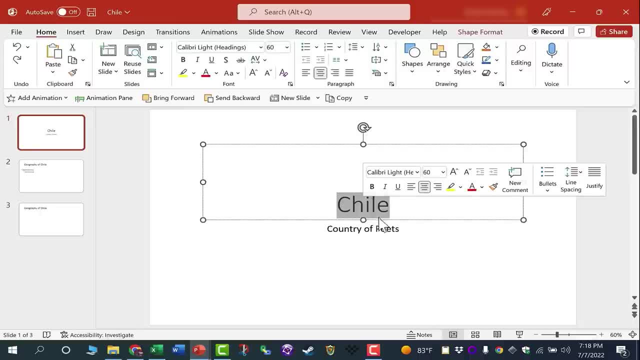 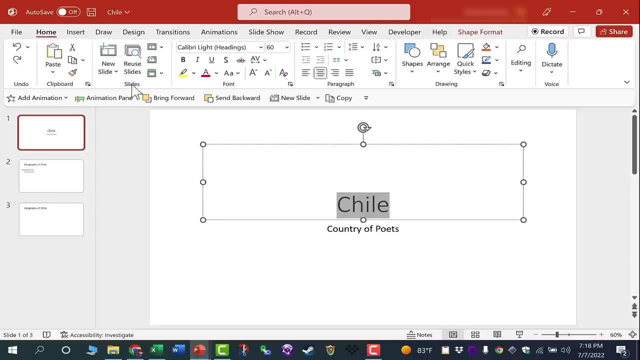 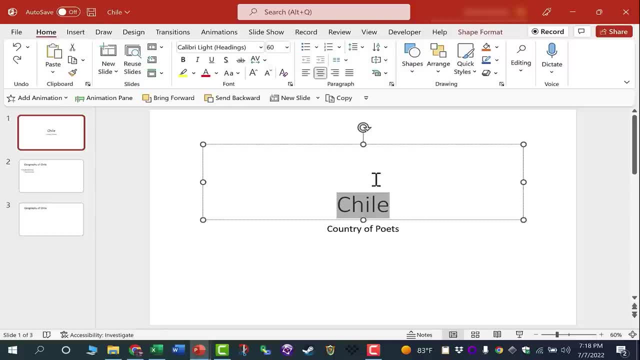 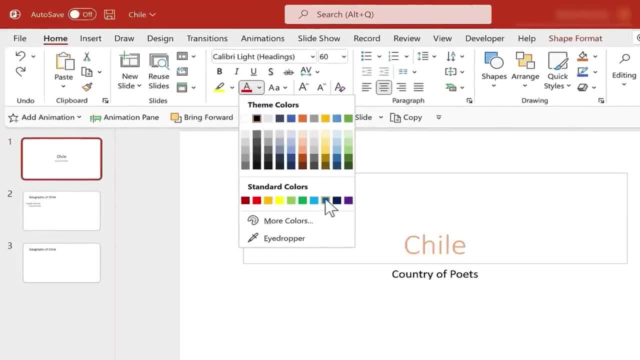 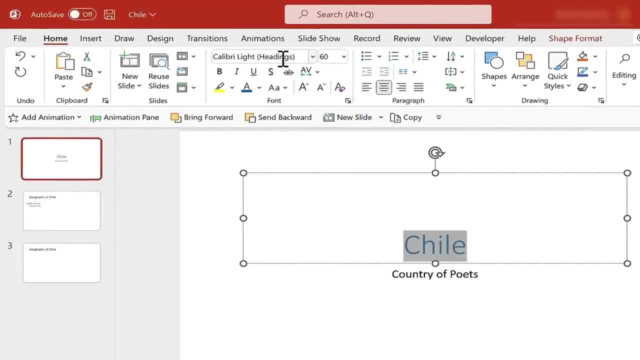 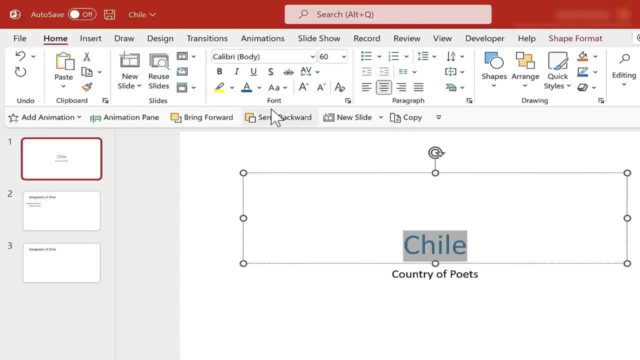 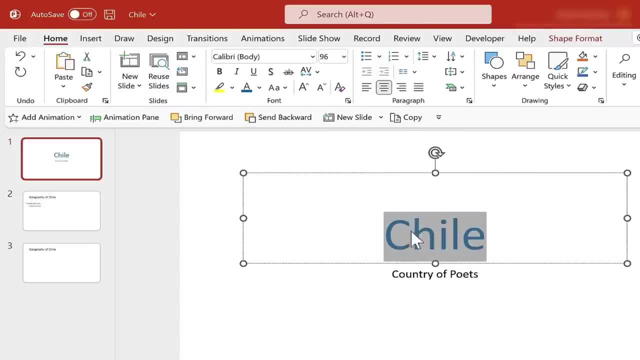 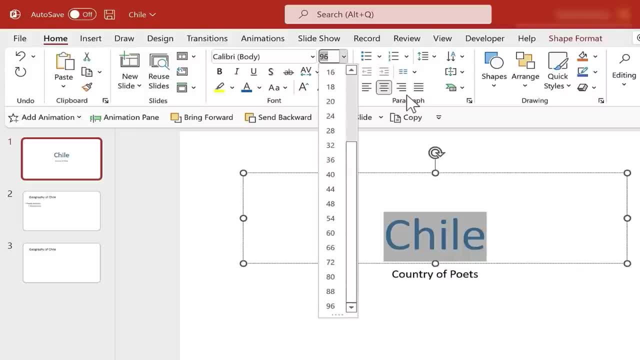 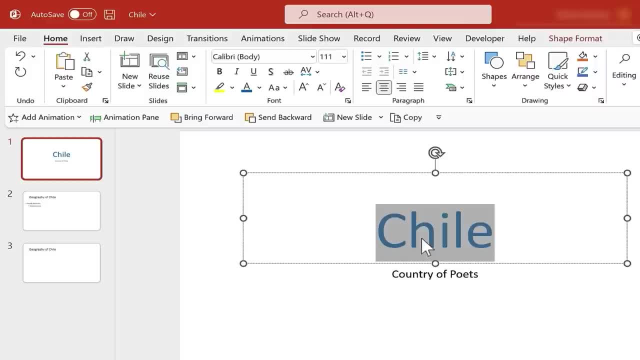 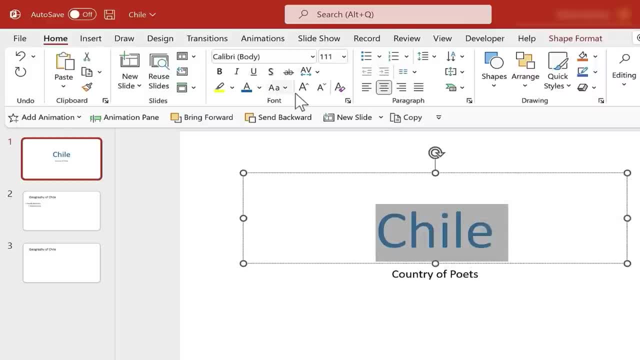 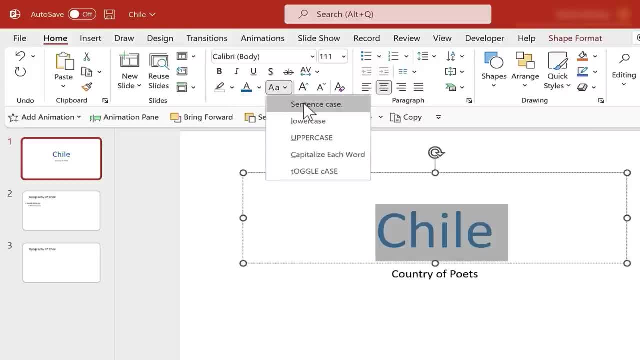 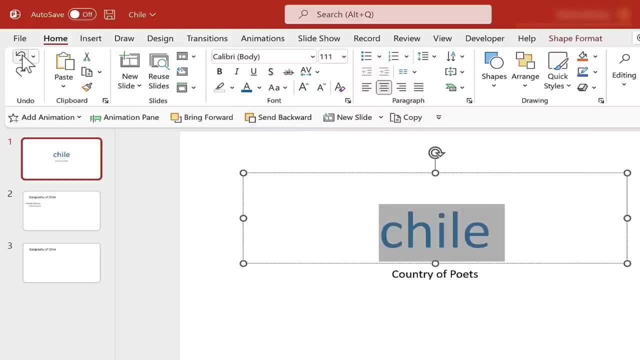 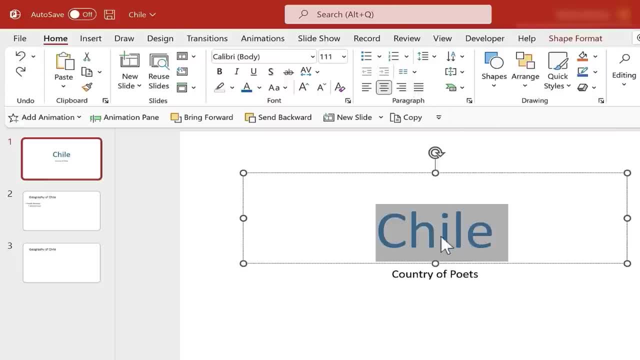 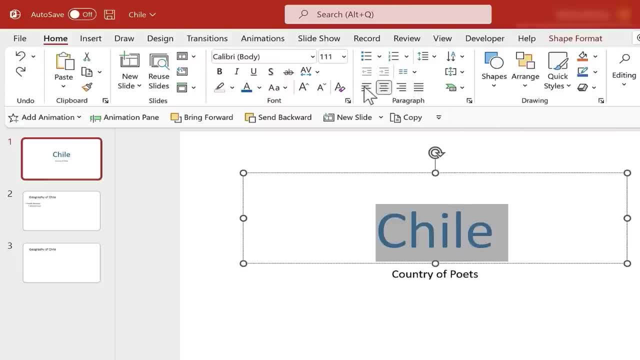 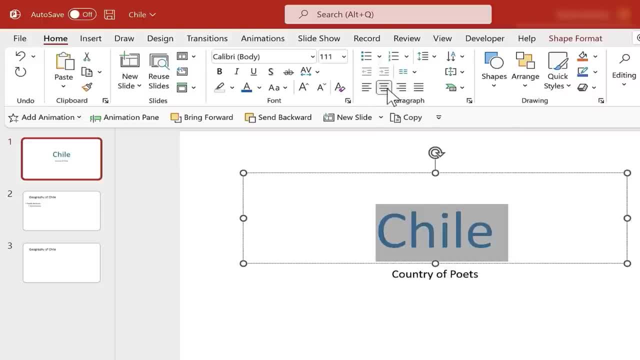 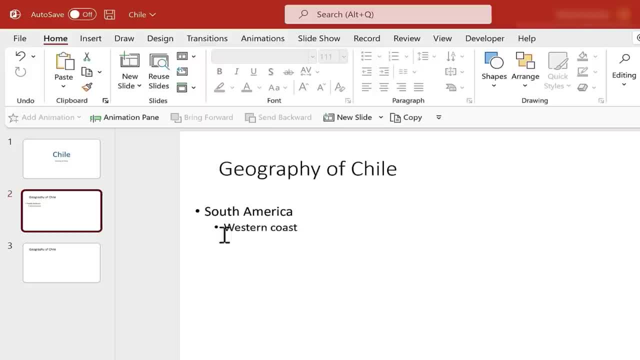 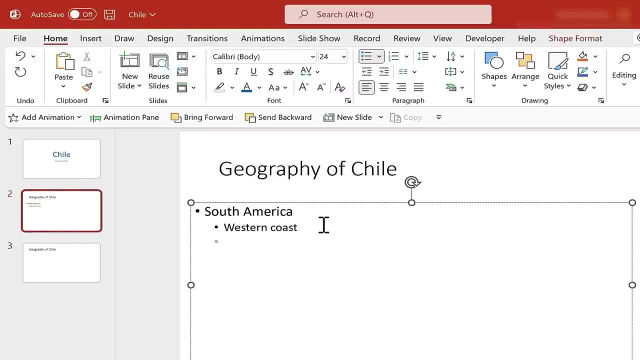 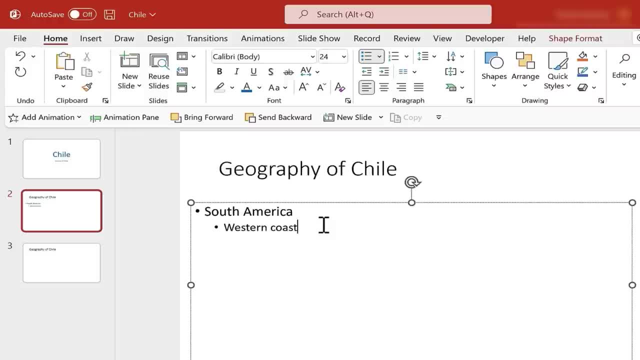 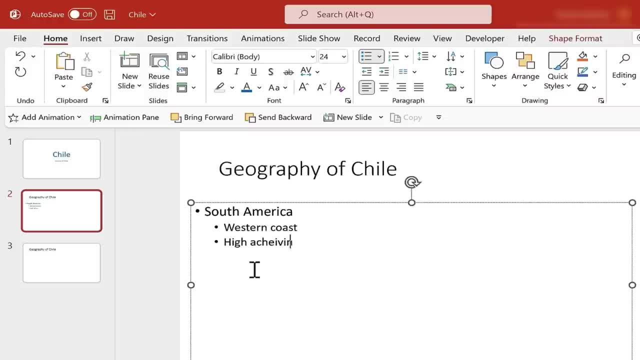 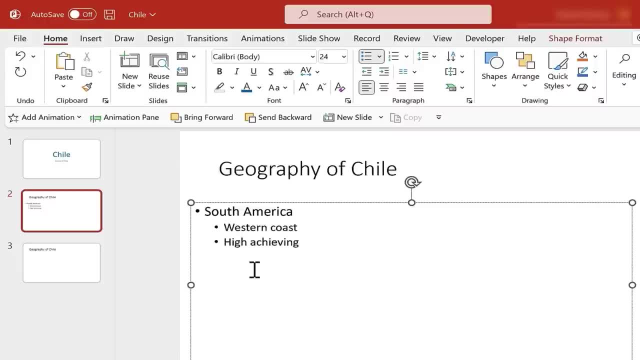 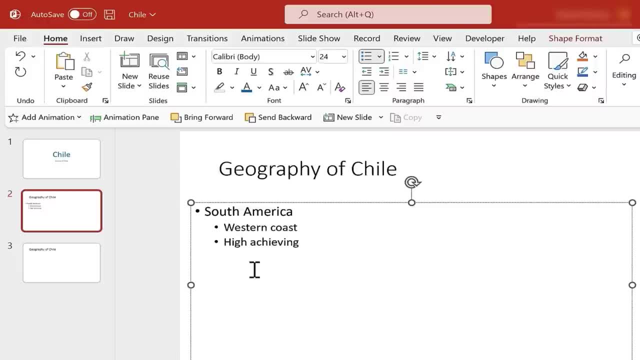 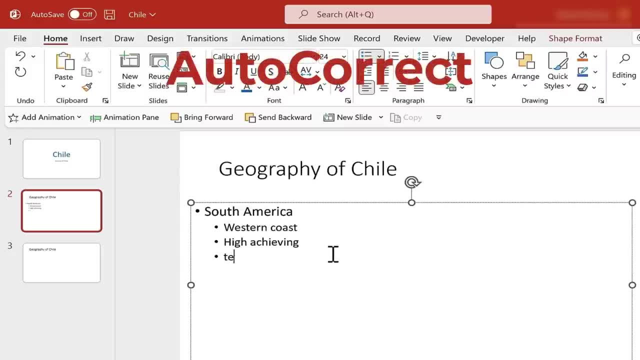 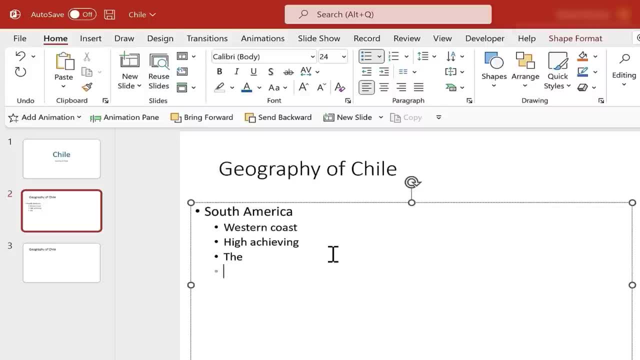 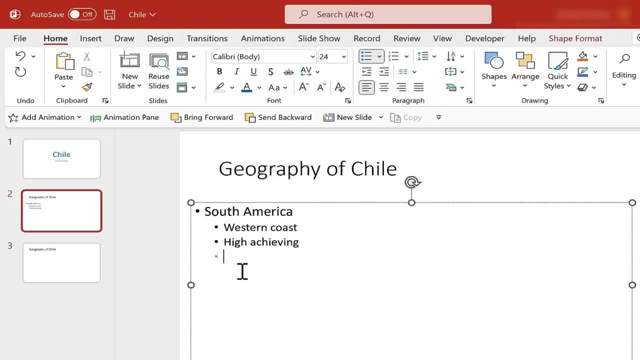 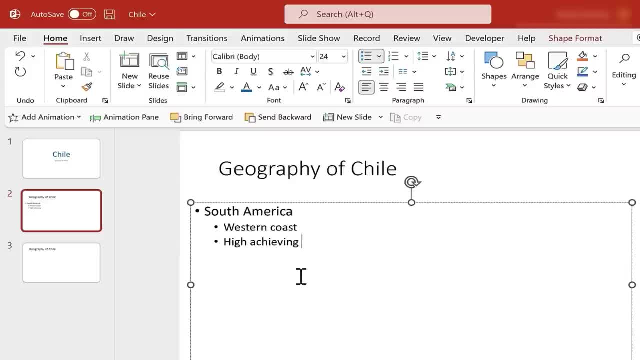 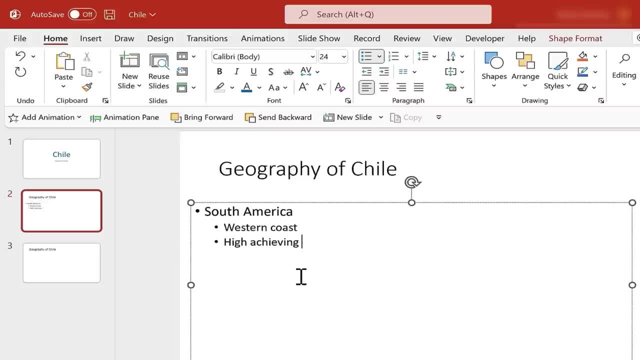 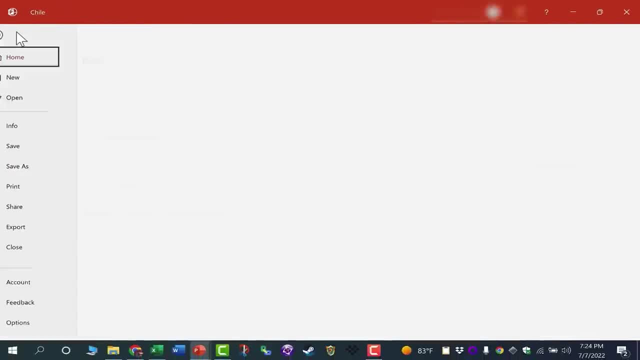 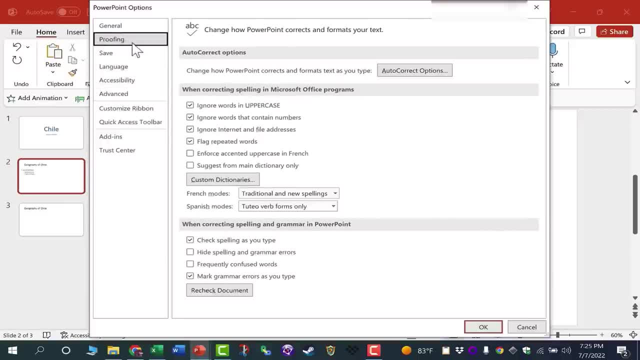 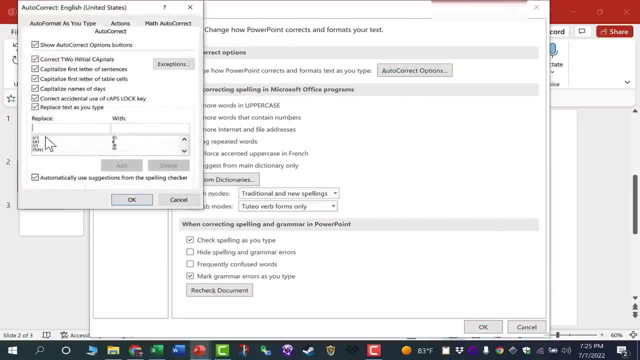 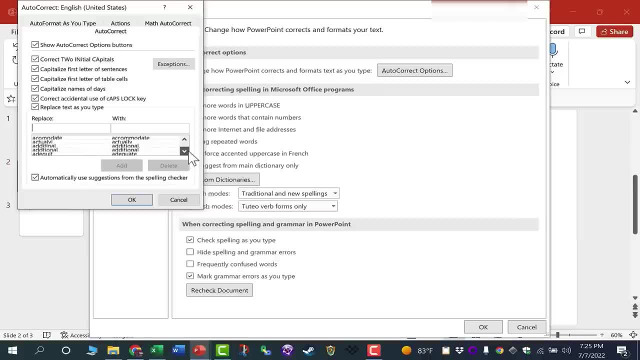 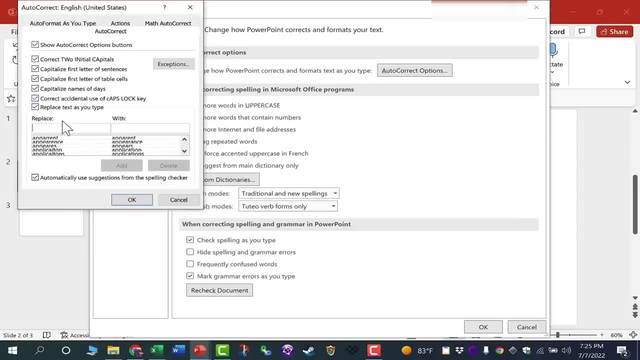 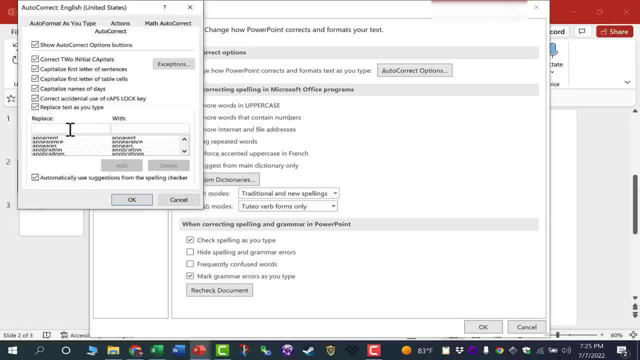 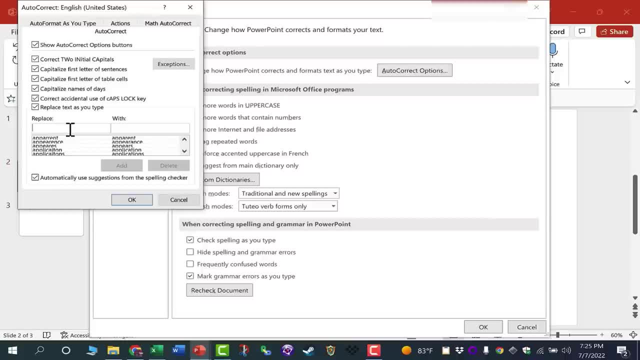 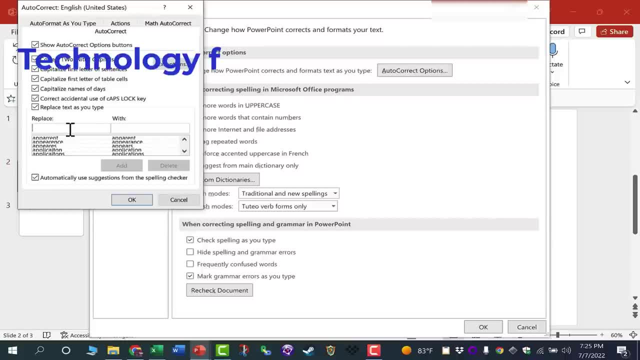 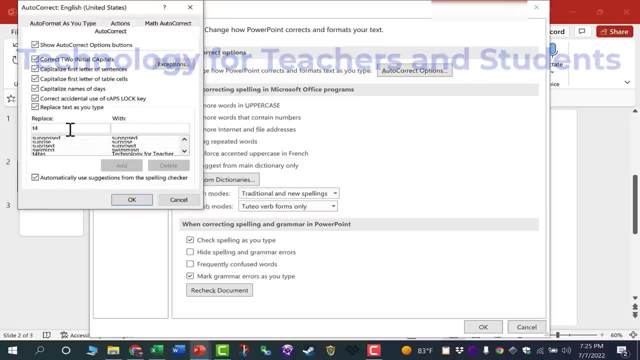 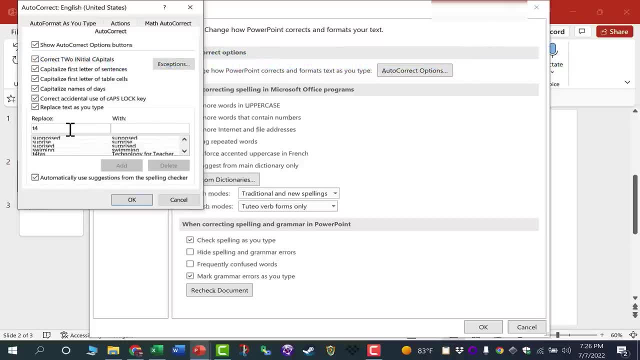 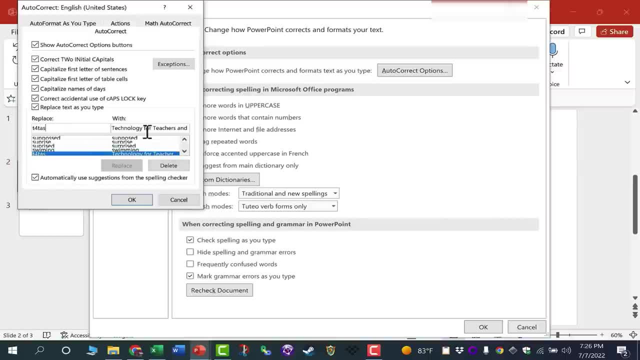 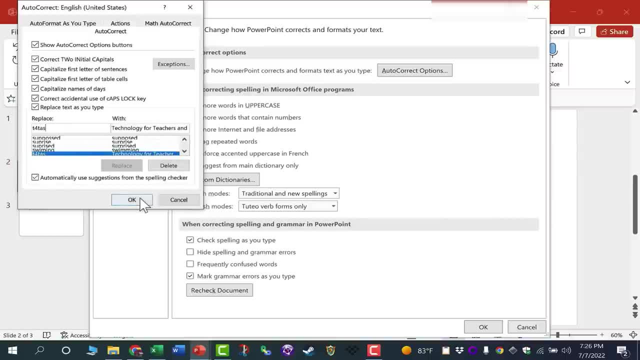 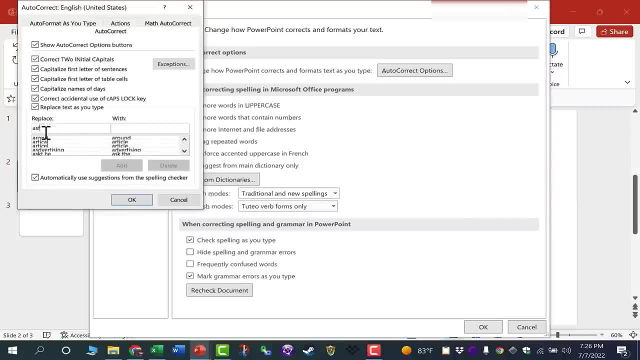 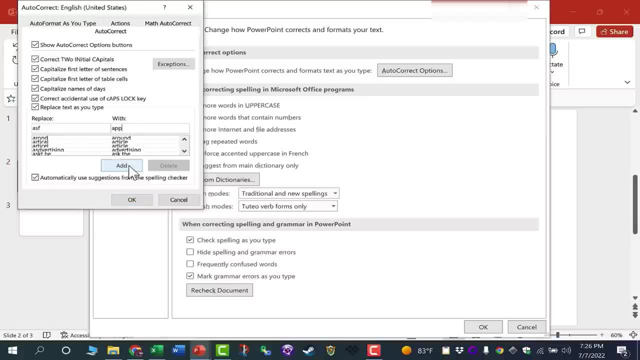 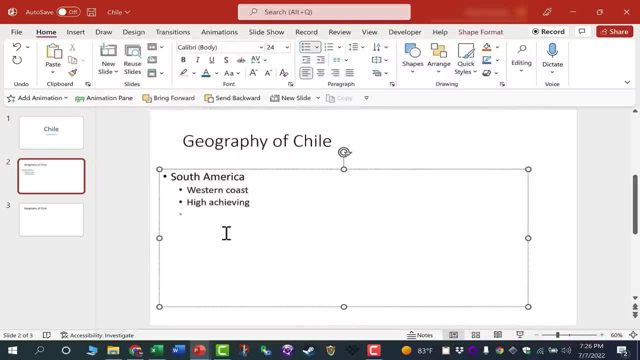 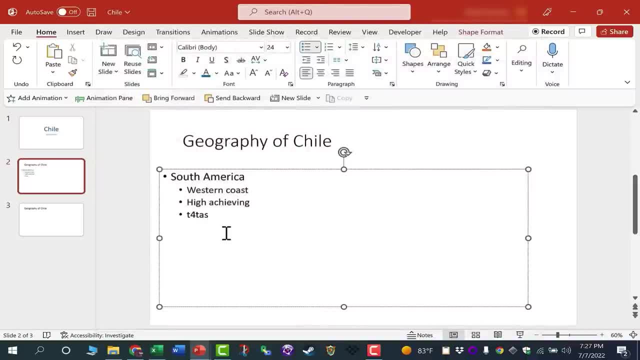 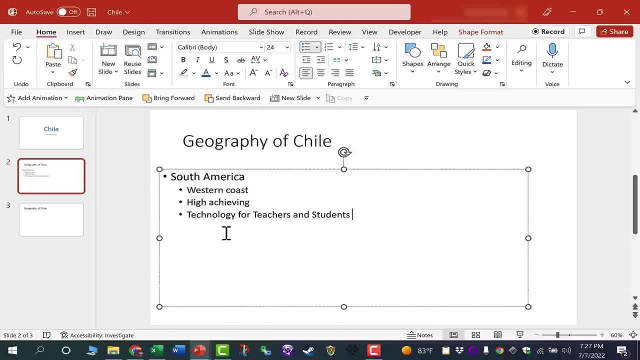 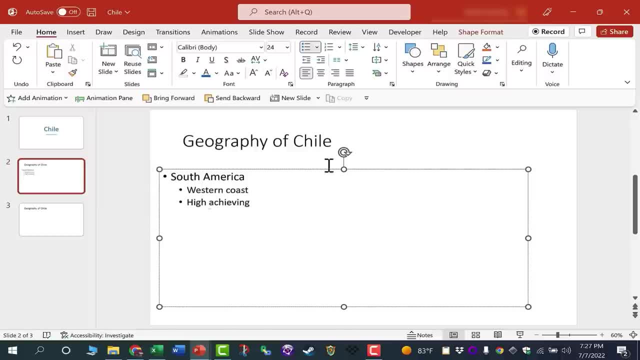 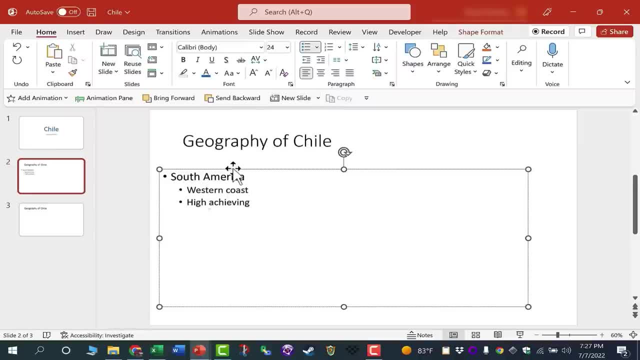 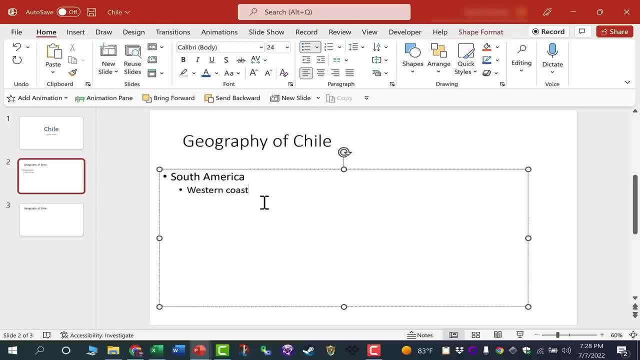 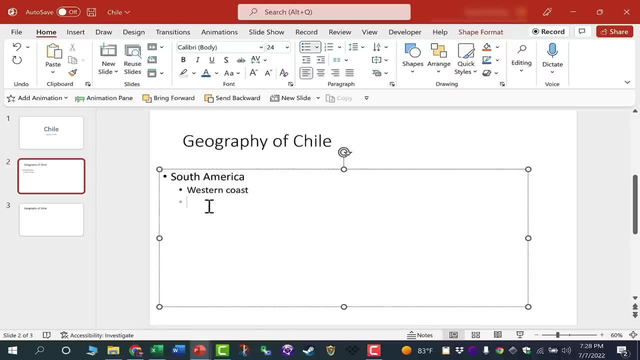 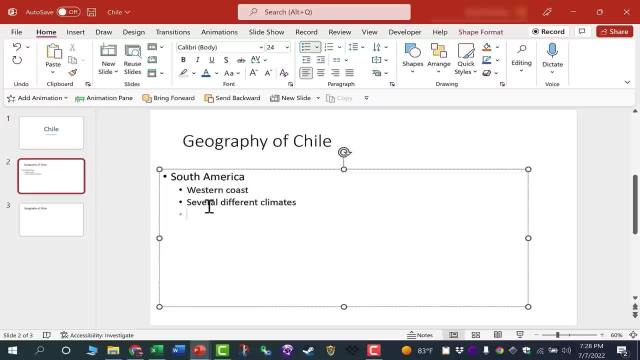 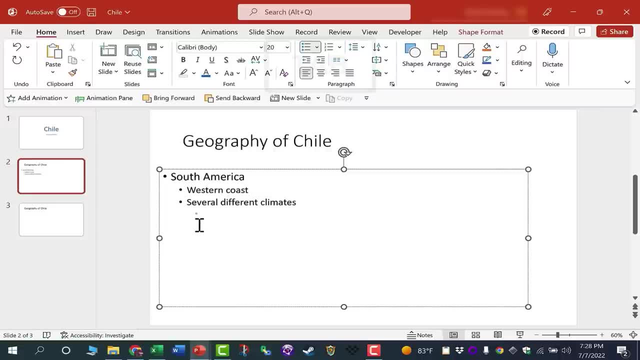 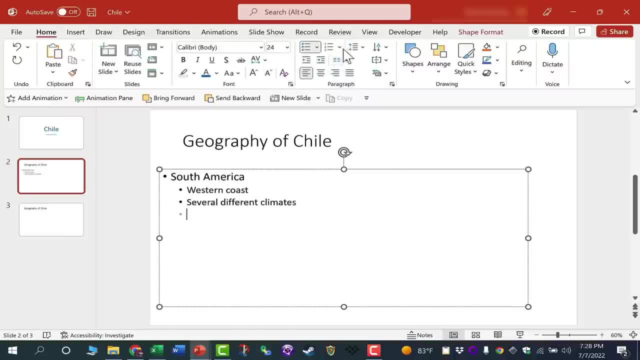 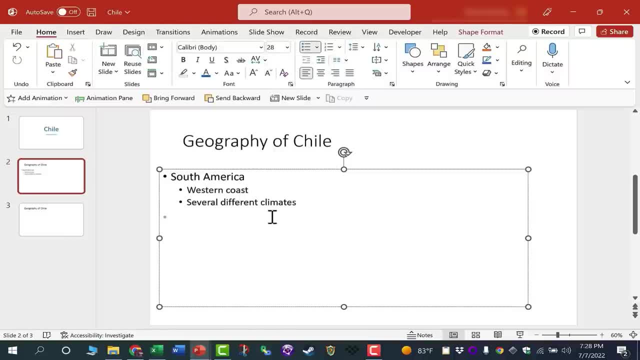 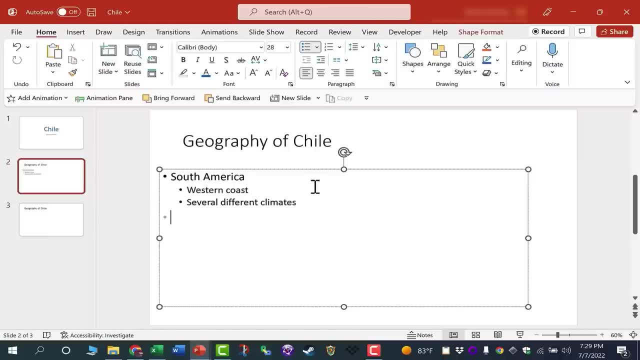 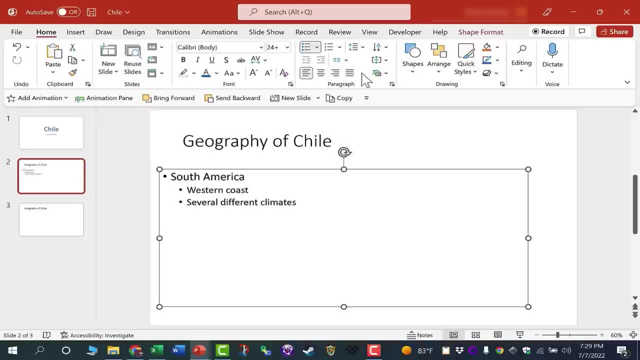 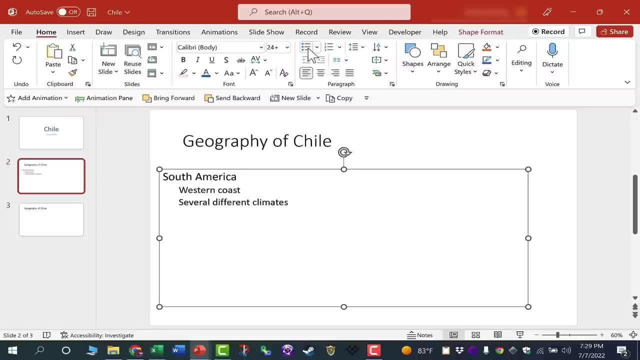 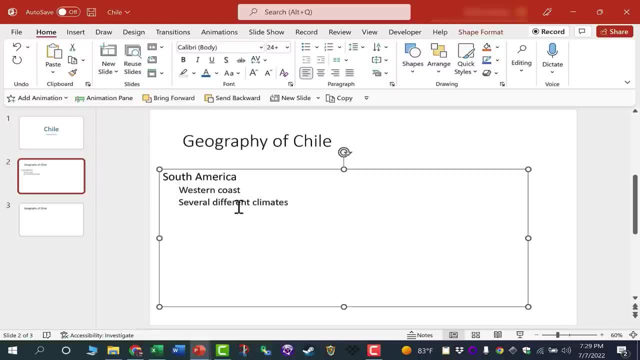 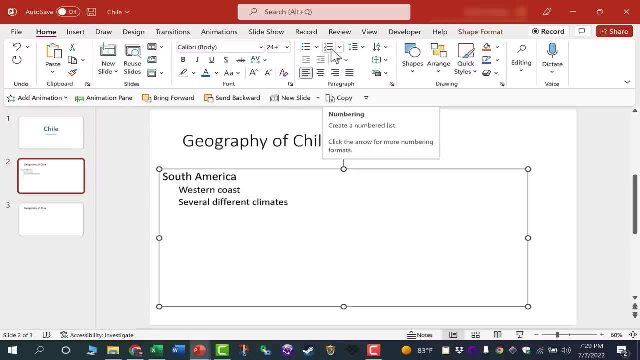 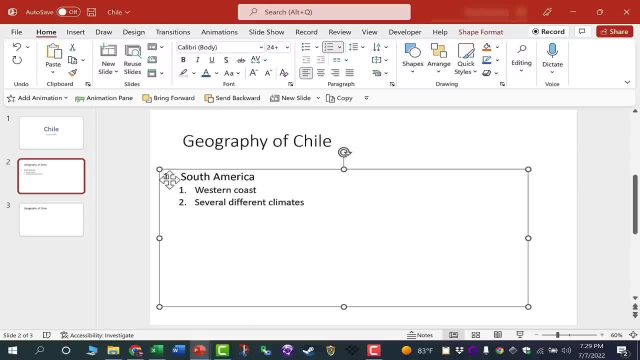 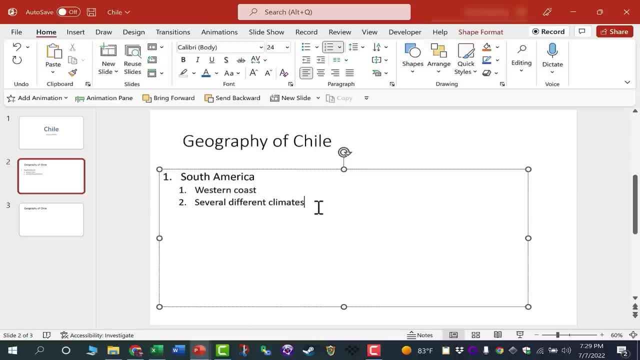 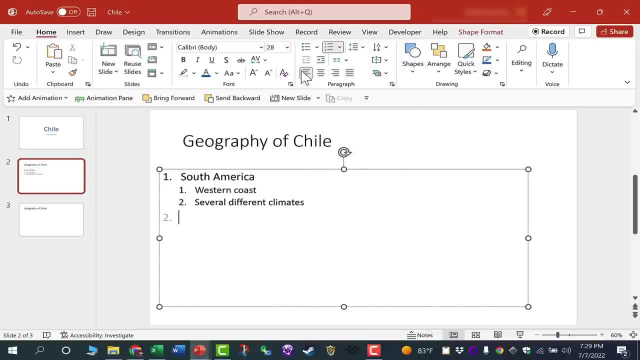 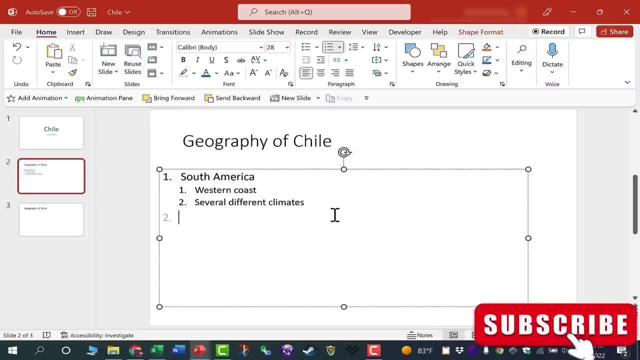 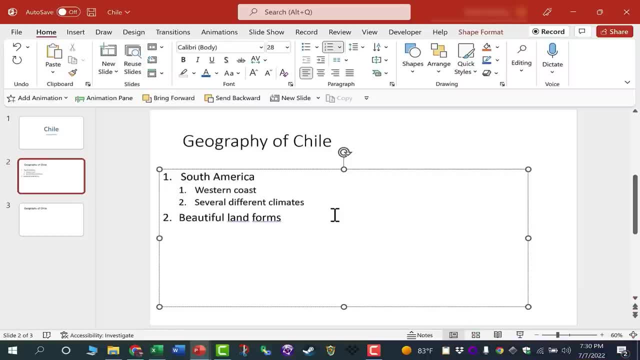 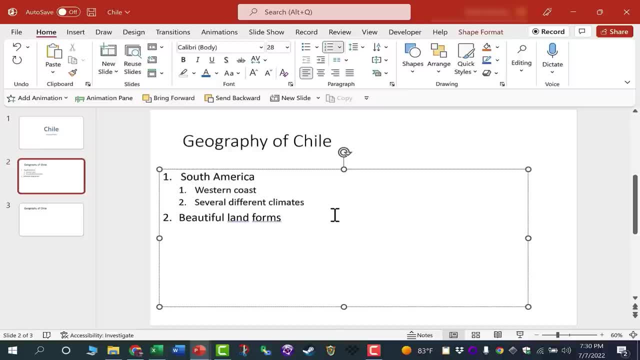 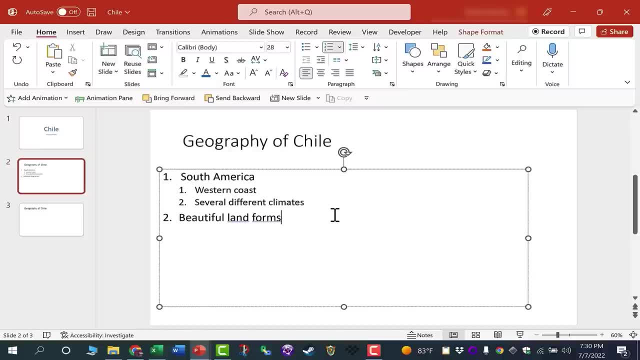 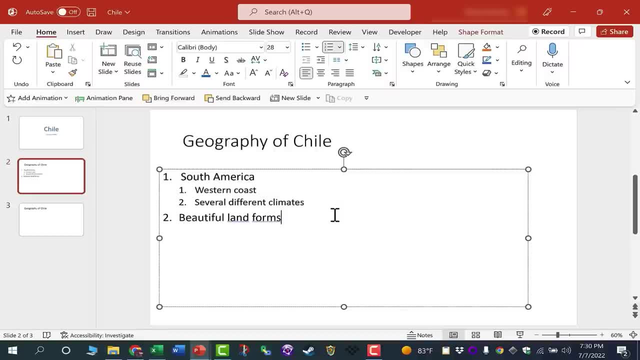 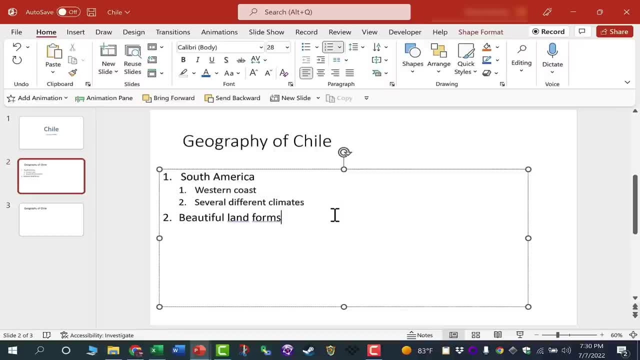 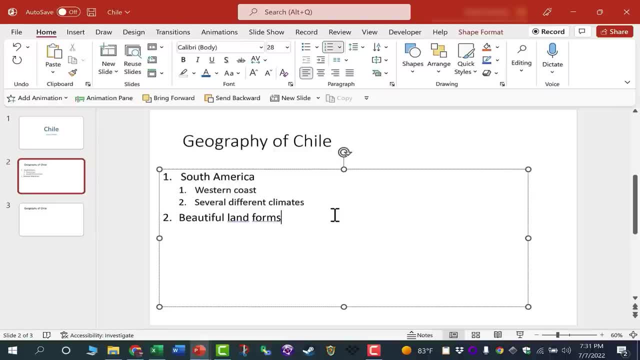 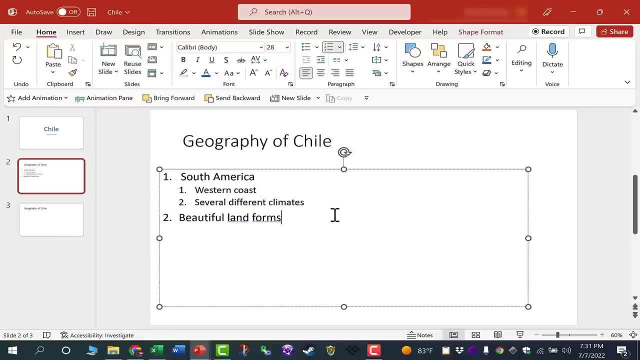 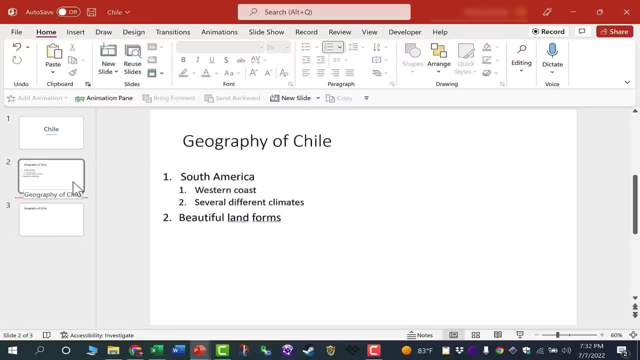 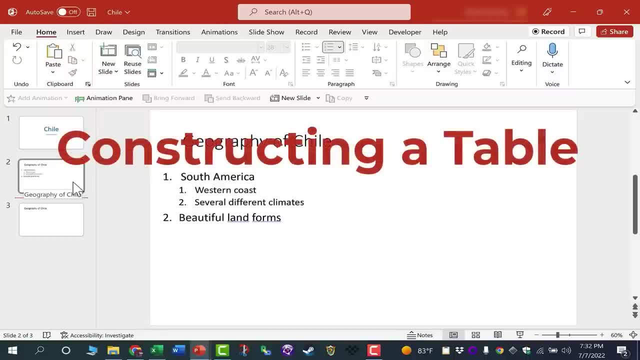 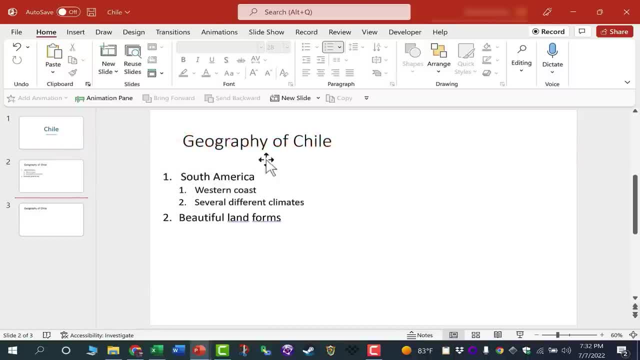 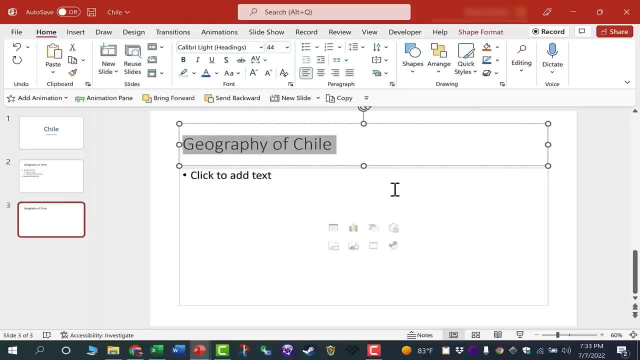 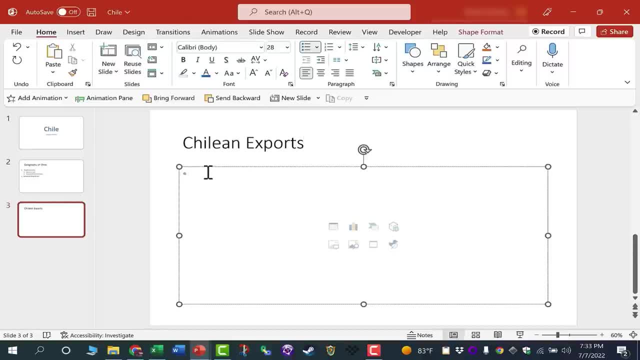 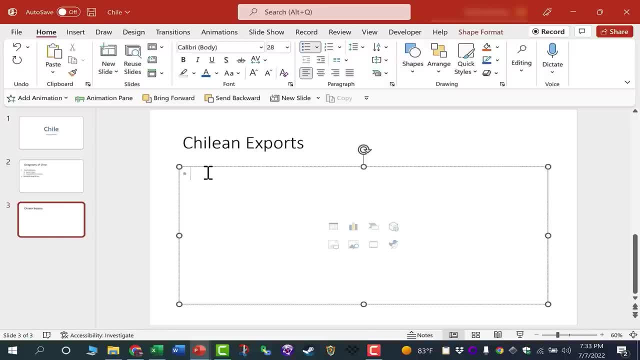 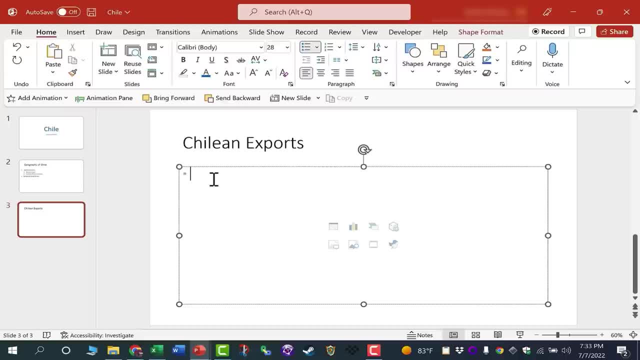 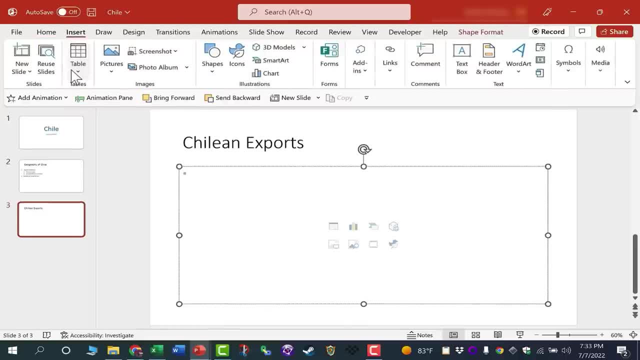 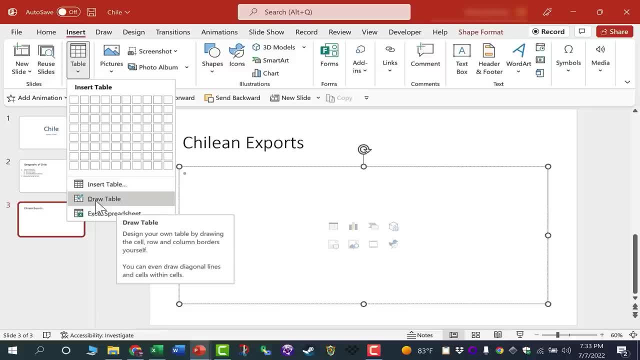 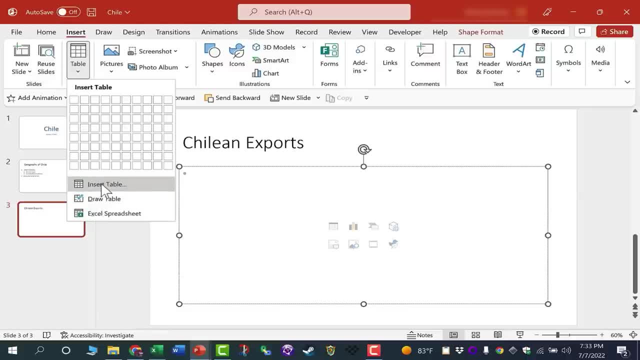 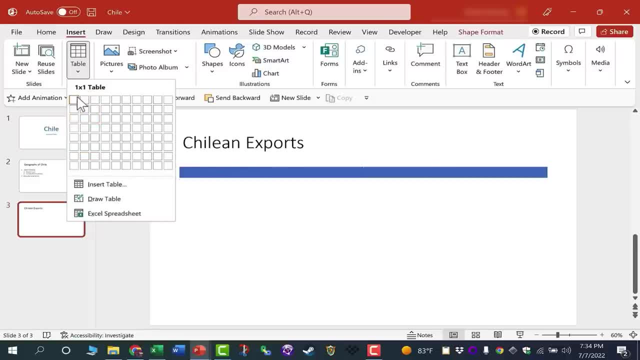 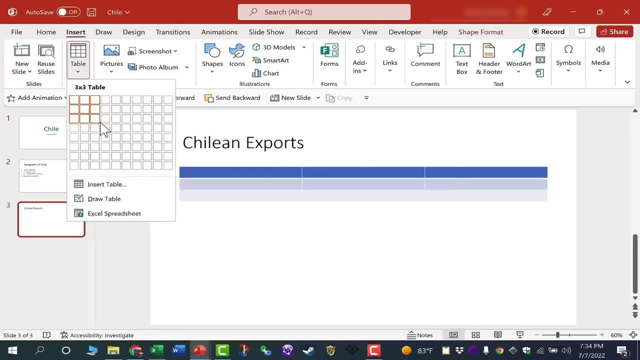 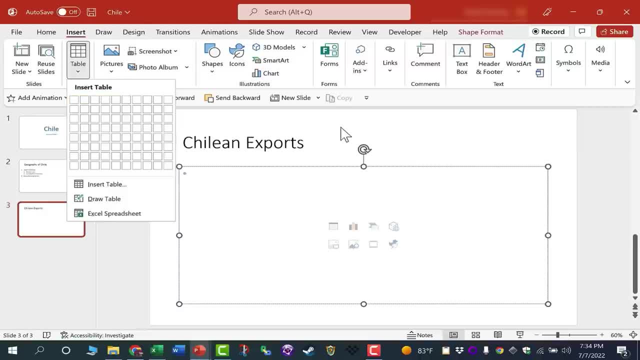 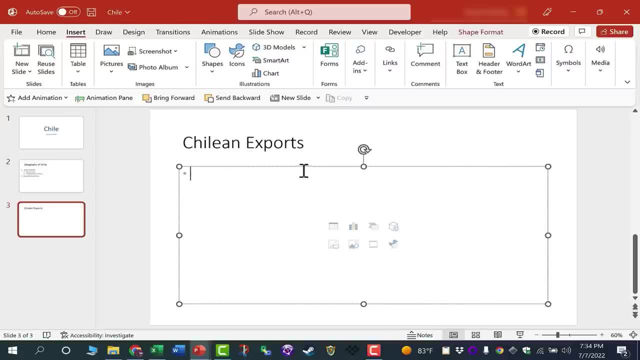 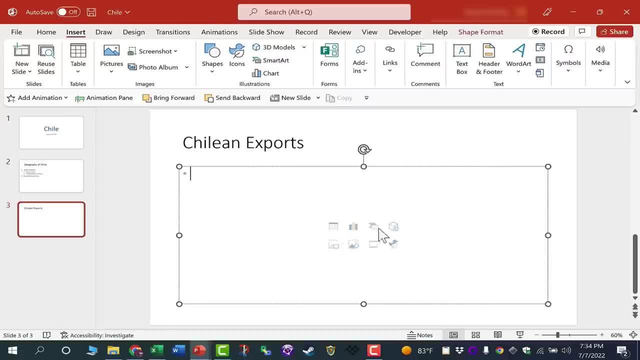 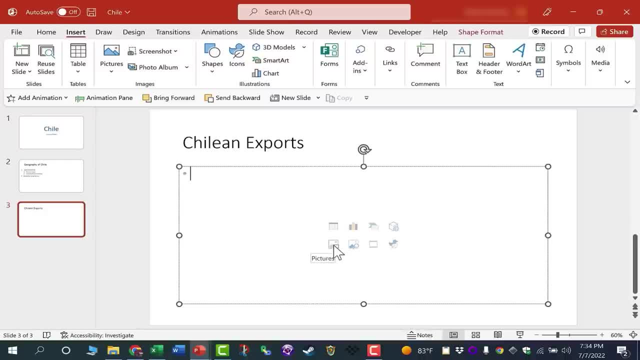 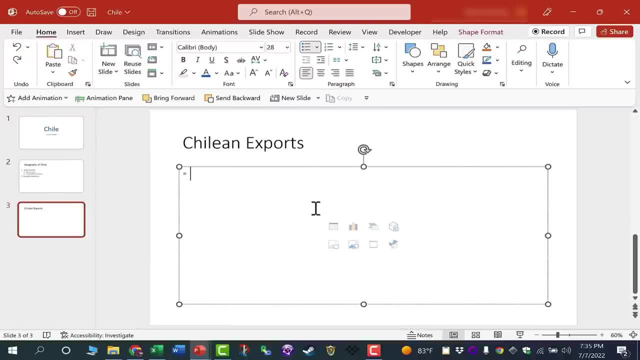 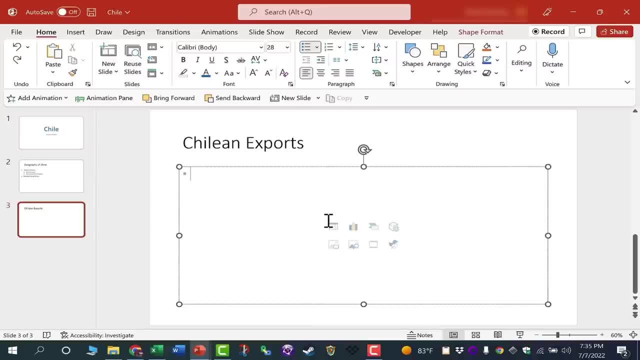 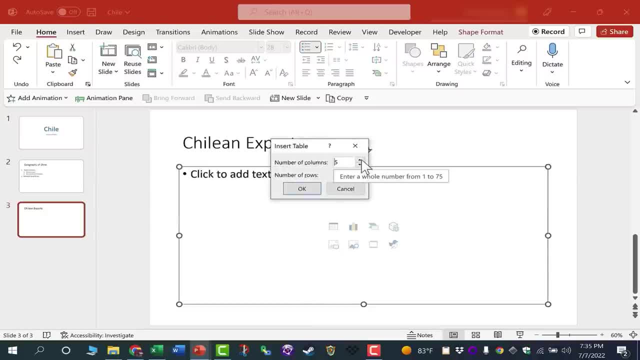 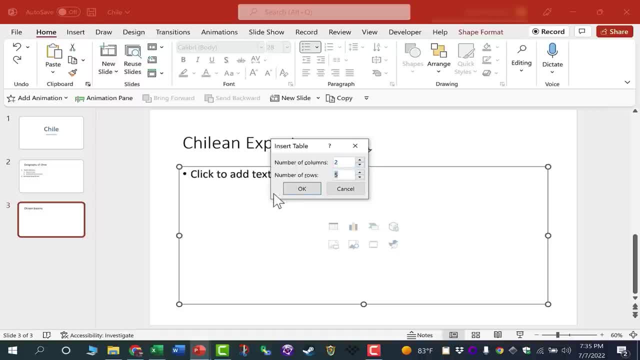 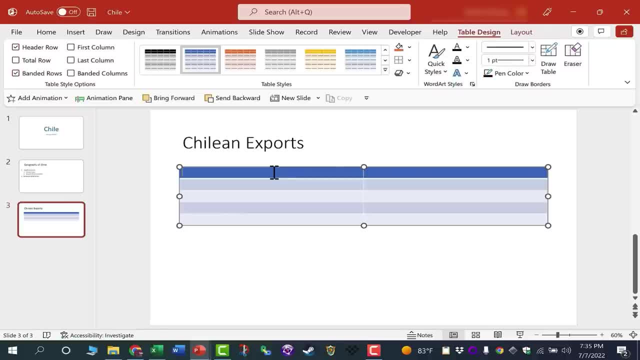 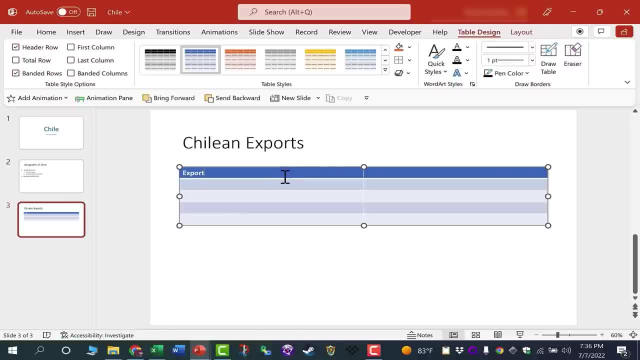 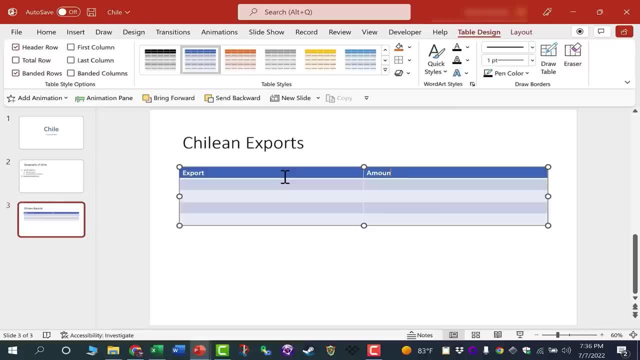 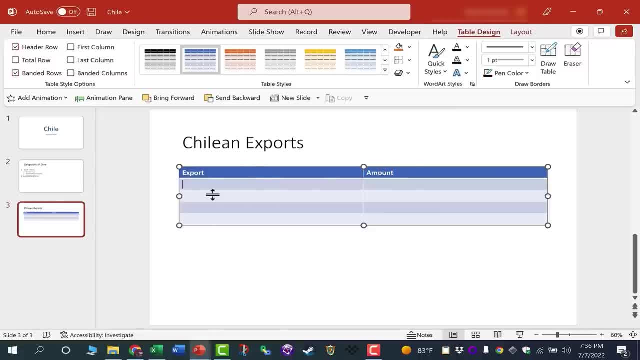 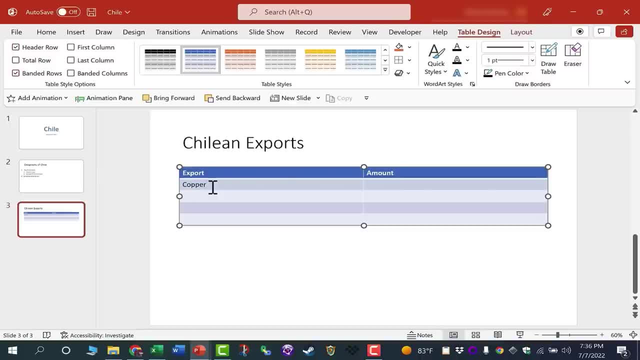 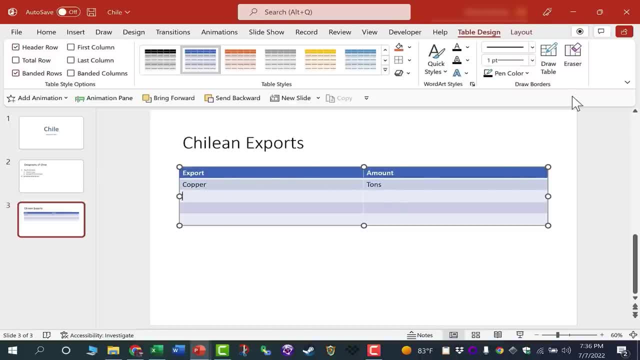 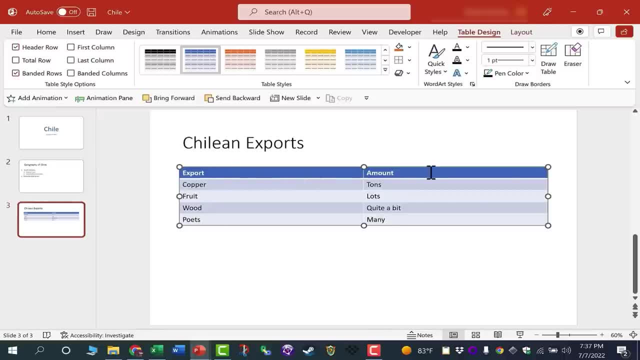 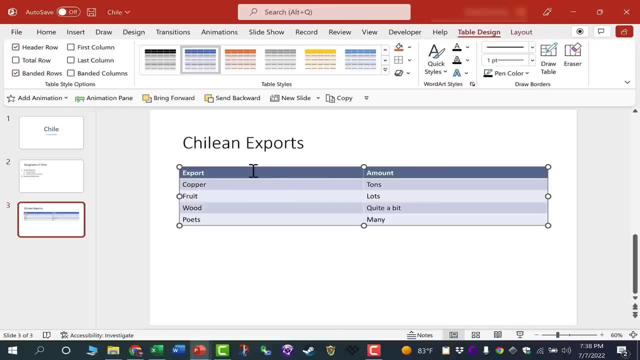 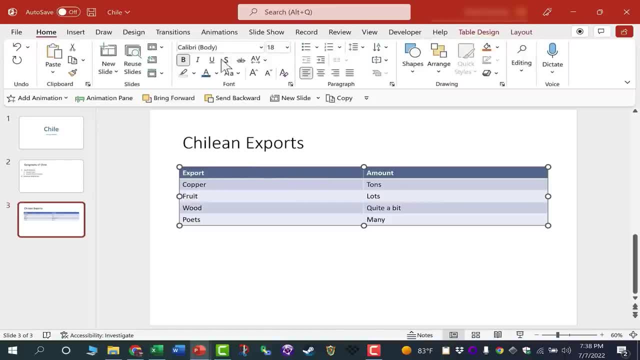 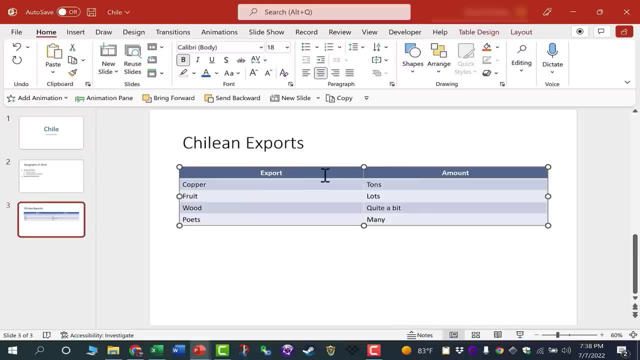 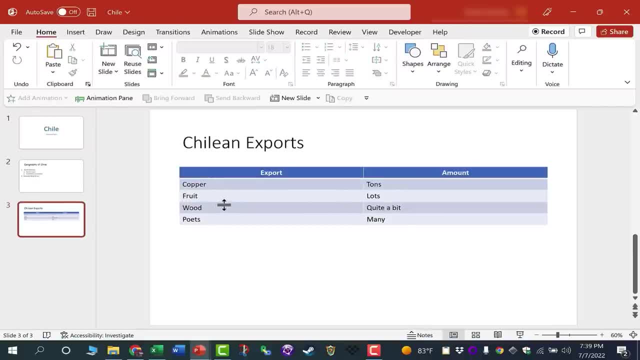 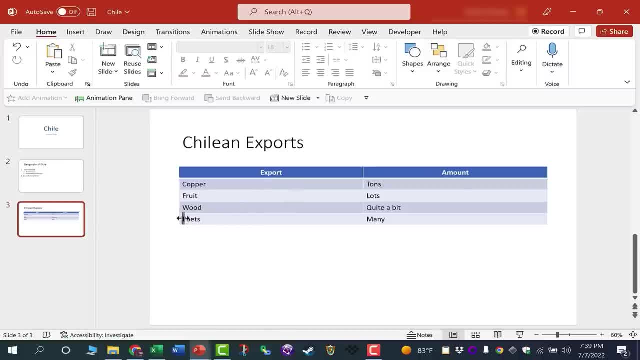 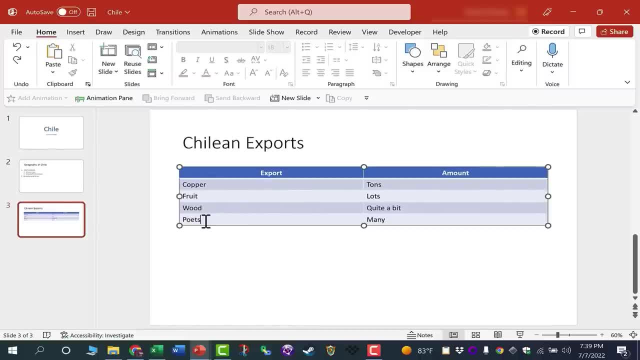 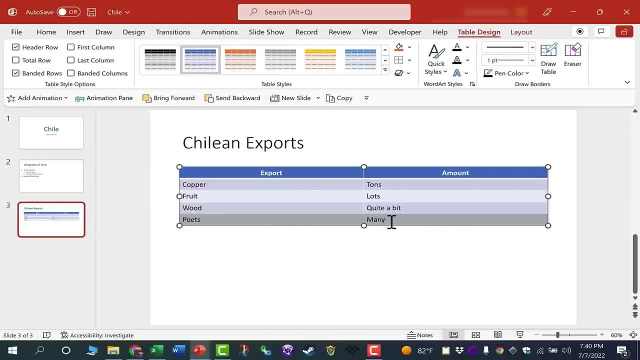 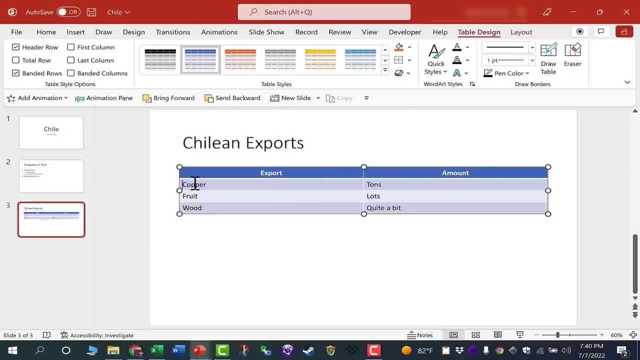 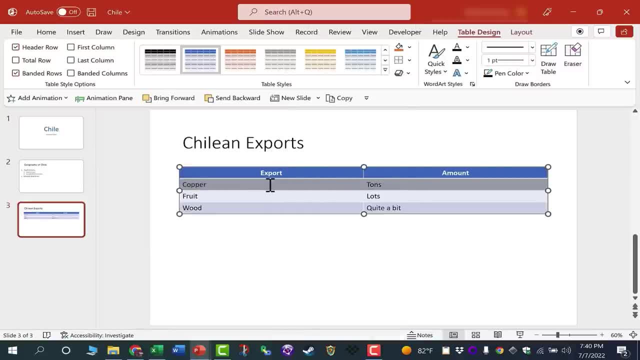 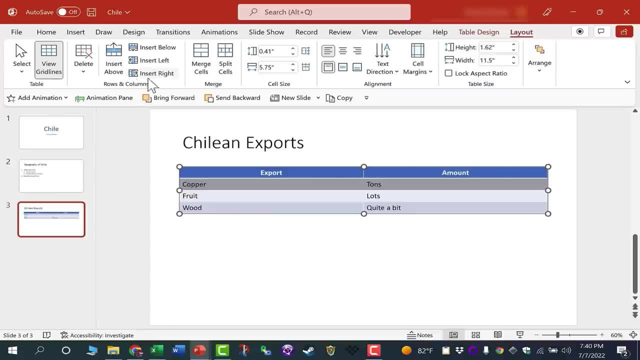 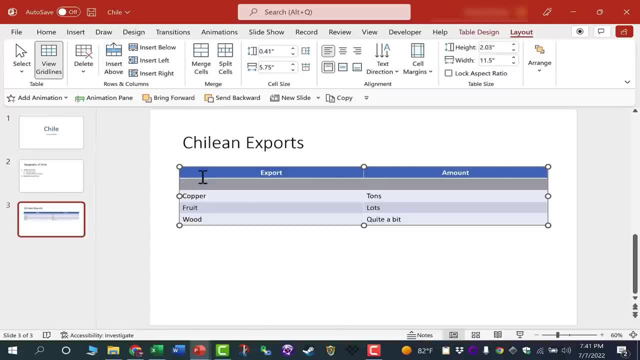 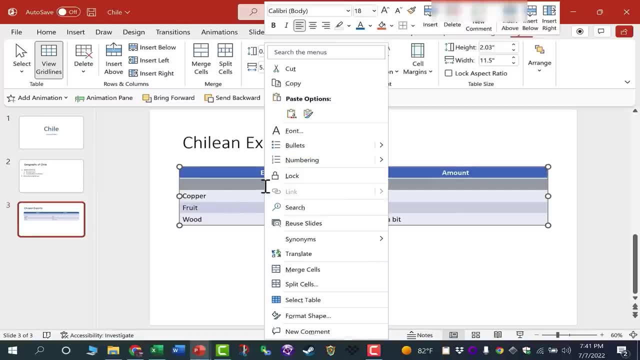 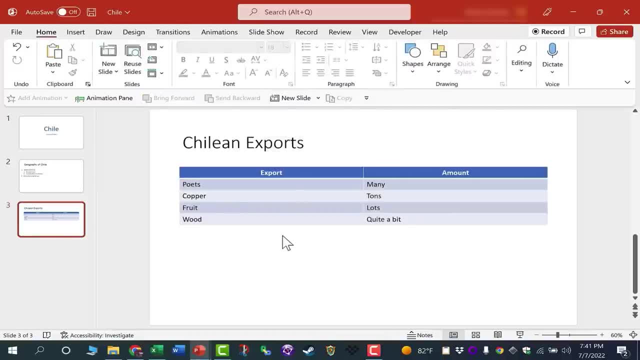 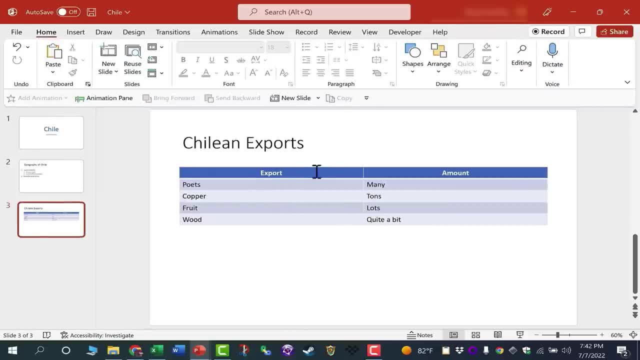 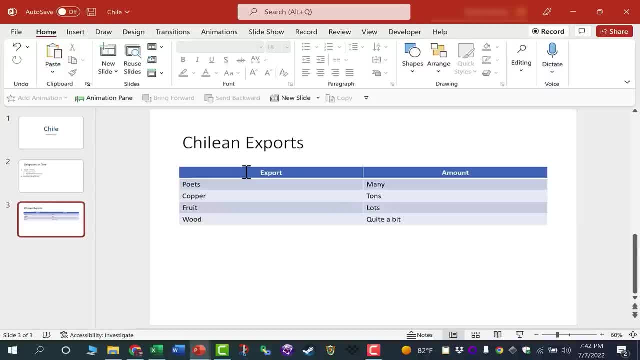 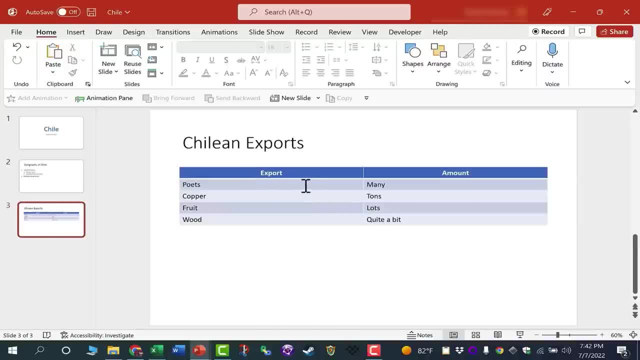 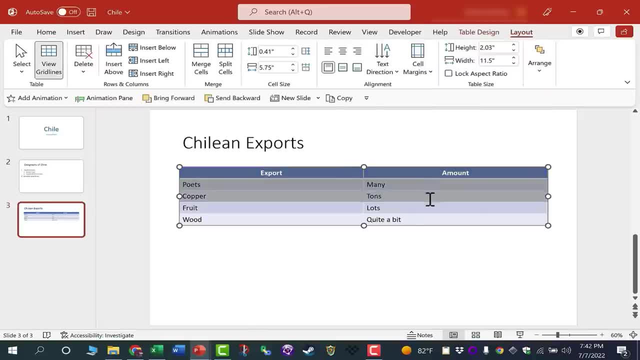 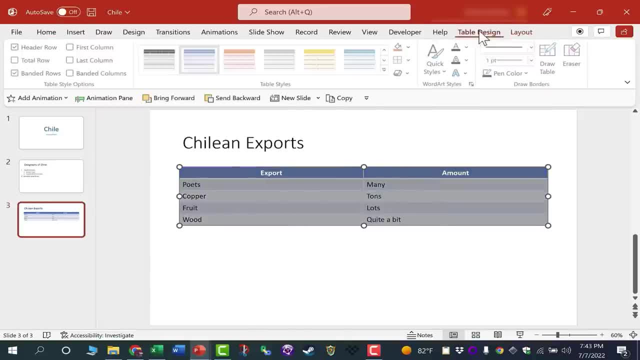 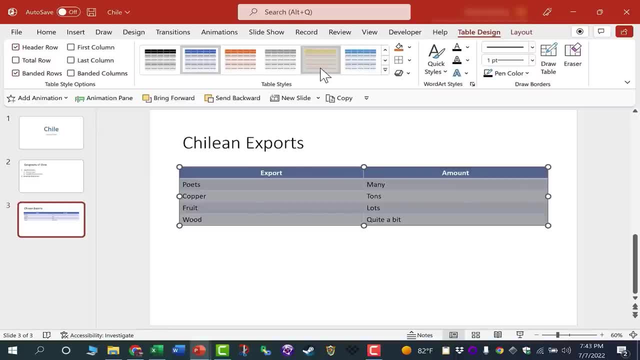 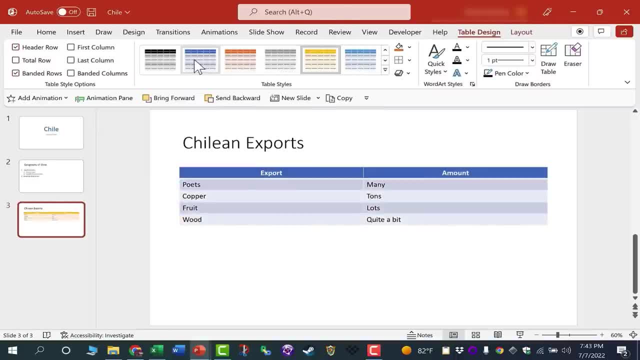 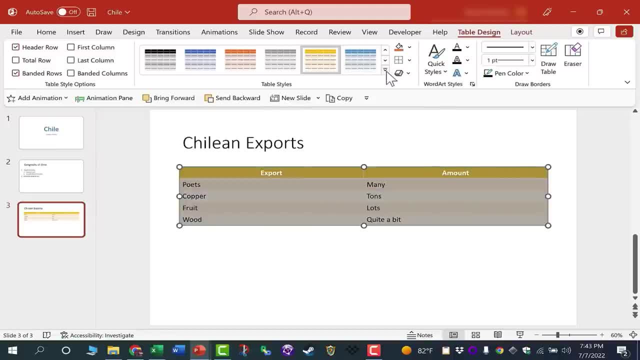 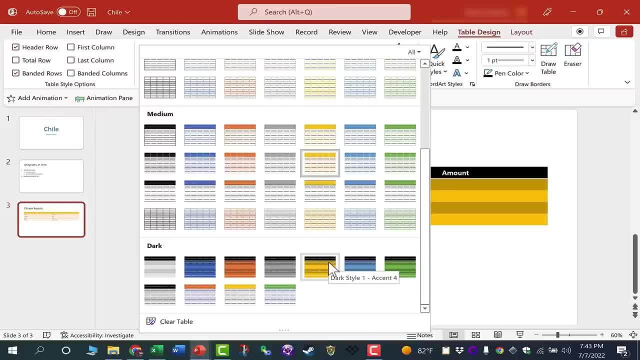 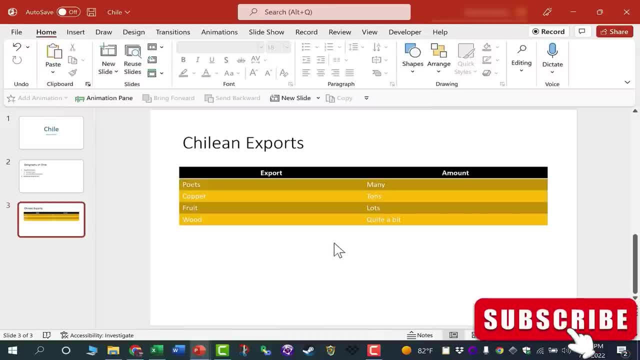 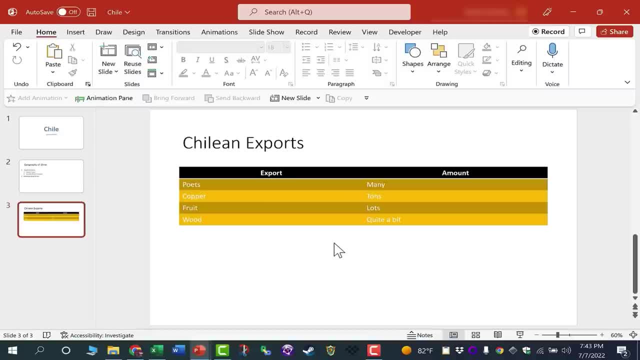 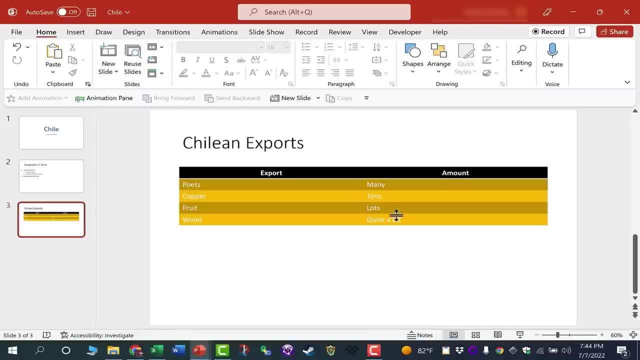 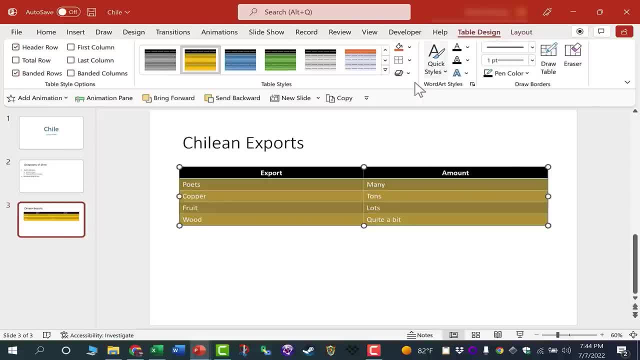 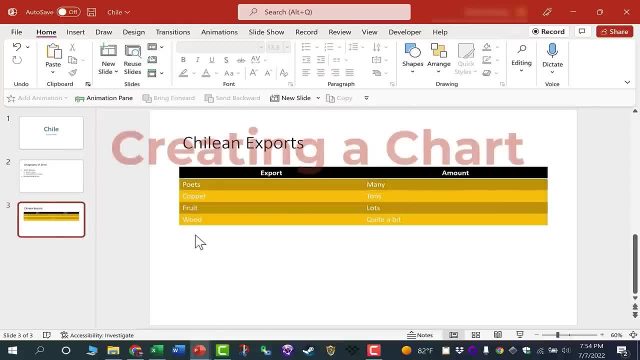 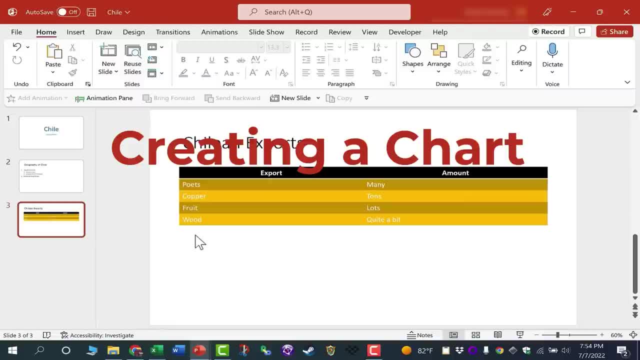 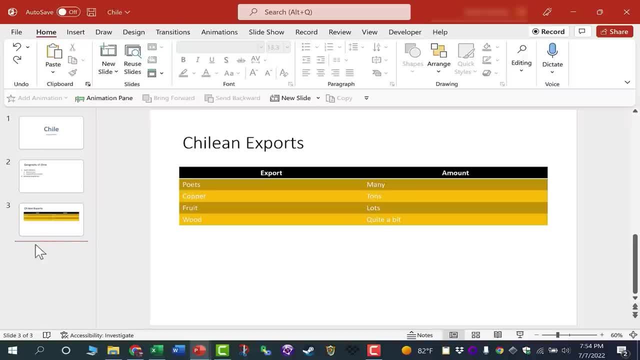 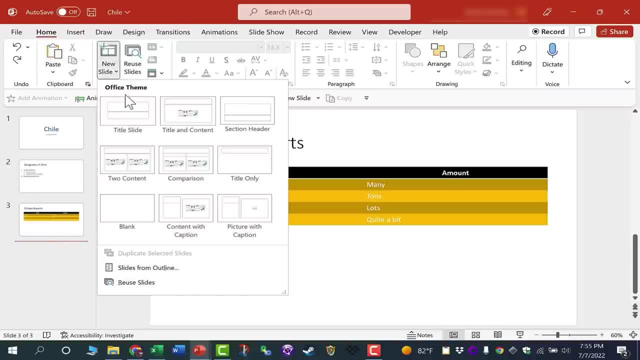 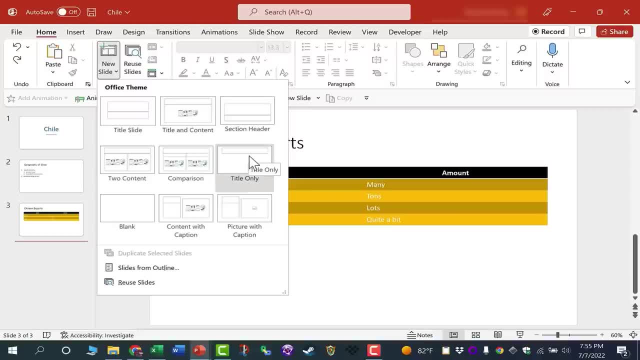 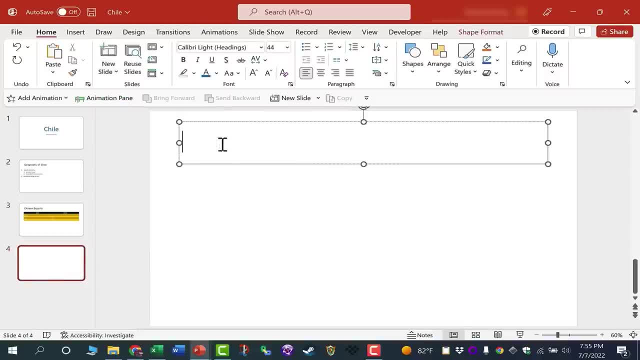 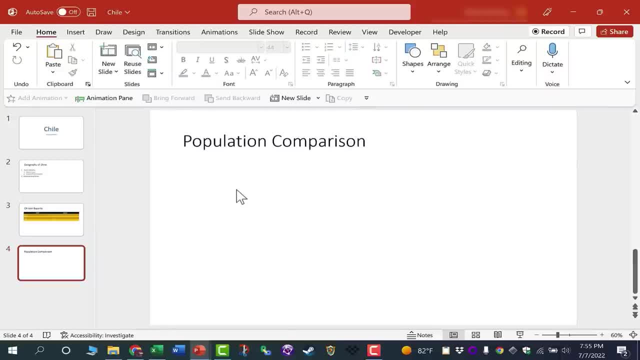 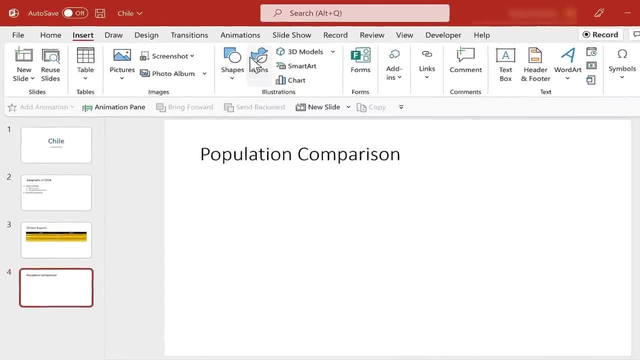 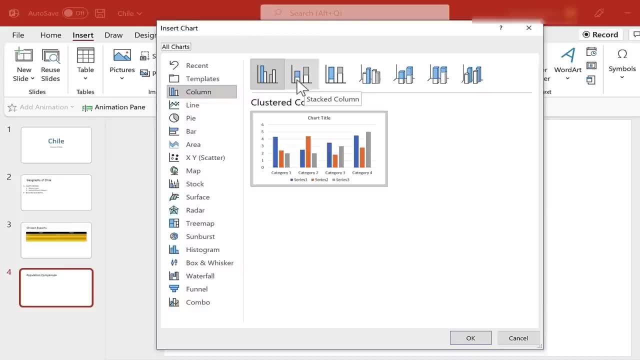 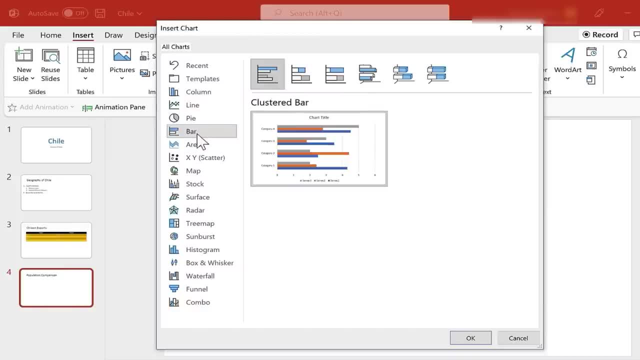 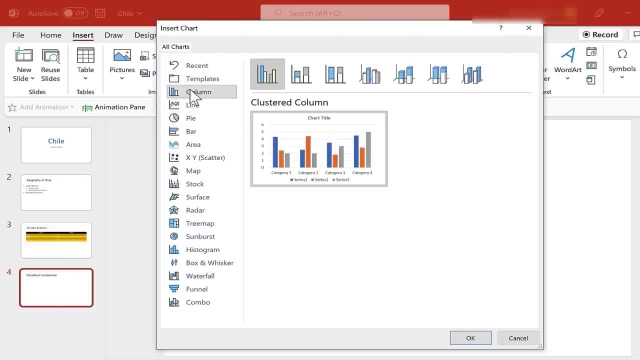 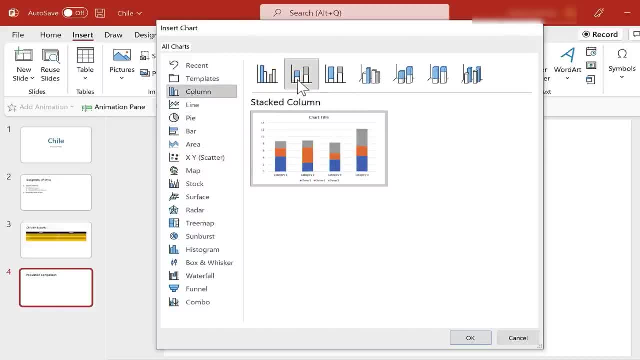 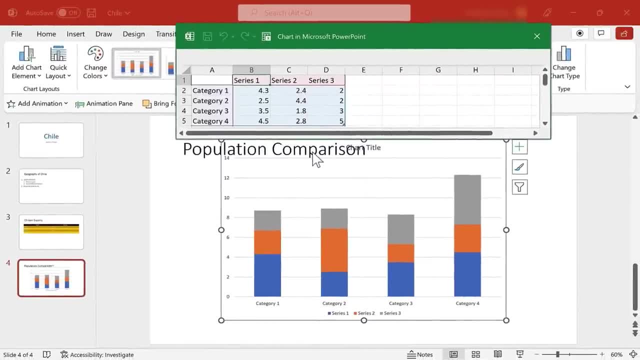 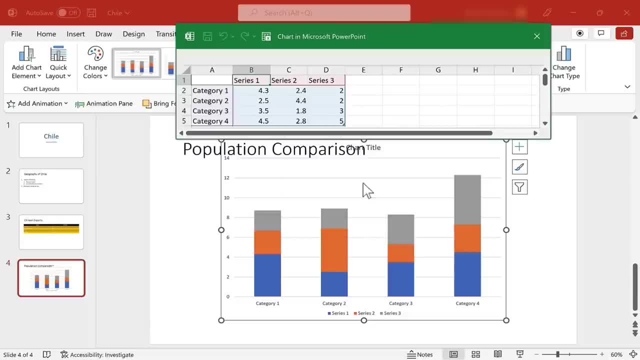 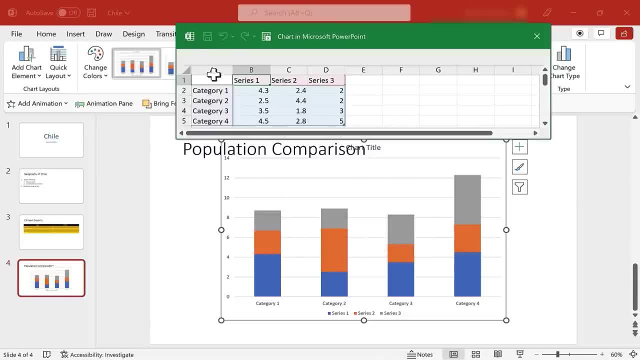 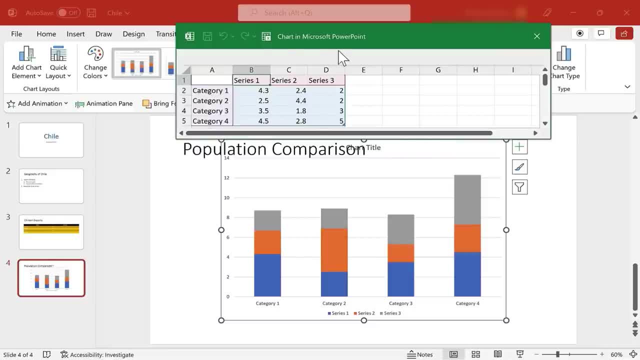 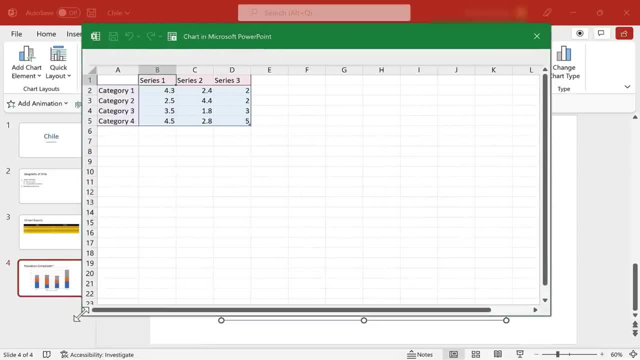 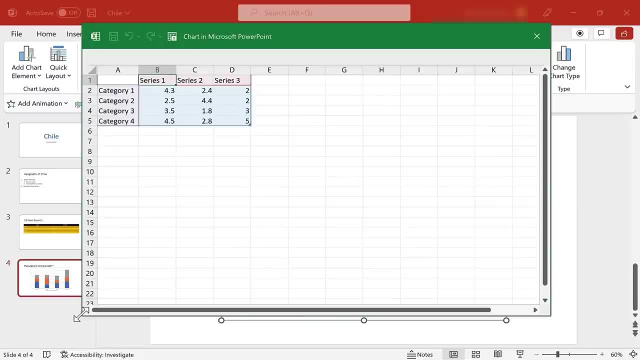 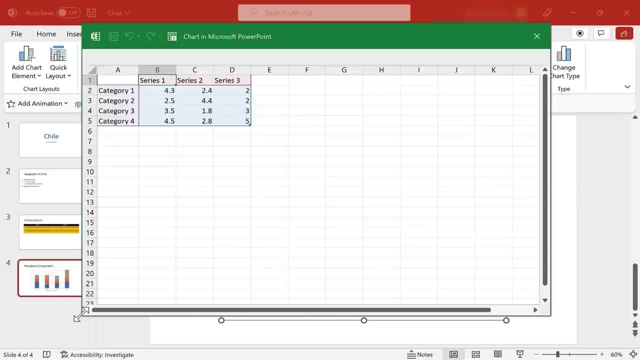 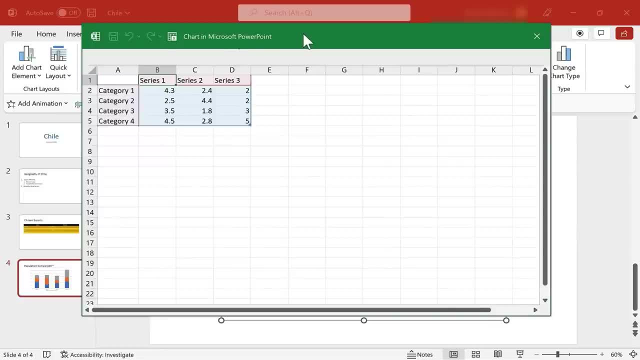 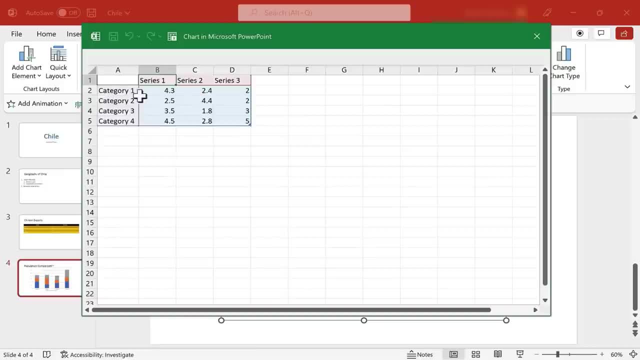 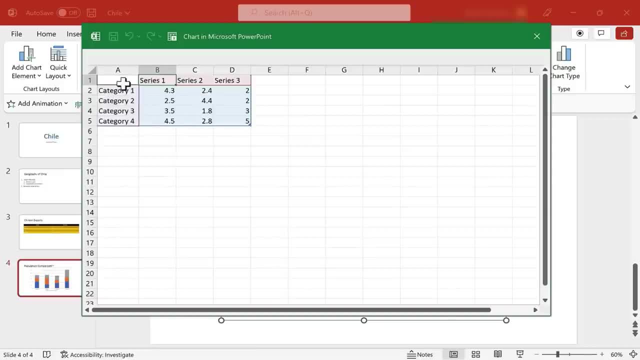 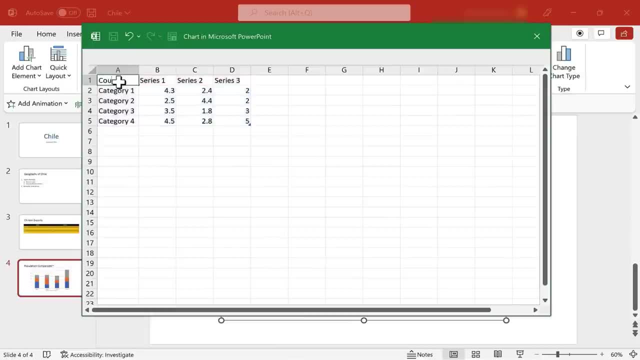 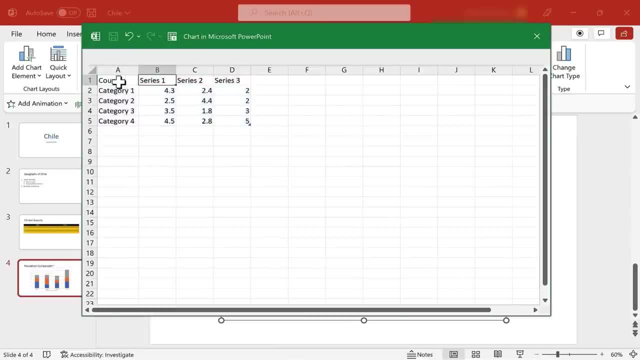 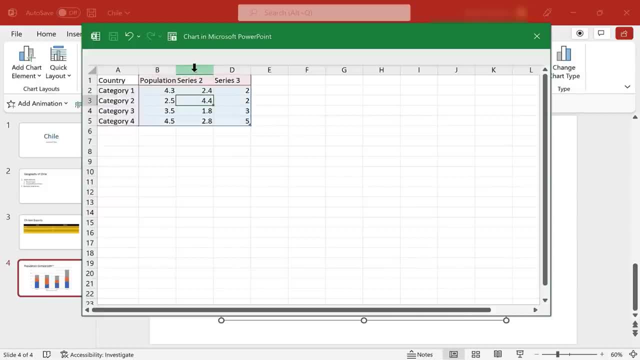 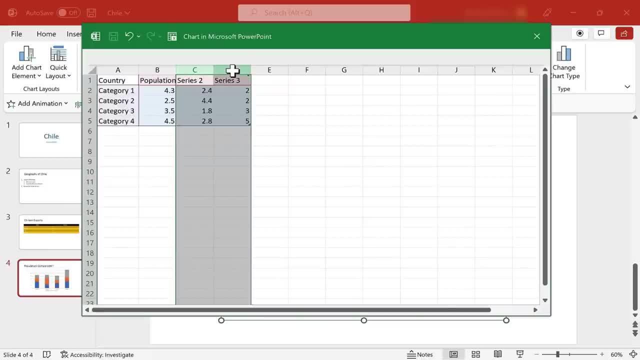 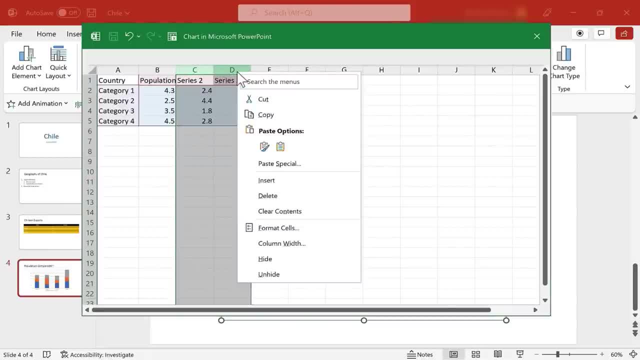 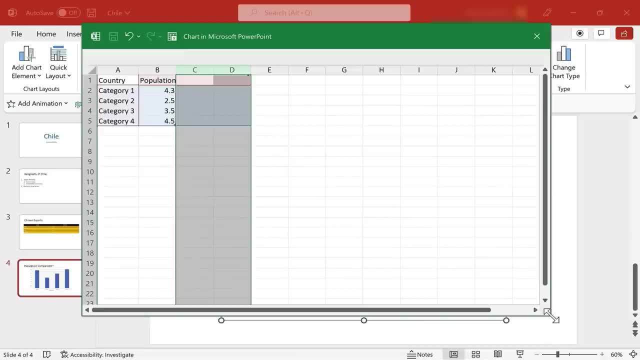 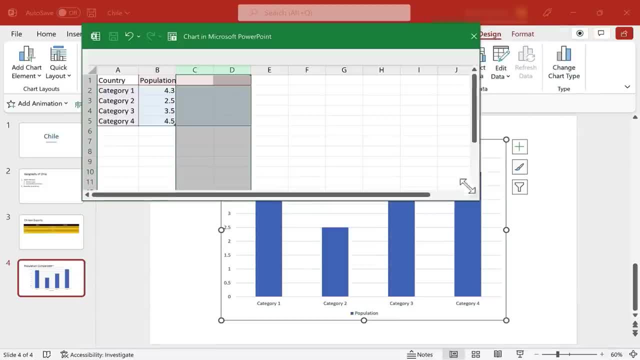 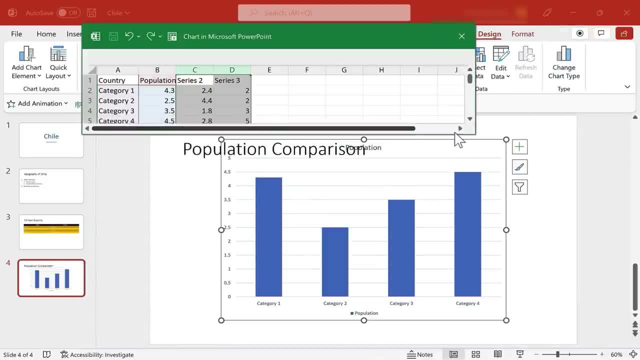 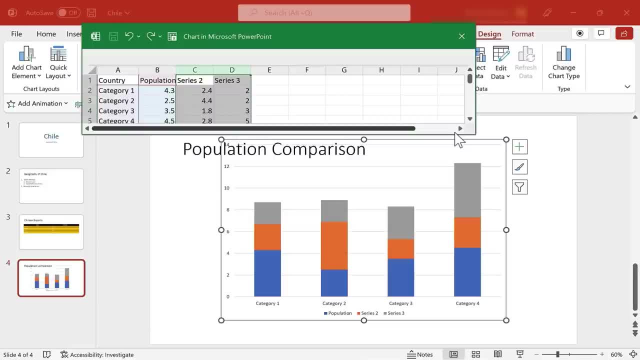 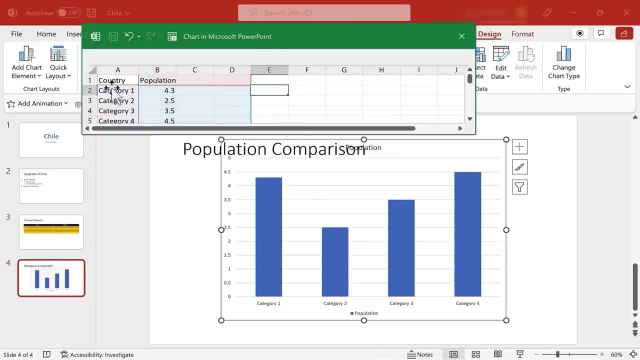 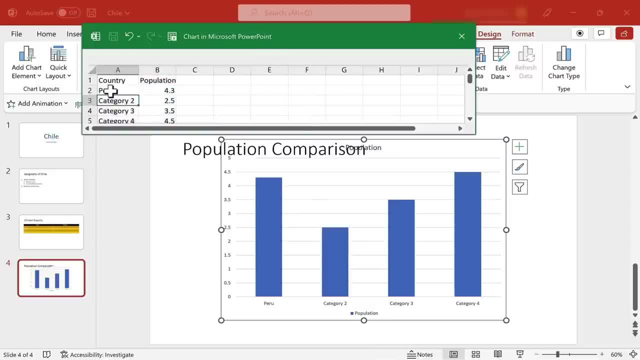 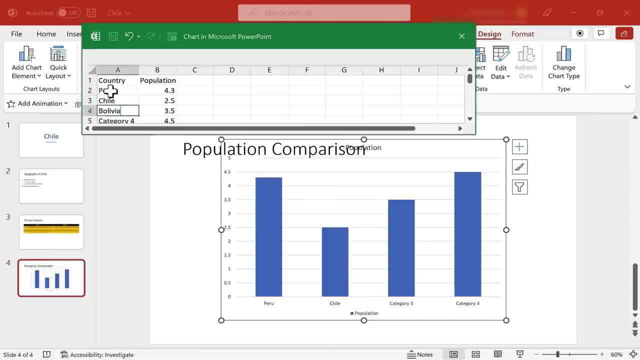 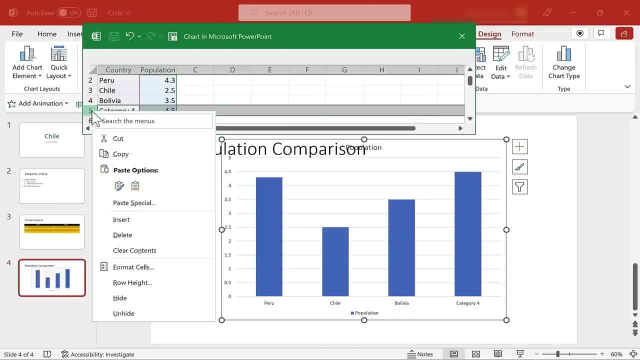 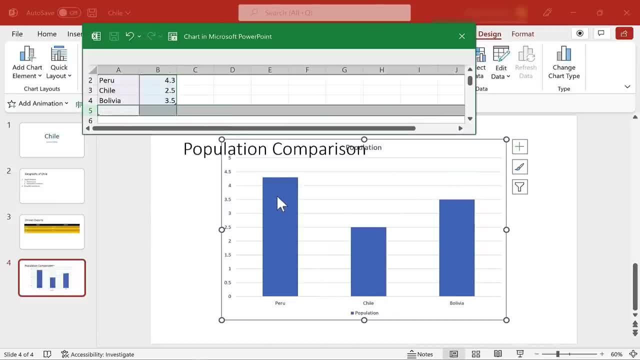 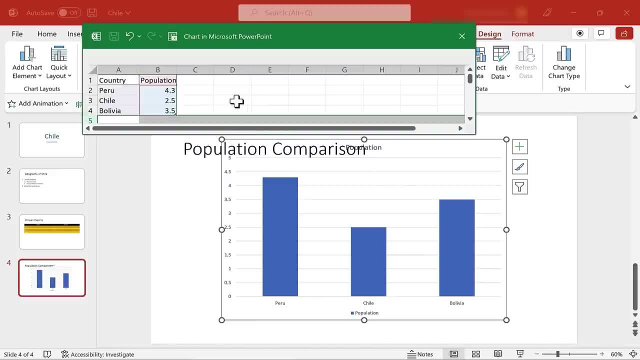 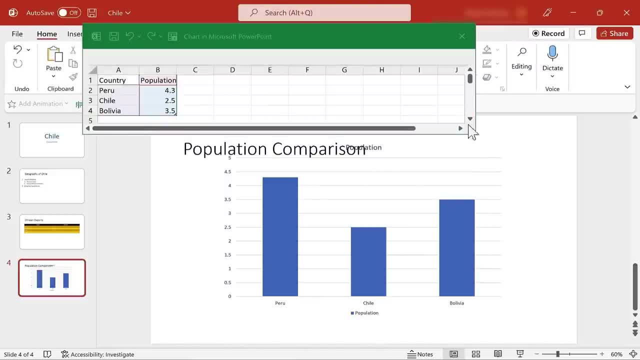 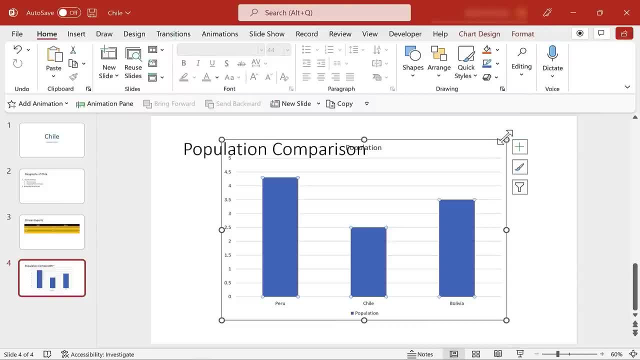 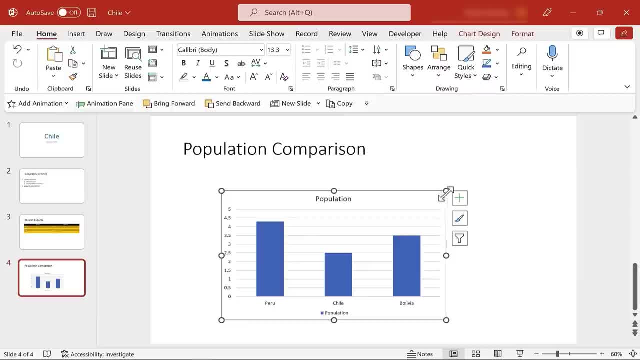 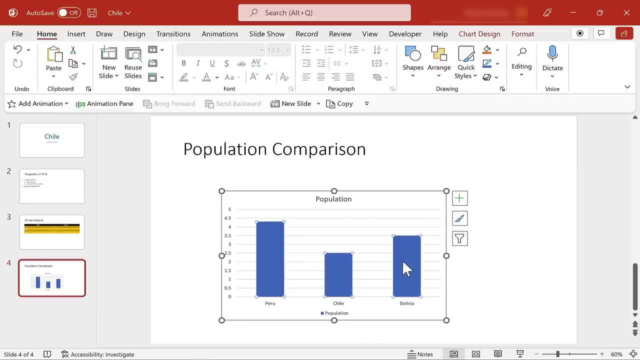 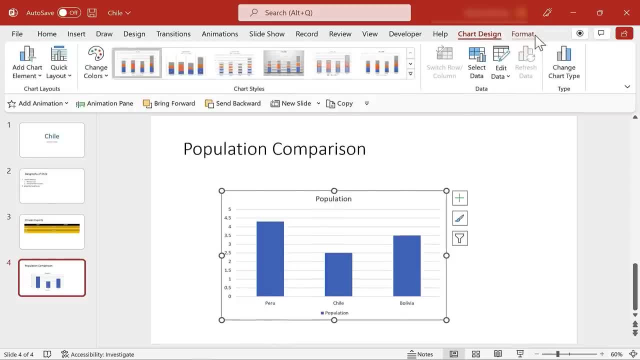 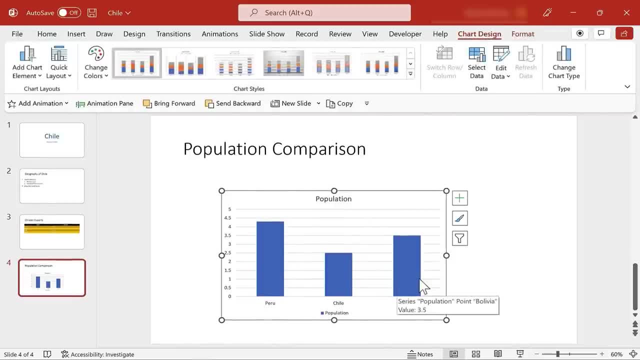 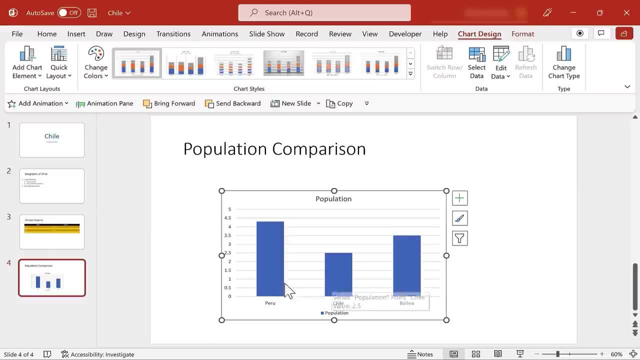 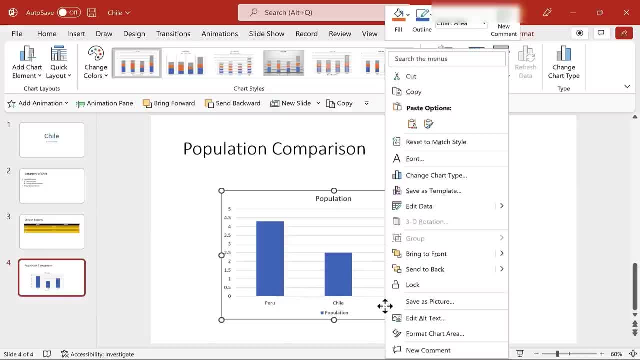 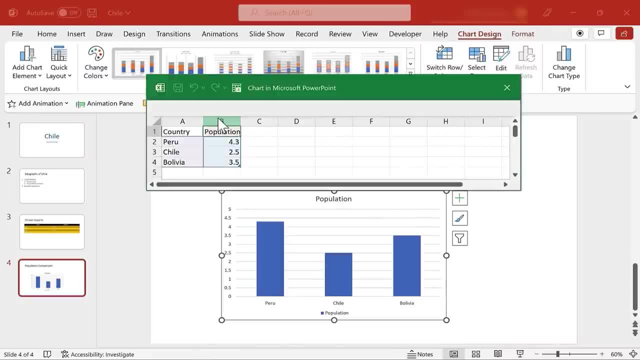 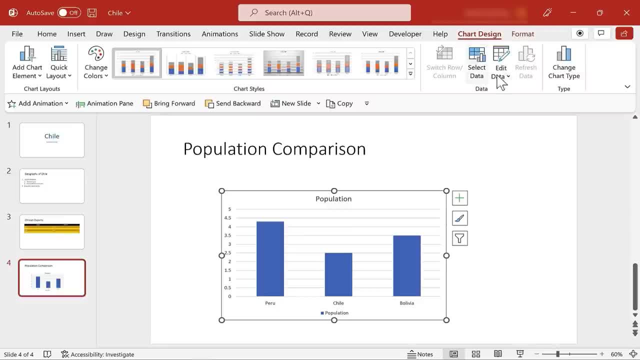 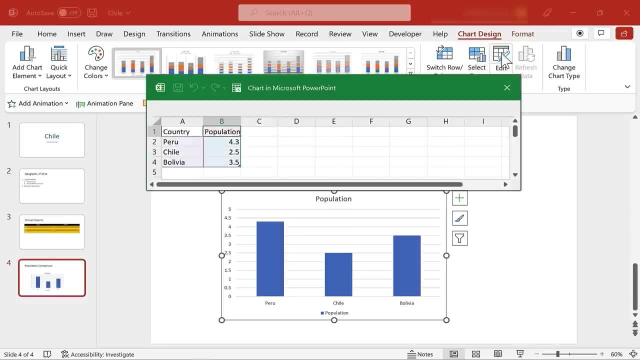 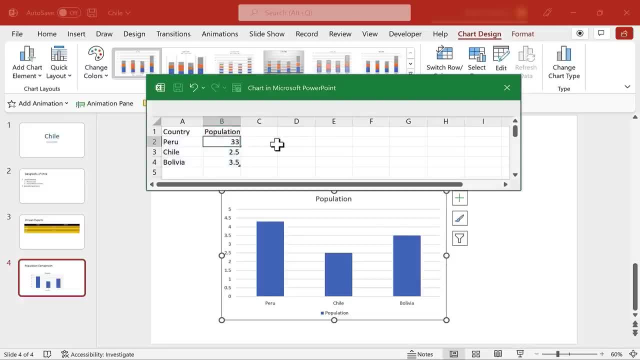 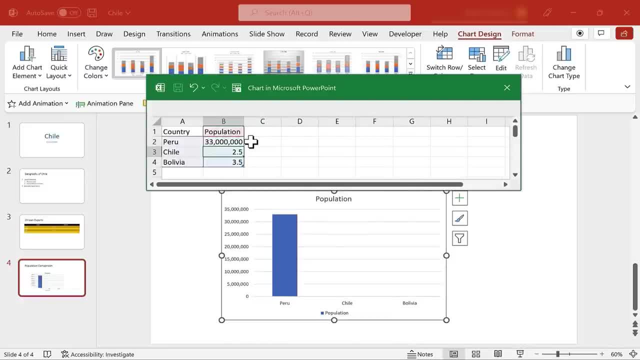 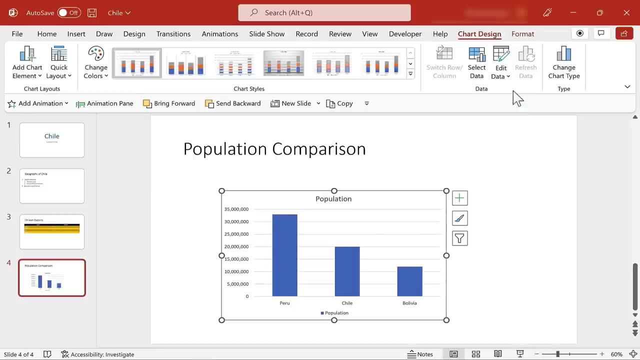 of Peru approximately. Tap enter. Notice that my chart reacted to that change. and now I can put in the population for Chile. Tap enter Again. my chart reacts to the new information. and also I can put in Bolivia's population. Tap enter. Now I can close the Excel window and get back to working. 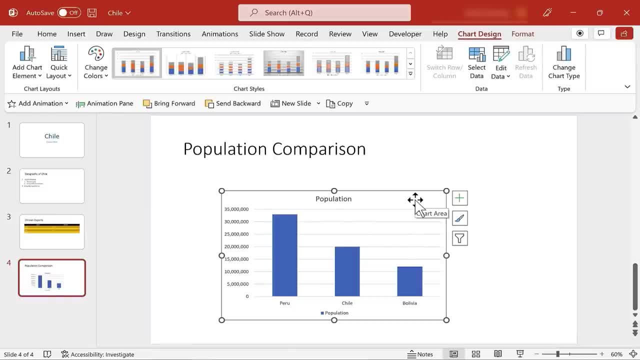 on the look and feel of my chart. Let's just look at a few of the chart options that we have Here. on the chart design tab we can add chart elements and you can see all of the different options that you have there. There are also some quick layout options that you could try. You can see a preview. 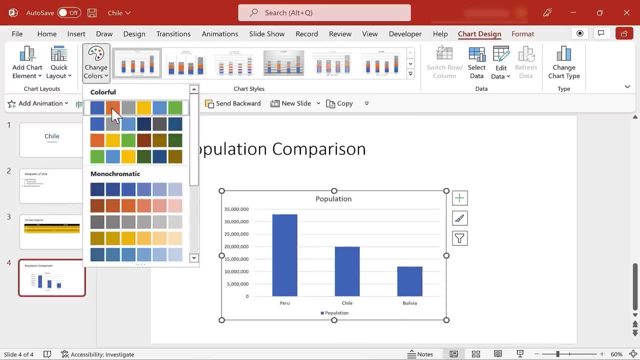 of what they'd look like. as you mouse over them, You could change the color scheme of your chart and again you get a preview without clicking. There are also chart styles that you can browse through, and if you click here, you get even more chart styles. I'm going to go with style 8, so I 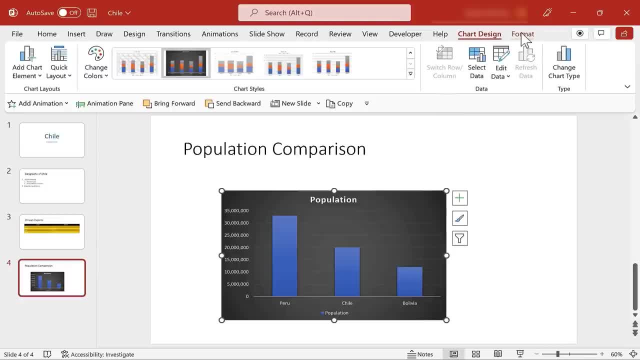 just click. In addition to what I've already shown, we also have style 8.. I'm going to go with style 8.. I'm going to go with style 8.. I'm going to go with style 8.. Some chart format options, including changing the word art styles. So, for example, this the word: 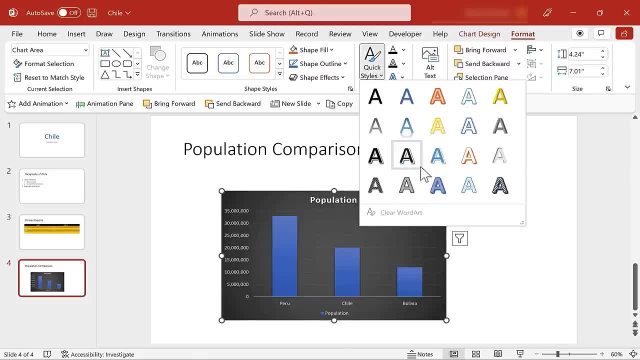 population is a word, art style, and I can change that up by clicking any of these other options. Now, on this same chart format tab, I could annotate this chart. One way to do that would be to insert shapes. So, for example, I'm going to click here on the oval and then I'll click and drag on my chart. 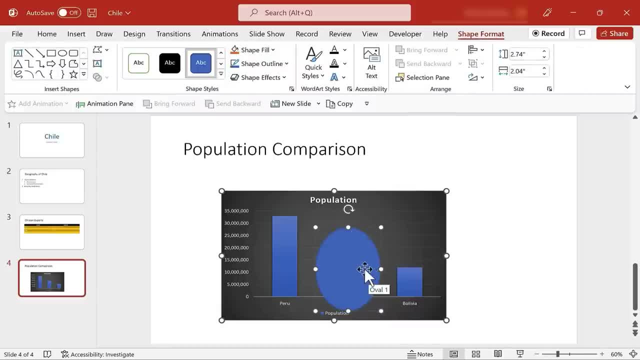 to basically circle Chile. Now that I've added that oval, I can go up here to the shape format tab In the shape styles group. I can change the format and I think I need to change the shape fill. I'll make it no fill. I could change the shape. 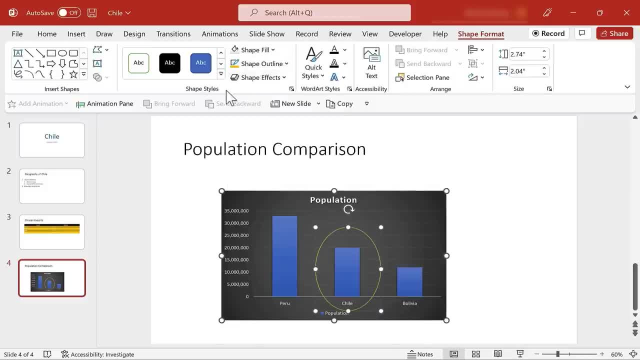 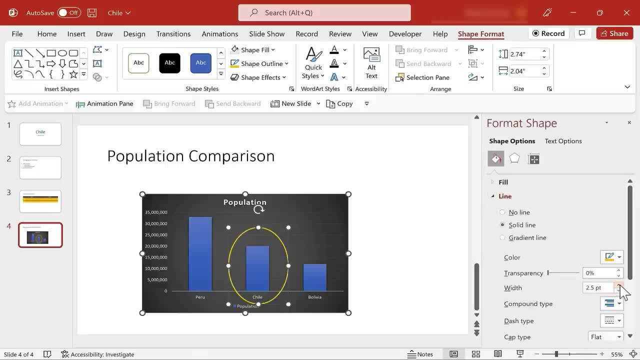 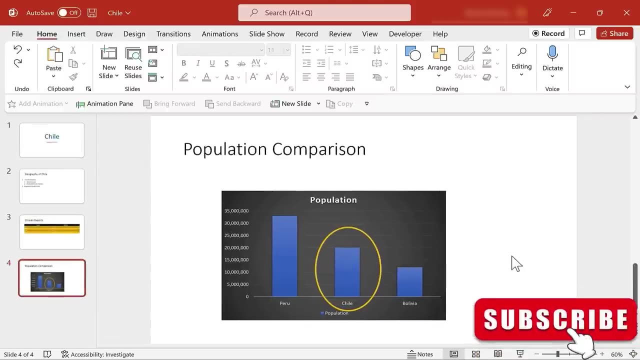 outline to maybe a different color, and if I click the shape styles launch button it gives me even more options, including some line options. I could make the line width much bigger and thicker, So that's a nice way to annotate a chart in PowerPoint. In this segment we've looked at how to. 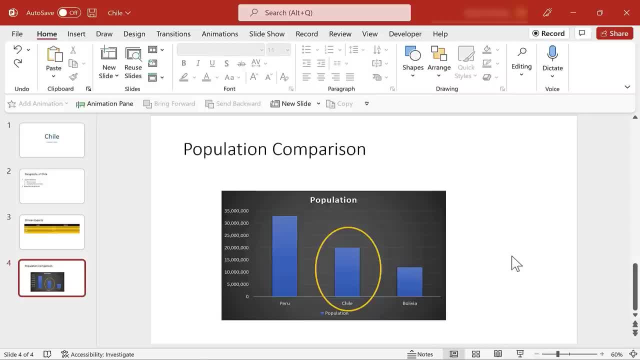 create a simple chart in PowerPoint, how to enter data into the little Excel window that pops up, how to edit that data, how you can choose a chart type, how to modify what the chart looks like and how to do some simple annotations In this next segment of PowerPoint for Beginners. 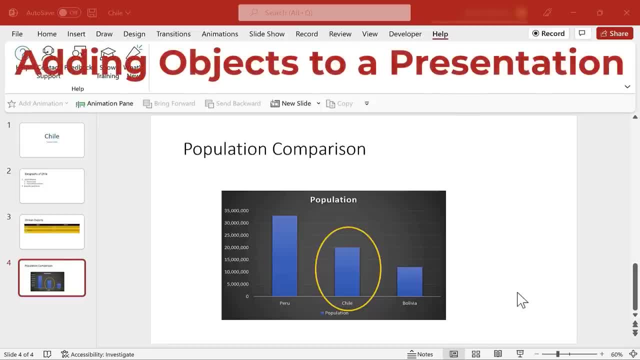 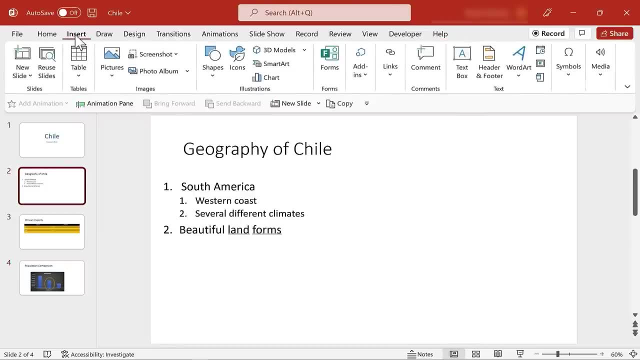 Complete Course. we're going to look at some of the object types that you can add to your presentations, And I'm going to start by clicking here on slide number two and I'll go to the insert tab On the insert ribbon you'll find here in the text. 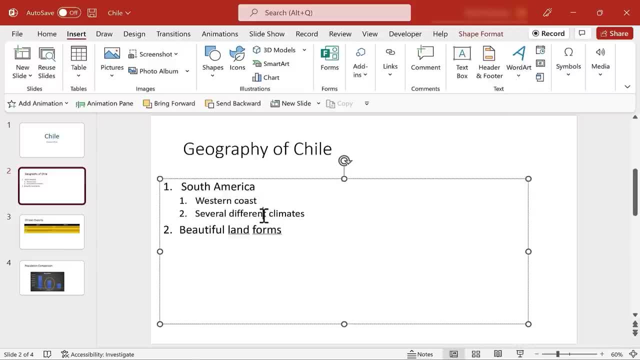 group some options for adding more text. Now we already have a text box with a numbered list. but one of the nice things about PowerPoint is that you can add as many other text items as you want and as you can fit on your slide. But just so you know, it's not a great idea to overburden your 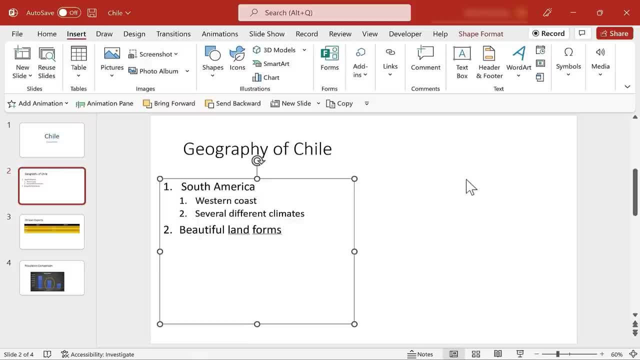 slides with text. If you add too much text, you're going to lose the audience. Having said that, let's add some more text. So here on that, insert ribbon in the text group. let's start with adding word art. If you click there on word art, it gives you different styles to choose from. I'll select this. 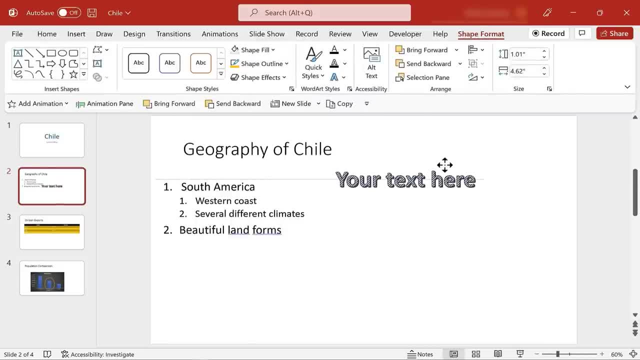 one here and then I get a text box that's added to my slide. But this isn't just regular text, it's word art text. I could now triple click on that text to highlight it, and then I can type to put in the words that I want. Now, if I highlight my word art, notice that I get a pop-up here with 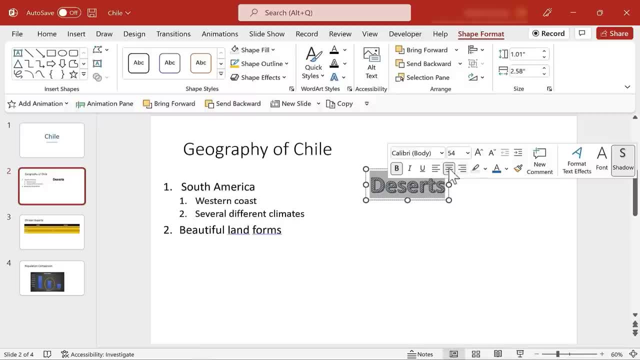 some of the common font options in PowerPoint. So this is another way to do things like bold or bold your text, change the font type, the font color, the font size Anytime. you see that handy pop-up, it's kind of a shortcut Using. that is often faster than going here to the home tab. 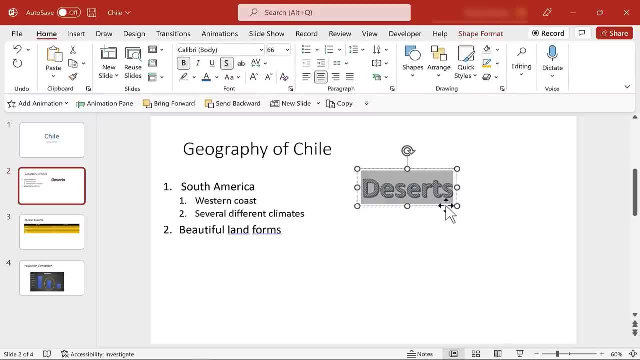 and using the font group. Now I can go to the very edge of the text box and I can click and drag to put it where I want it to be on my slide. Now, one of the nice things about having more than one text box is you can overlap them. You can work with each text box separately from the others. 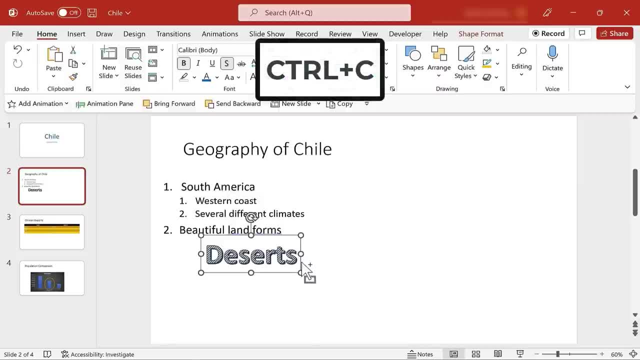 I'm going to click on the edge of that text box, hold control and tap C to copy that, and then I'll hold control and tap V to paste and I'll just move this over here and maybe I'll double click on that word and type in. 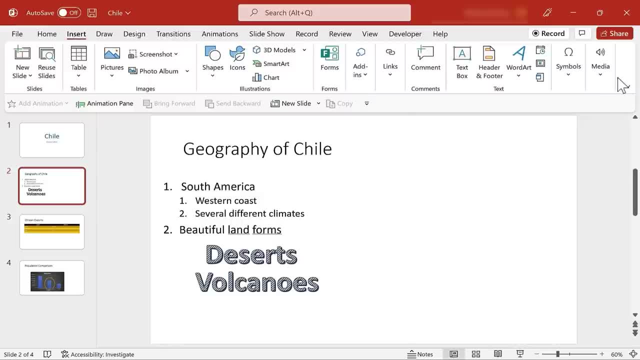 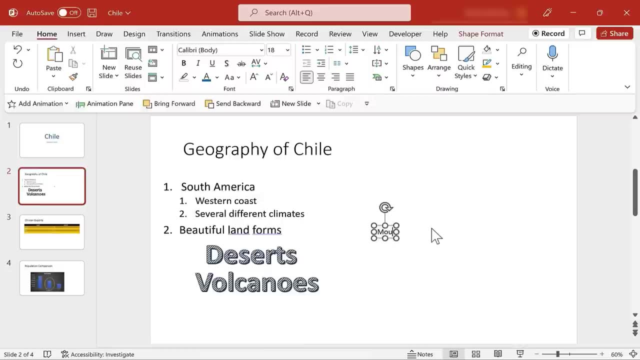 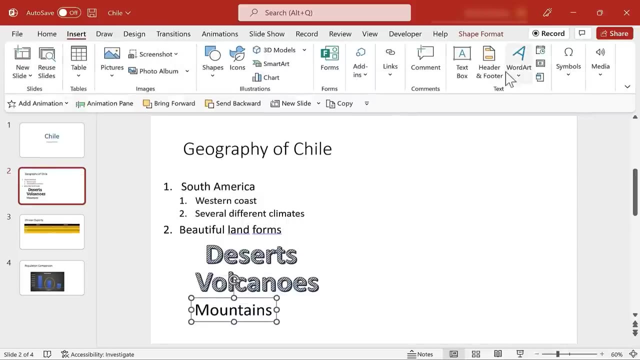 the word volcanoes. Now, in addition to inserting word art, you can also insert just a regular text box. I can now click anywhere in my slide and I can type. So that's another type of text box that you can add into your slides. Now, in addition to inserting different types of text, I can also 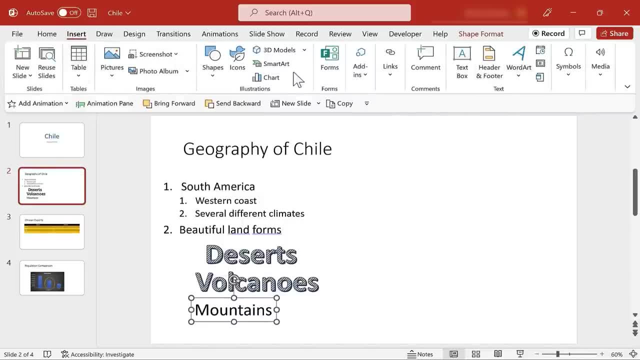 insert pictures. Here on the insert ribbon in the images group, we have a pictures button. When you click that, you need to specify where the picture is coming from. Is it on this device or do I want to access stock images? Now, some versions of PowerPoint don't have access to this stock images. 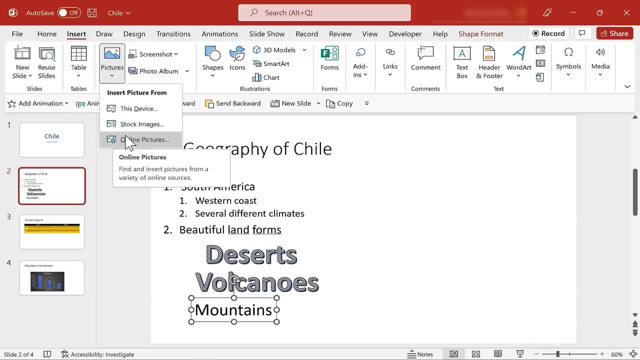 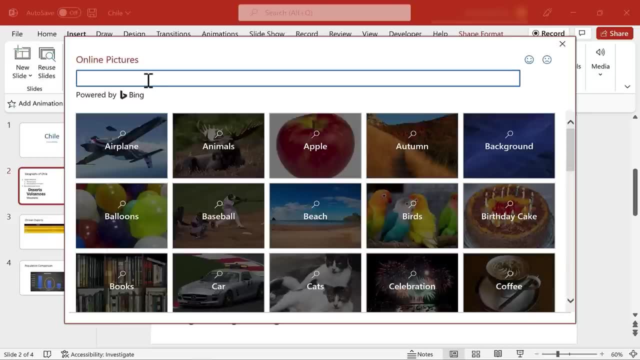 option, but you probably do have online pictures, So let's start with online pictures. When I click that, PowerPoint accesses the Bing image search and you can search for the images that you want to search right here from within PowerPoint for an image to use in your presentation. So I'm going to 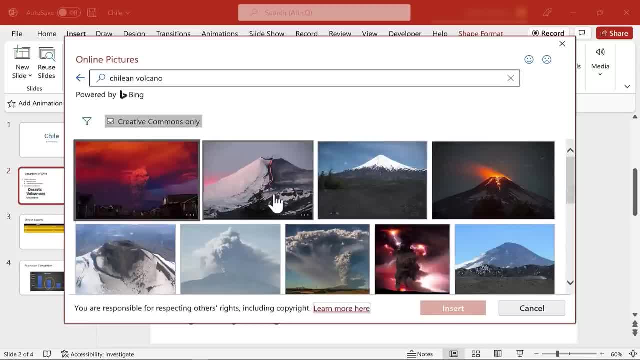 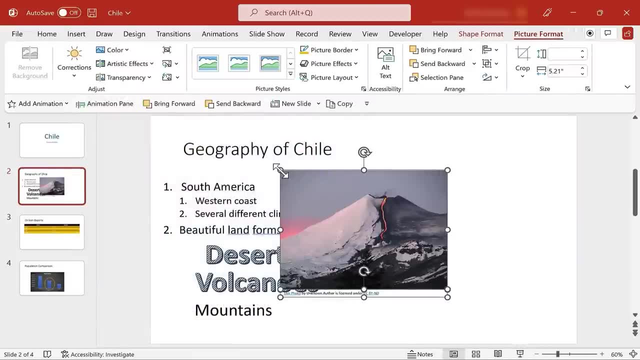 search for Chilean volcano and it brings up some great options and I can click to insert the volcano, in this case, that I want to add to my presentation. Once I have that on the slide, I can click on any of the corners and drag to resize the image and put it where I want it to be. Let's look at some. 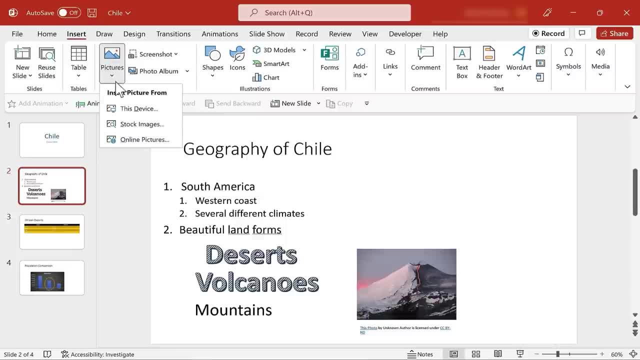 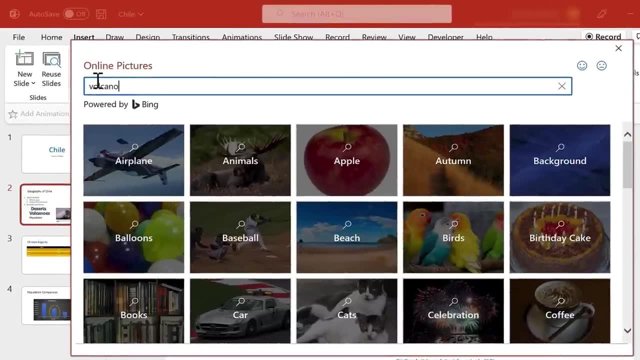 other pictures. options- Insert pictures. I'm going to add another online picture, but this time I want to show you a trick. If I do a search for volcano and then add PNG to the end of that and tap enter, it's going to search for. 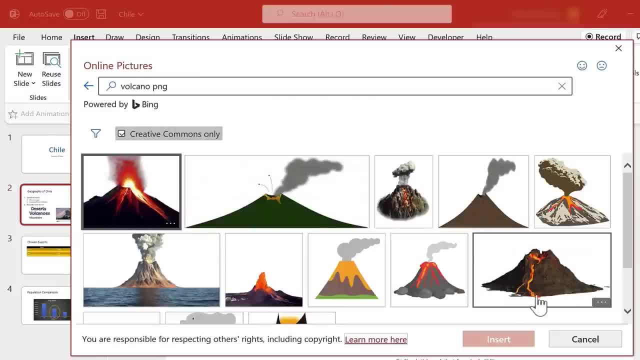 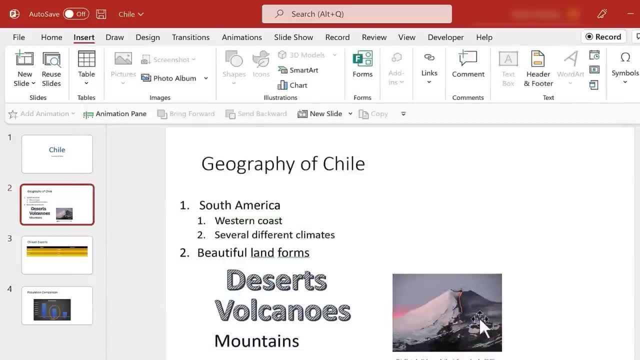 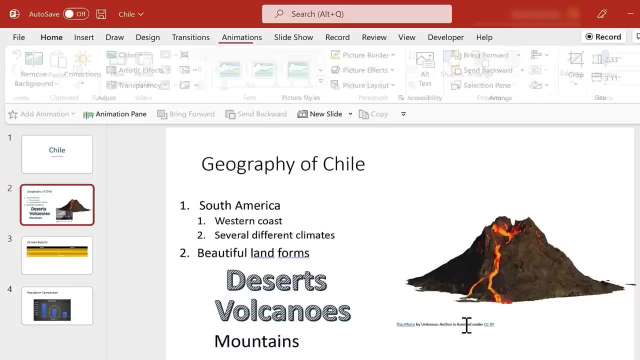 volcanoes that tend to not have the rectangular backgrounds. So, for example, this one should have a transparent background behind the volcano. So if I select it and click insert now look what I get. I get a volcano, just the volcano, no background or anything else. So if I wanted to, I could delete. 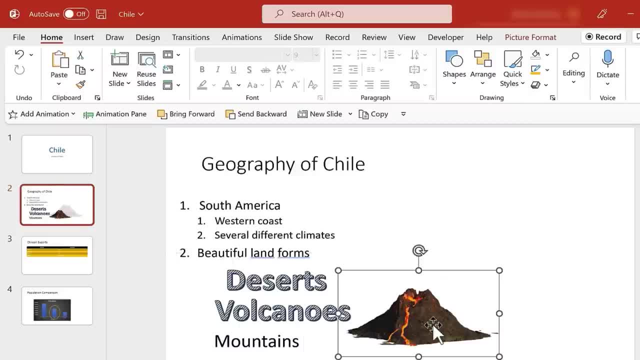 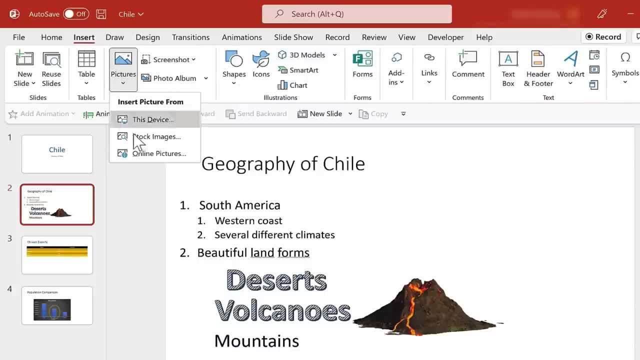 the other volcano and just use this one. So that's a trick to try Adding PNG to your image searches. It doesn't work every time, but it often does. Let's insert a different kind of picture this time. How about stock images? When I select stock images, it lets: 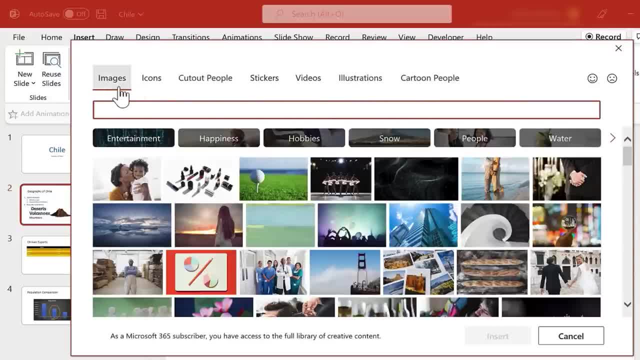 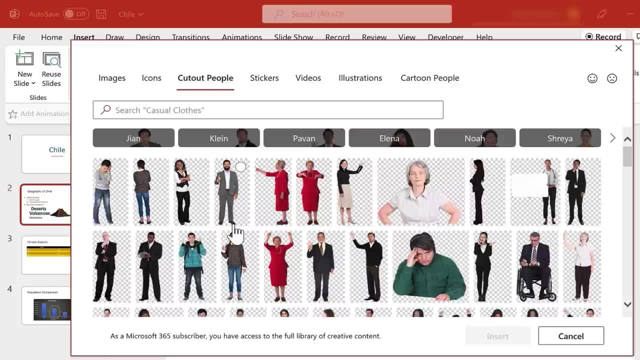 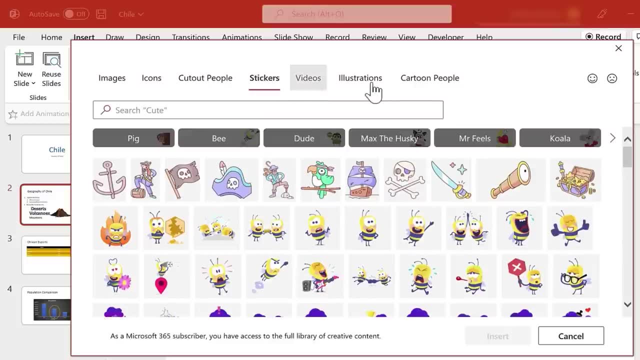 me search for all of these different kinds of images: Generic images, icons, cut out people, which are very useful in PowerPoint. You can have people pointing at different parts of your PowerPoint, People showing different expressions. We also have stickers, videos that you can add. 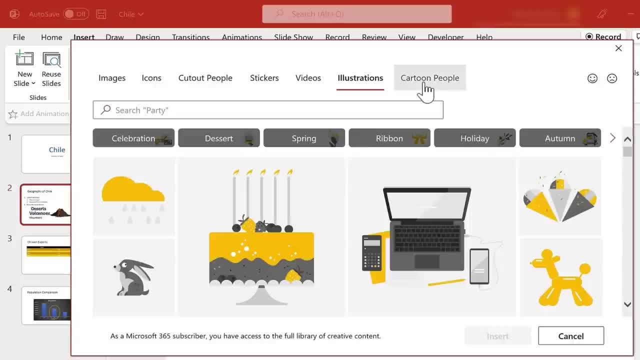 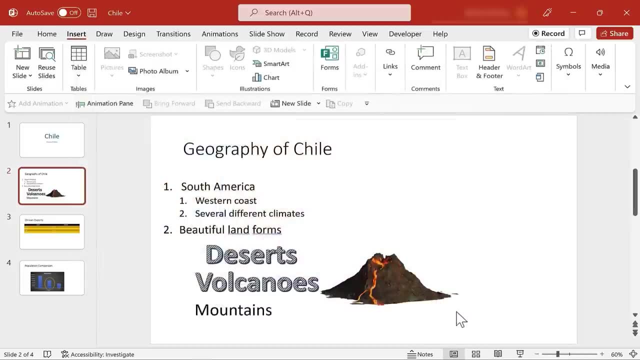 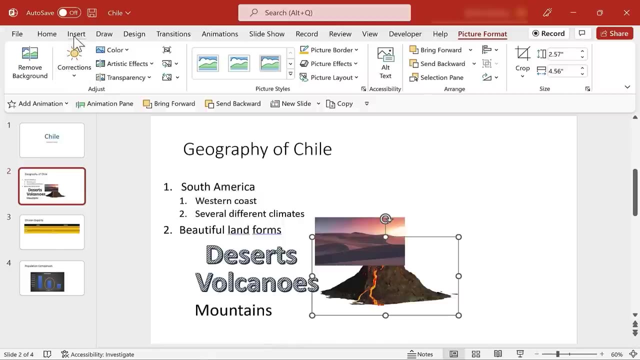 Just short little clips, illustrations and cartoon people. I'm going to go back to images and I'll search the word desert. I'll select this one and insert it into my presentation slide. It comes in way too big but fortunately I can resize that down. It is also possible to insert pictures from your computer. 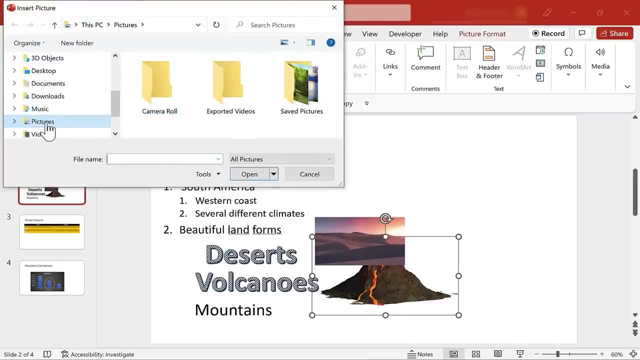 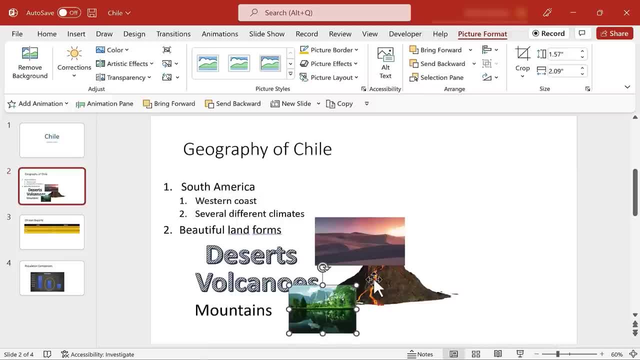 the faster way, and then I could resize that down. Now, if you're adding multiple items like this onto your slide in PowerPoint, there will be times when you want to reorder what is on top of what. So, for example, this volcano is covered partially by the picture of the desert. To fix this, 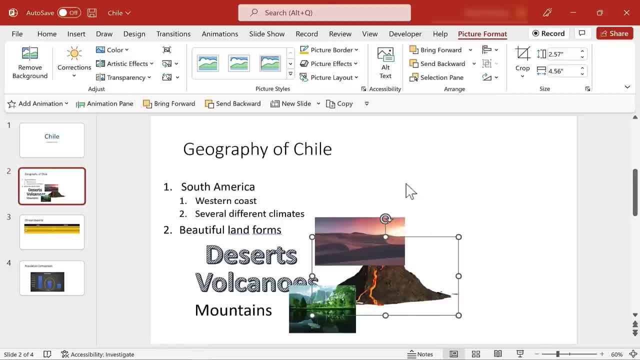 all I have to do is click on the picture of the volcano and then go to the picture format tab that will appear once you've selected the picture, and then I can click bring forward, and that changes the order in which these pictures appear on the slide. a couple of other things i can do with the. 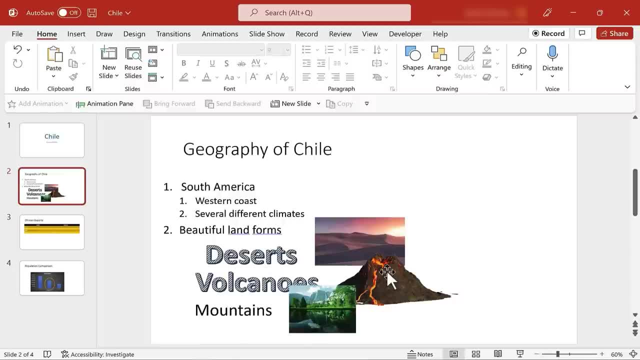 word art, the text boxes and my images is i can click on them and then use this circular arrow to change the direction or the angle of the item. and again i could do the same thing with my text. maybe i could make volcanoes tilt to the right a little bit and mountains to the left, and i think 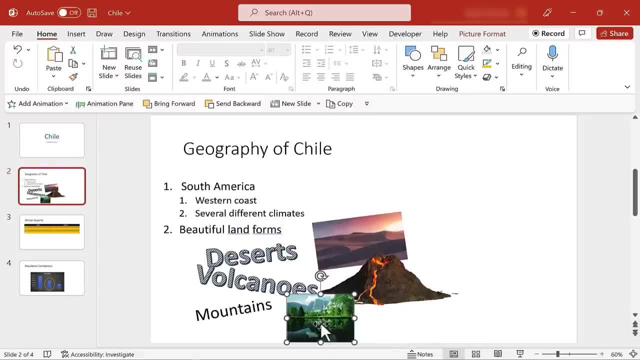 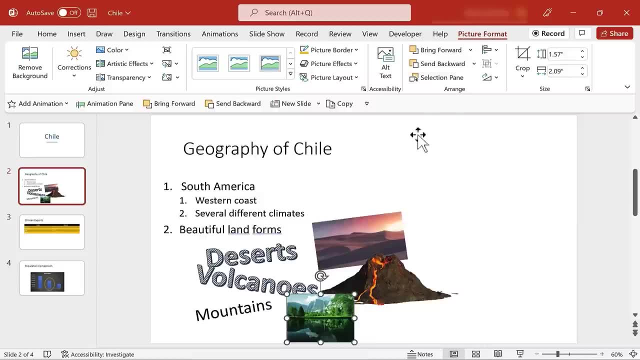 i need to play with this to make it look a little better. i'm also going to move this picture behind the word volcanoes. another way to bring things forward and send them back, instead of using the picture format tab, is to just right click on an item and choose send to back or bring forward. 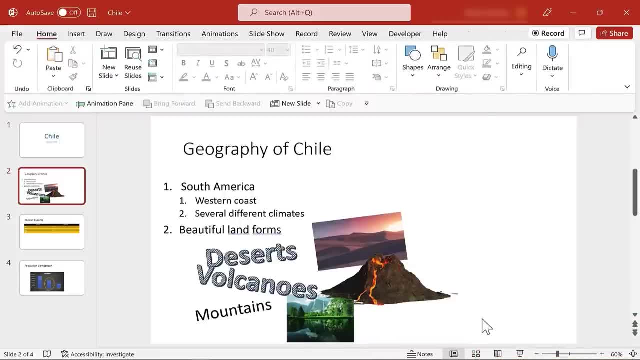 so in this segment, we've learned how to insert word art, additional text boxes, pictures from various sources and how to change the angle of the things that we add onto our slides. in this next segment of powerpoint for beginners- complete course- we're going to look at how to create drawn 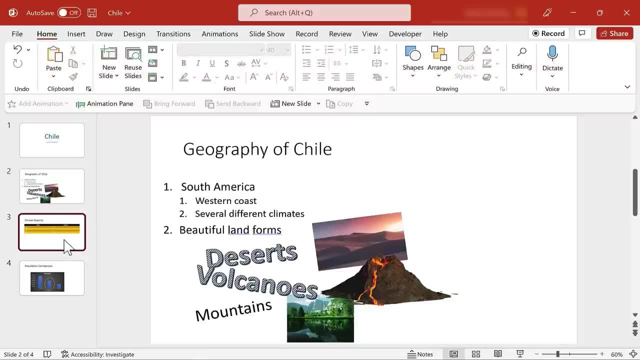 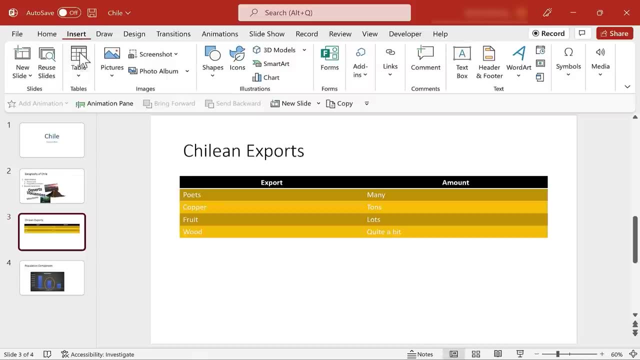 objects in powerpoint and i'm going to click here on the slide 3 thumbnail and once again, i'm going to go to the insert tab. whenever i use powerpoint, i find myself using the insert tab and ribbon very frequently because there are so many different great objects that i can add to my slides using 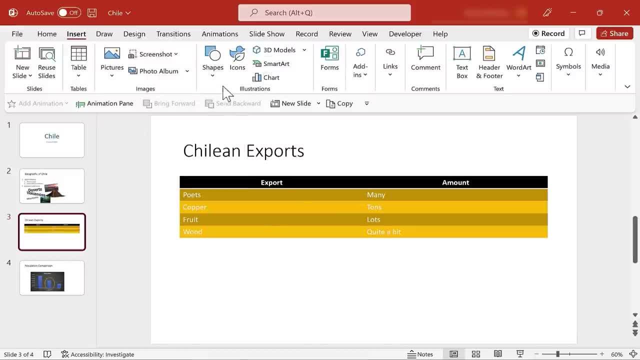 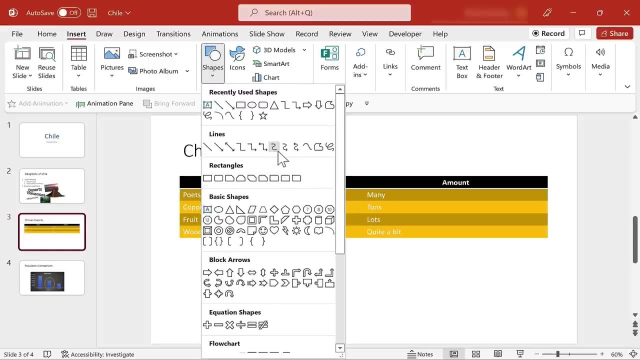 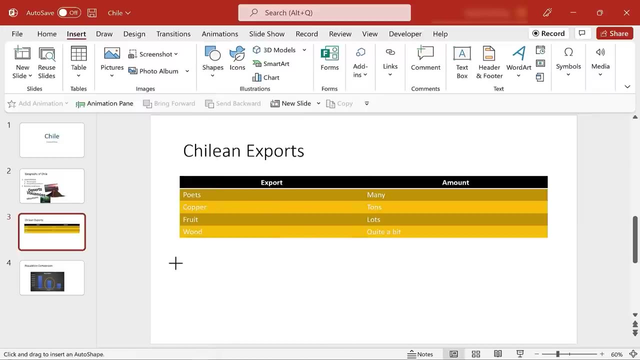 that ribbon. for example, here in the illustrations group i can select shapes and i can choose from a huge selection of different kinds of shapes. some of the most commonly used shapes in powerpoint are arrows and lines, so i'll click here on line and i could click and drag across my slide to. 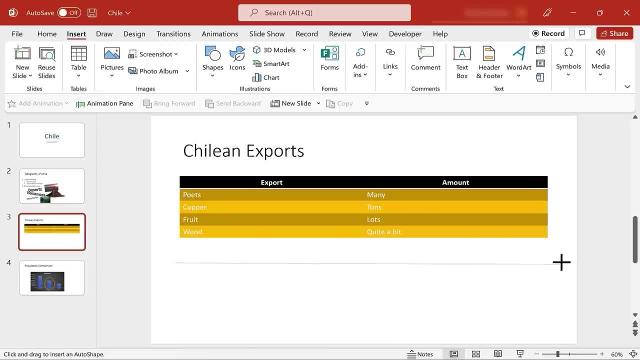 insert a line to separate content that's above from the content that's below. now, if you're struggling, like i am, to insert the line completely horizontally across this slide, there is a trick that you can use. if you hold the shift key, notice that the line snaps into place in a perfectly 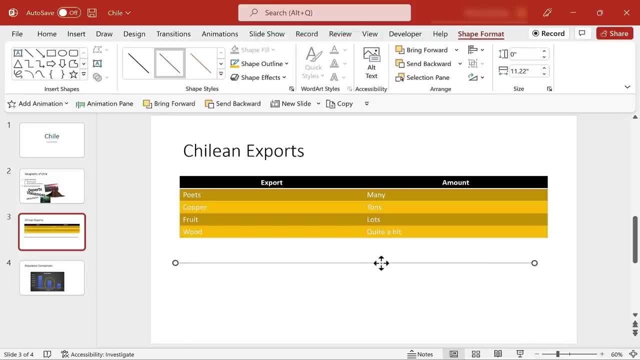 horizontal line. now that i've added a shape and it's selected- notice that i just want to make sure that i have a shape format tab- right from that tab- i can add another line if i want to, or another shape. this time i'm going to make a vertical line, i'll just click and drag and again i can hold the. 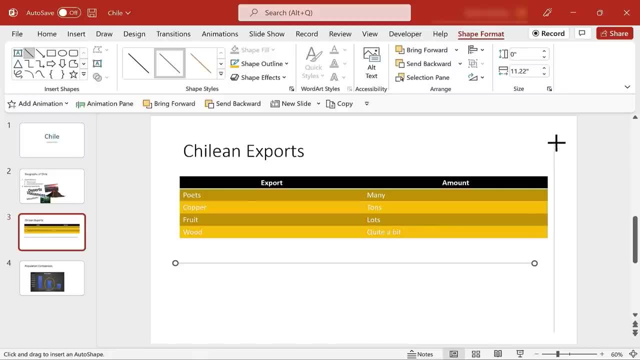 shift key to force it to be perfectly straight vertically. i can also insert arrows. i can just go down here and select arrow, click and drag to insert the arrow and then, if i make sure that the arrow is selected, i can go to the shape format tools and go to shape outline and i could change. 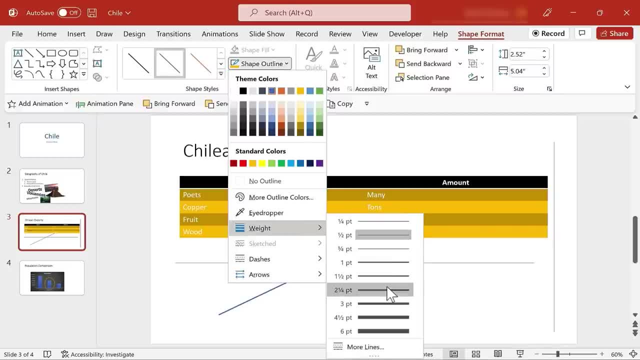 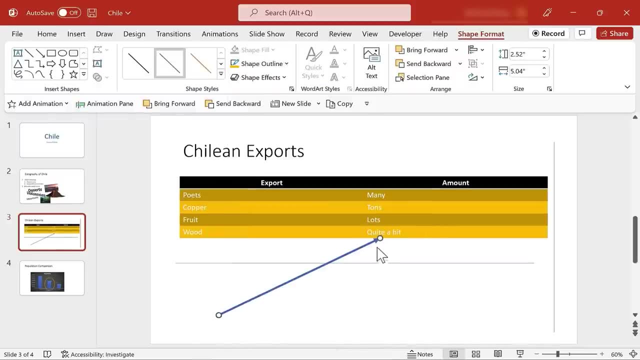 the width of this arrow. i often find that the default line weight is way too thin. i want it to be thicker in most cases, so i'm going to change it to four and a half point and i think that looks a lot better. there are other shape outline options that you can also use. you can change the type of. 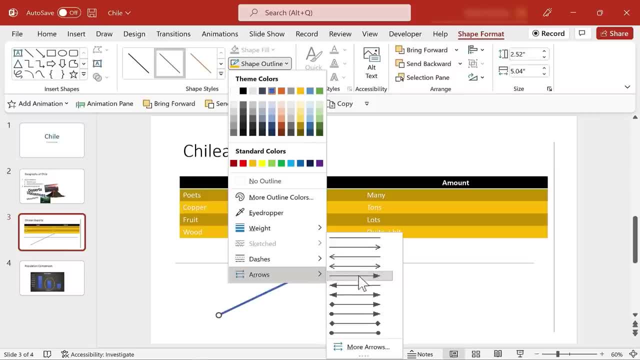 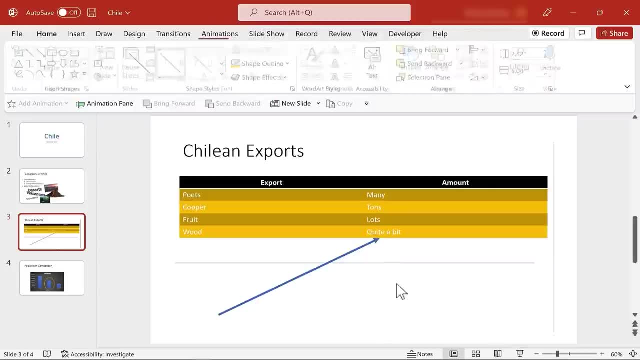 line that the arrow has and you can change the arrow heads, making it a two-sided arrow or any of these other options. i'm going to tap escape to get out of those options because i like the way the arrow is right now. i can also insert other shapes. 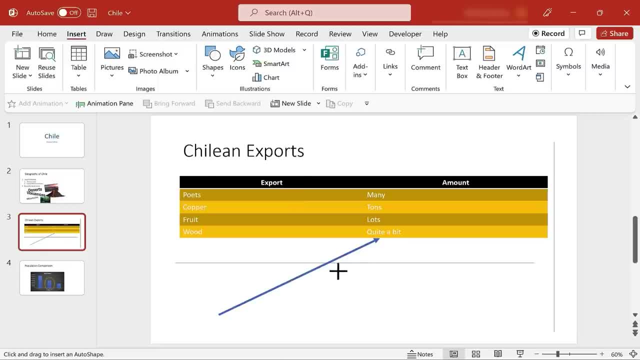 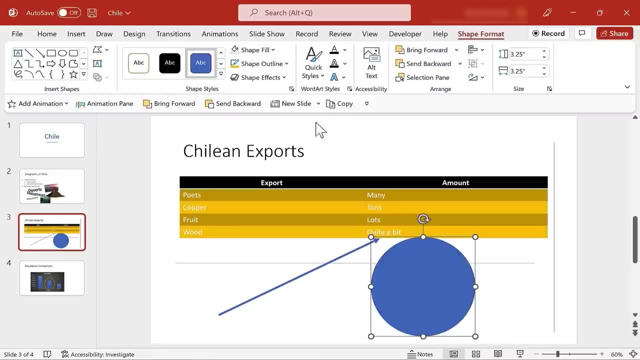 rectangles, ovals, etc. with ovals: if you click and drag, an oval will appear on your slide, but if you hold the shift key it converts it to a perfect circle with all of these different shapes. you can click on the shape and then change the fill color, or you can choose to have no fill at all. 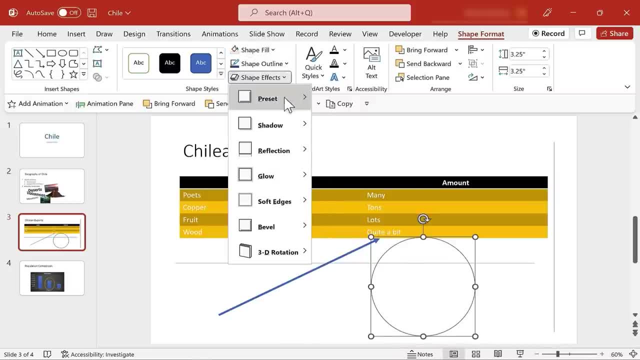 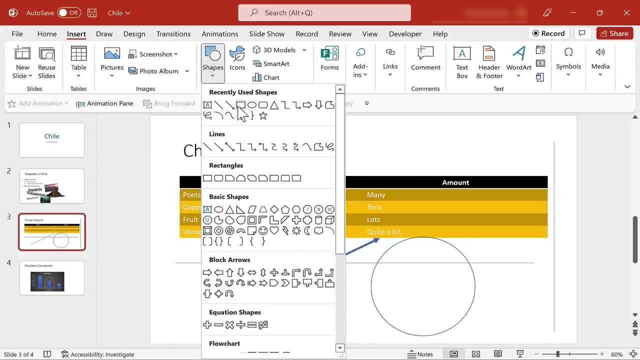 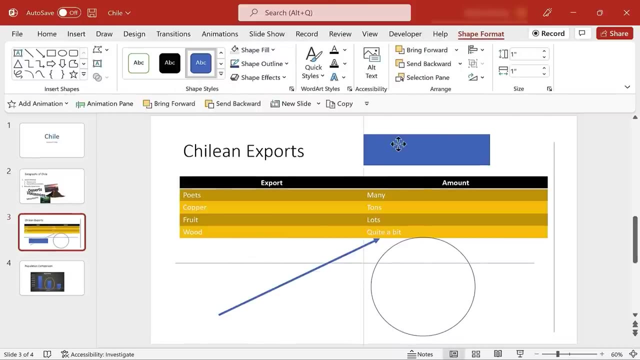 you can also change the outline color, and there are lots of other options that are fun to try. one other option that you should know about: when you insert shapes: you can add some of these shapes and then you can change the size of them and then clicking, or clicking and dragging to place them. 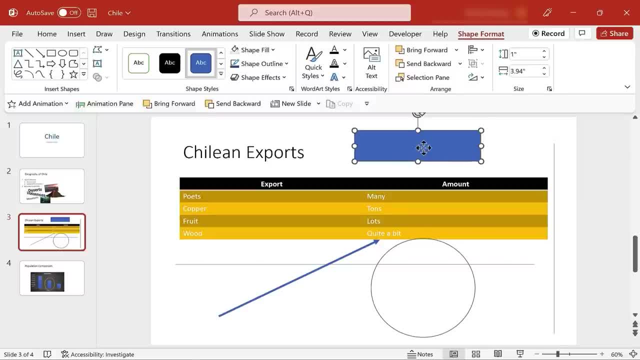 on your slide and then you could resize them as necessary. but then watch what you can do. you can double click on that shape and you get a flashing insertion point or flashing cursor and you can use this basically as a text box, but with color. you can just type in your text. double click on it if 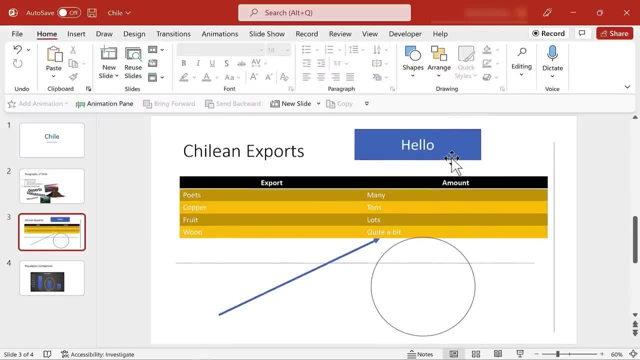 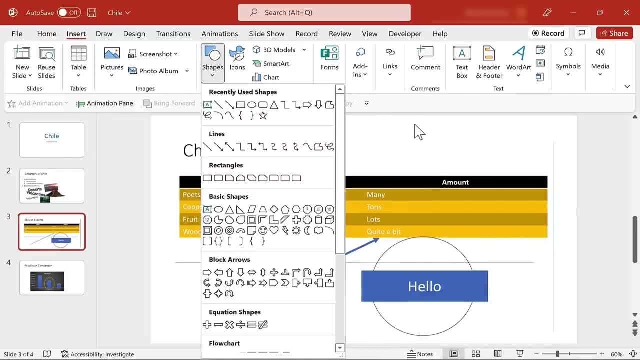 you want to increase the font, etc. this works basically like a text box, so that's a pretty good introduction to the insert shape outline option. so i'm going to go ahead and add a little bit of a preview here as well. we can see that we have a lot of different shapes options that we have in. 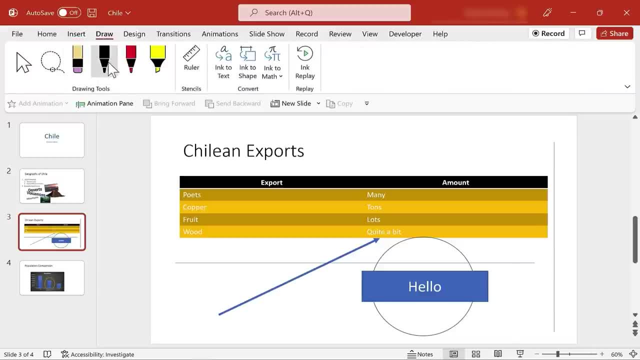 powerpoint. in newer versions of powerpoint we also have a draw tab and some drawing tools and you can click and then simply click and drag on the slide to add a drawing, a doodle, maybe your latest masterpiece. you can click on this arrow here to change the color of the pen, and we do have an 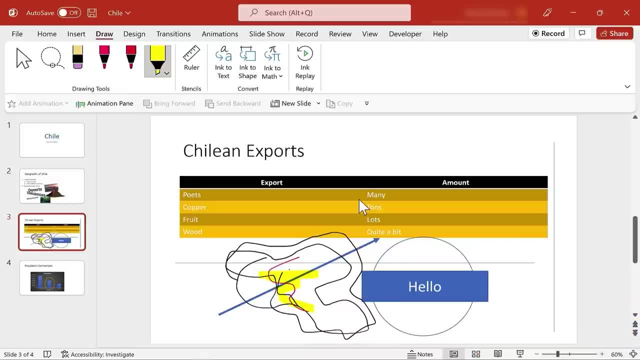 eraser. we have a second pen that we can use and a highlighter. so in this segment of powerpoint for insert shapes, arrows, lines and some drawings, as well as how to use a shape as a text box, In this next segment of PowerPoint for Beginners- Complete Course- we're going to look at a couple 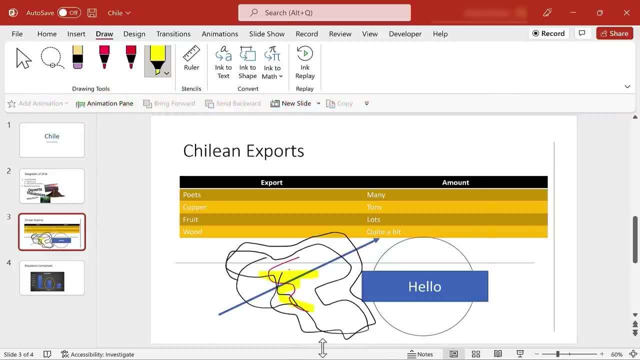 of refinements that we can add to our PowerPoint presentations, And those are how to add a background image to a slide, and also how to add transitions and timing to a presentation, And then we'll finish this segment by looking at how to add themes to your PowerPoint slides. So I'm going to 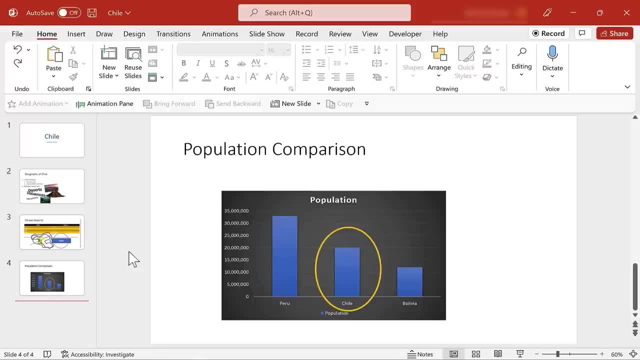 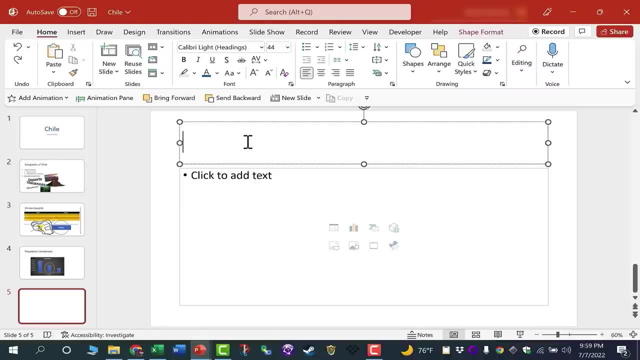 go over here to the left and click below my last slide And I'll go up here to the Home tab and click New Slide And for this I want title and content And I'll click to add title and I'll call this Chilean Food. So that's the title for this slide. Now I could certainly click Insert. 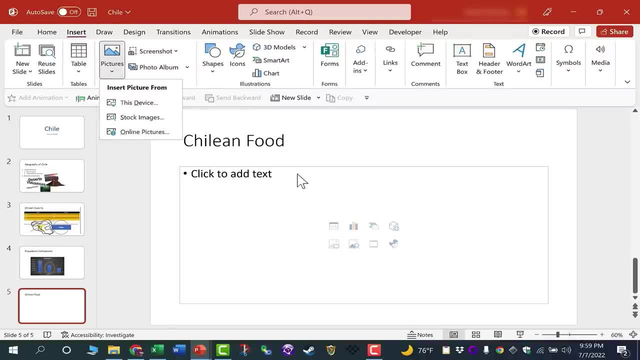 and insert some photos of Chilean food onto this slide. But another way to use images in PowerPoint is to actually add a picture or an image as the background of the slide. To do this you would go to the Design tab and click Add, And then you would see that you have a slide that you want to. 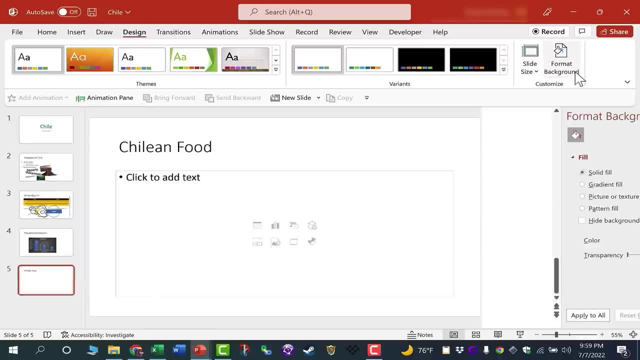 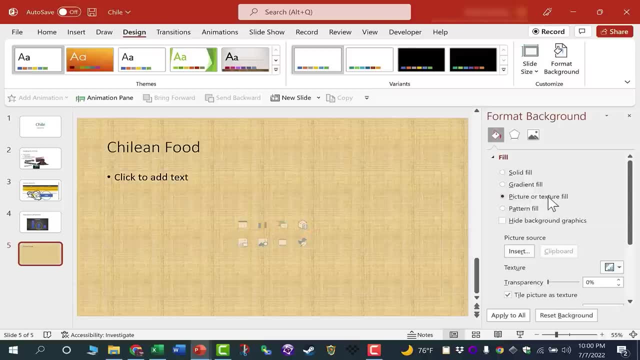 add an image to. So I'm going to go to the Design tab and here at the right just choose Format Background. There are several different format background options that you can choose from, but the one that's relevant right now is Picture or Texture Fill. When I click that, it just adds. 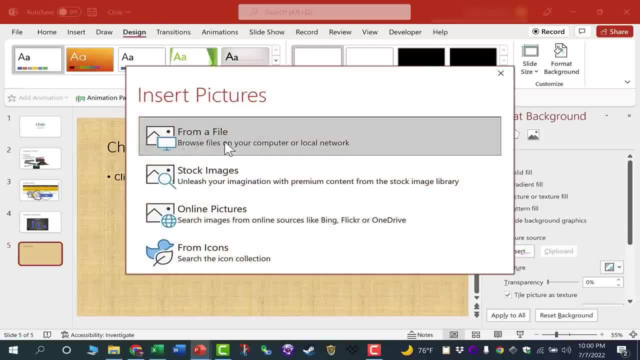 in a texture, But I can click Picture Source and upload an image from my computer And whatever that image is, it will become the background of this slide. I could also access stock images or online pictures, So I'm going to go to Online Pictures and I'll do a search for Chilean Food. 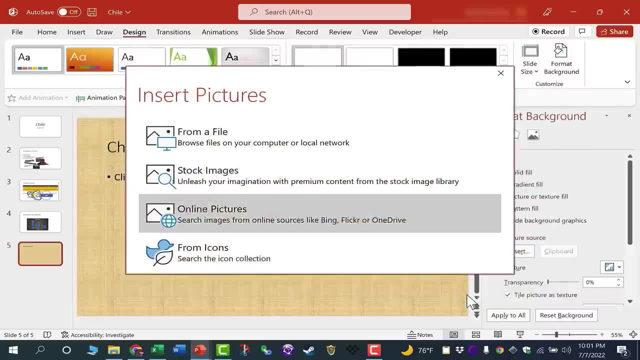 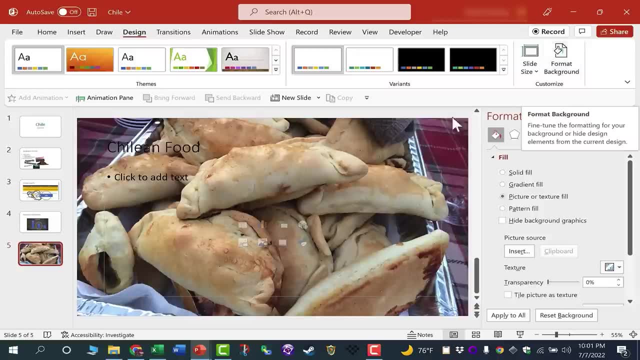 I'm going to select these empanadas and click Insert. And now the empanadas are the slide background. They fill the entire slide. If you decide to do this, you're going to find in many cases it makes it harder to read the text. Fortunately, there's an option that we have here. 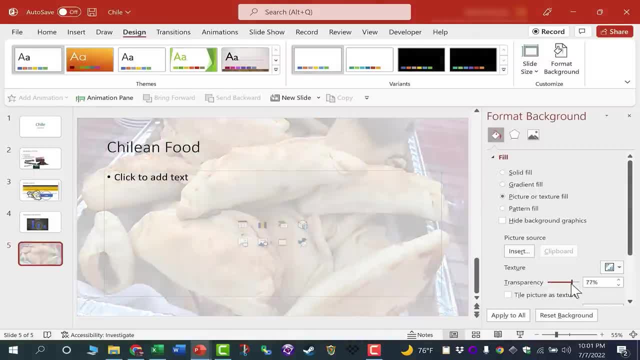 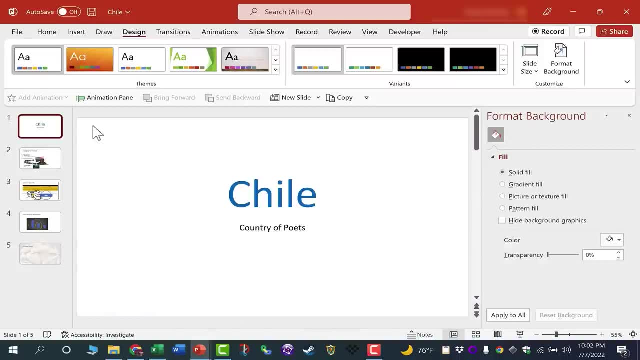 I can change the transparency level of the image to make it much more transparent, So that's a much nicer effect. Another refinement I could make to my PowerPoint presentation is to add some transitions and some timing. If I want to add some transitions, I can just click Add And that's it. 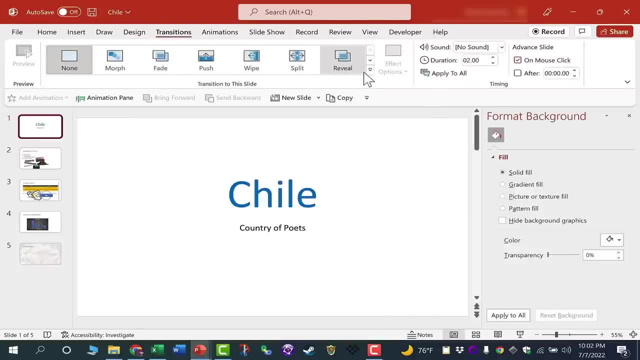 If we go to the Transitions tab, you can see that we can add all of these different types of transitions between slides. I'm going to go with just a simple fade, So that will be the transition to this slide. I'm going to close this Format Background pane by clicking this button here, so 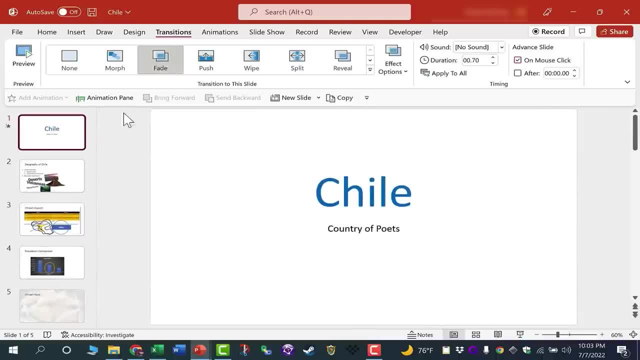 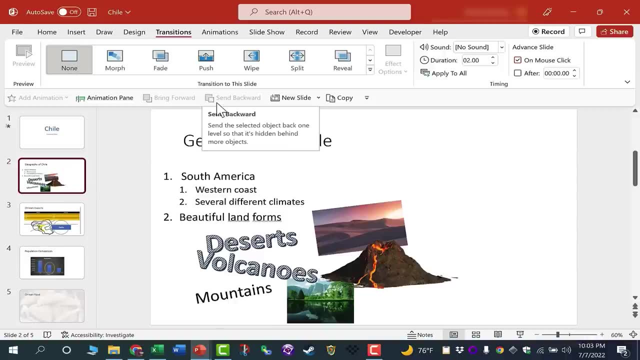 that you can see my slides a little better Now. if I wanted to, I could add a different transition for each of these slides. That's not really recommended. It's a common mistake a lot of new, less experienced PowerPoint users make is that they want to try every single transition that they. 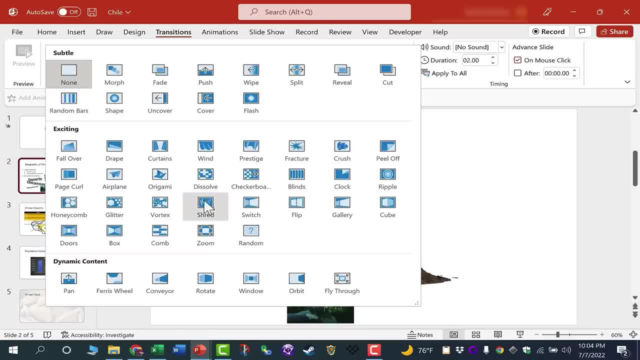 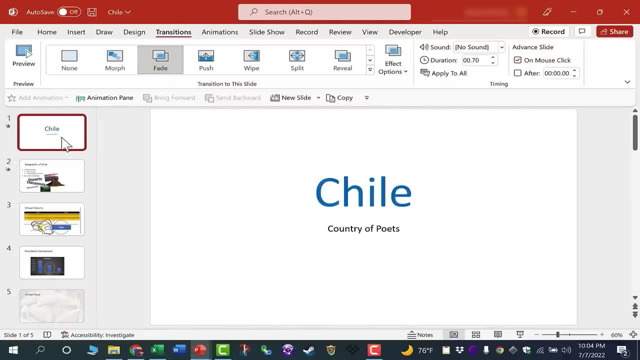 have available. So maybe on slide two I'll click here and I'll choose the Vortex transition. Take a look at that. But adding too many different transitions really distracts the viewer more than anything. Let's take a look at the two transitions and you can decide which is less. 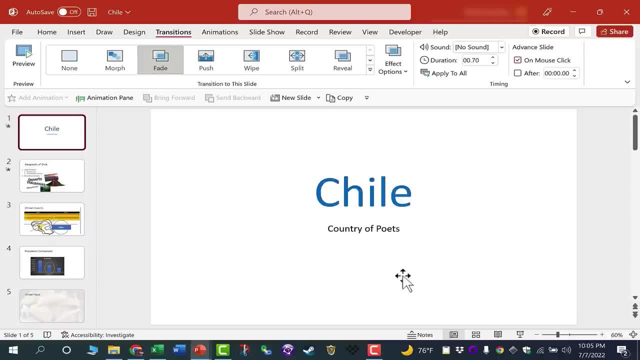 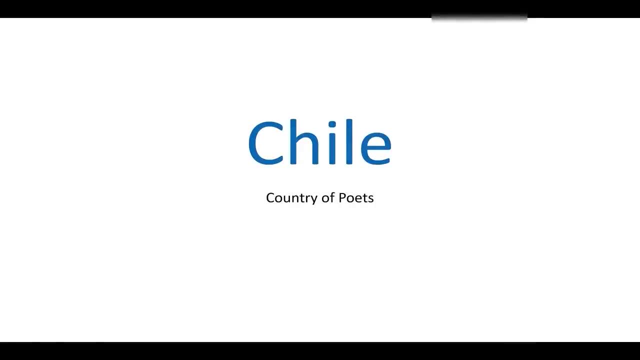 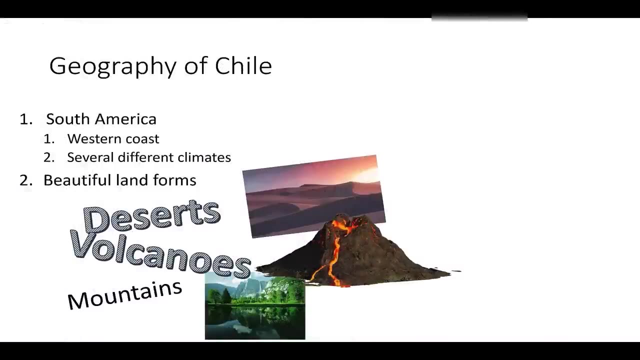 distracting. So I've clicked here on slide number one and then I'll go down here to the lower right corner. I'll click and there's my first slide fading in And then I can click to advance to the next slide and there's my very dramatic Vortex transition. I'm going to tap Escape to exit the. 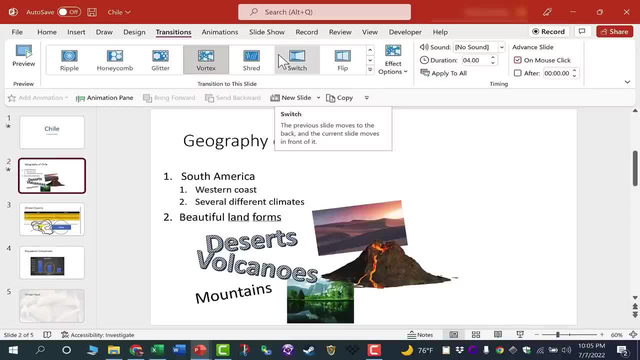 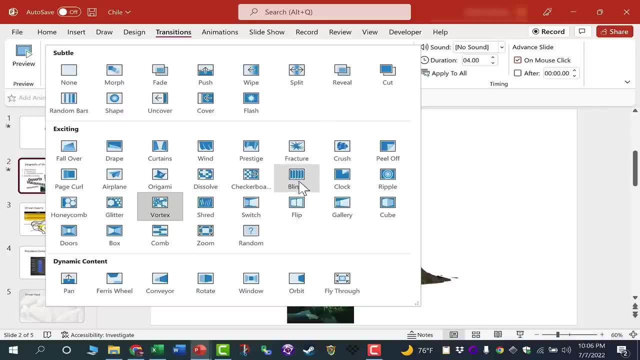 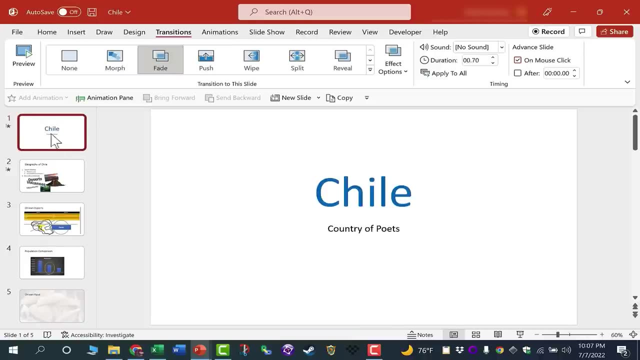 presentation. So have some fun with the transitions, but my advice is use them sparingly, use them judiciously and in many cases, just use the same transition over and over in a particular slideshow. So let's say I want to use the same transition on all of my slides. I'm going to 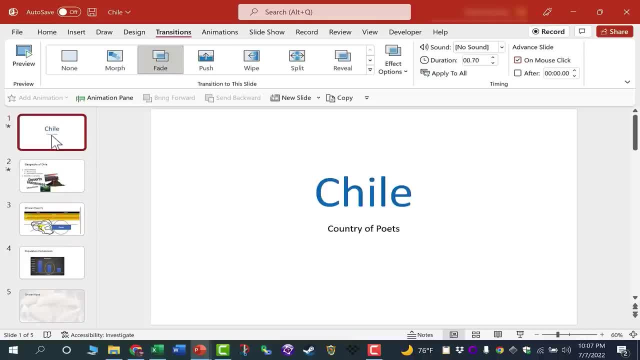 select all of my slides, Instead of adding each one one by one, I could simply add a transition to my first slide and then click this button: Apply to All. Now if you look here at the left, each of my slides has a little star with some lines to the left indicating movement. So now, 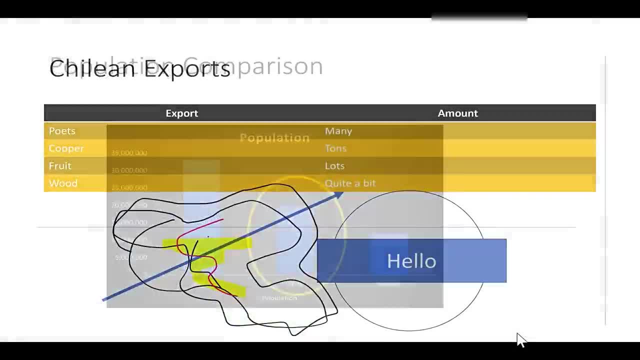 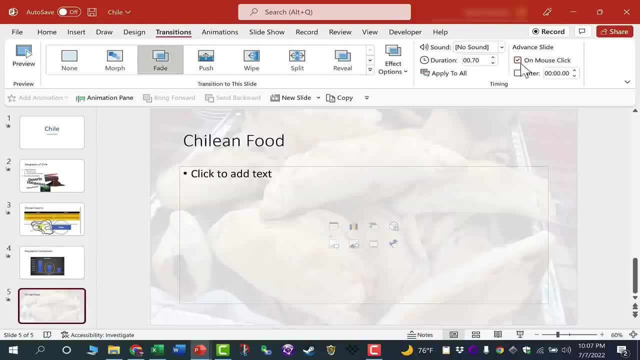 each of my slides should have the same transition effect, a simple fade. Now, another option that we have- that's here on the transitions ribbon- is Advance Slide. By default, the On Mouse Click is selected, and that's good. What that means is any time I want to transition from slide one to. 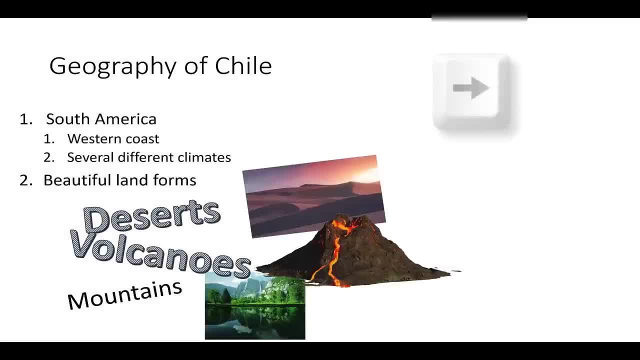 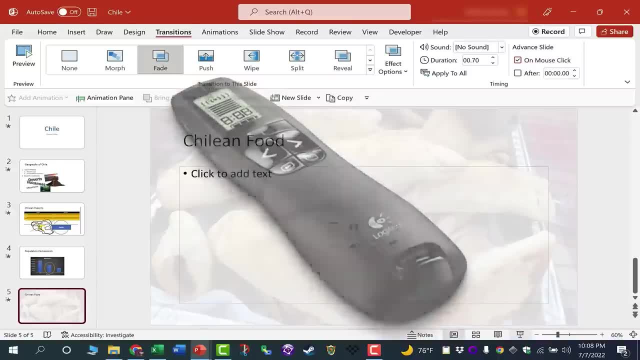 slide two. all I have to do is click the mouse button, Or, if I want to, I can use the right arrow or the space bar. All of those methods, or even a presentation remote, will advance the slides, And I'm going to leave it that way. I think it's a good idea to leave that checked, But if you want you. 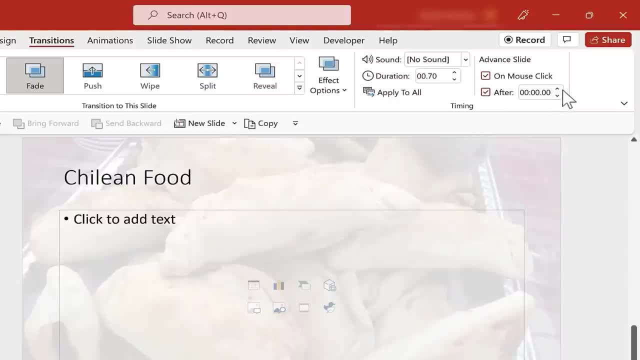 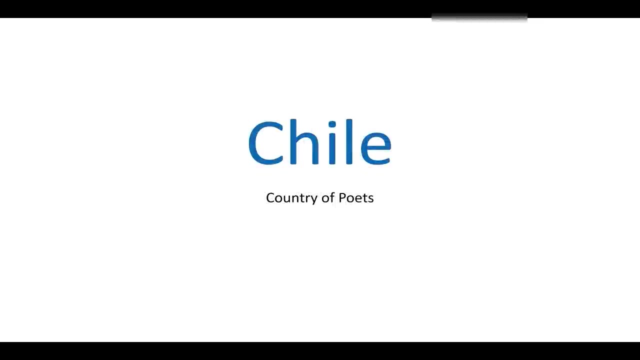 can also set some slide timing. So I could say I want the slide to advance after three seconds And click to apply that to all of my slides. Let's try it out. So if I click on my first slide and click this button to start my presentation, it loads up, I can see the title and it transitions. 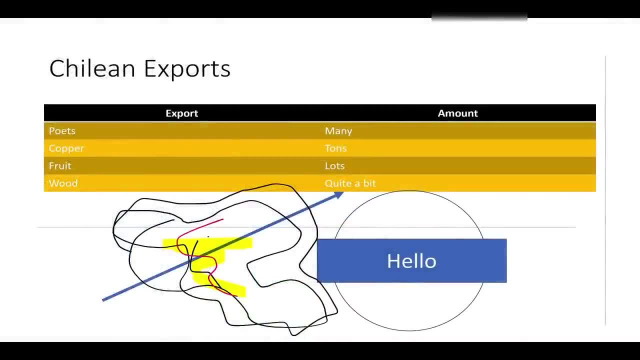 to the next slide And then, three seconds later, transitions to the next slide and then the next slide. Now, if you find that this is going a little too fast, you can tap the back arrow to go back, Or if it's going too slowly, you can tap the forward arrow on the keyboard to go forward. But in most cases, 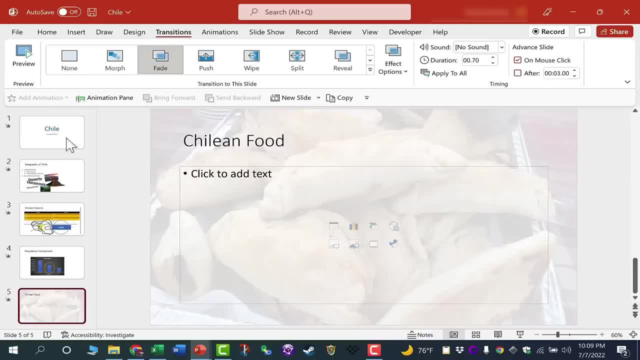 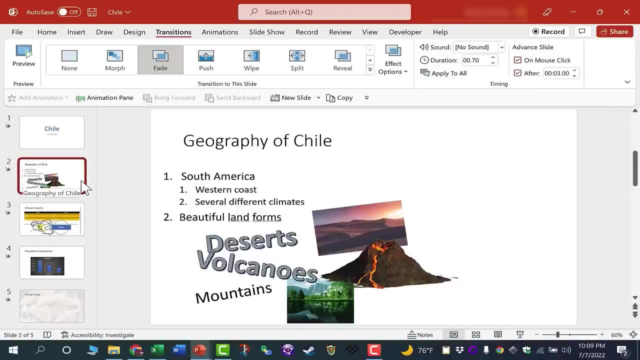 if you're going to use slide timing, you may want to set that on a slide by slide basis instead of applying it to all, And it's a good idea to rehearse those timings and practice so that you know that you have the right amount of time for each slide. The last refinement for our presentation that I 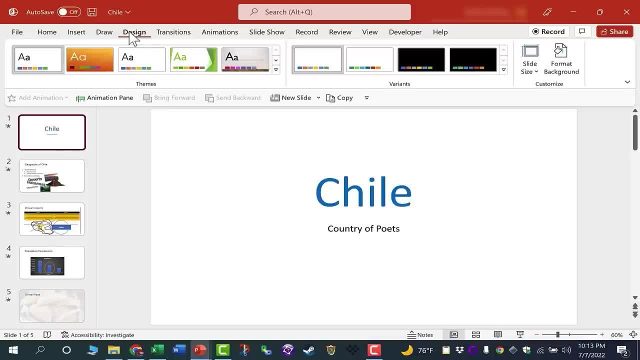 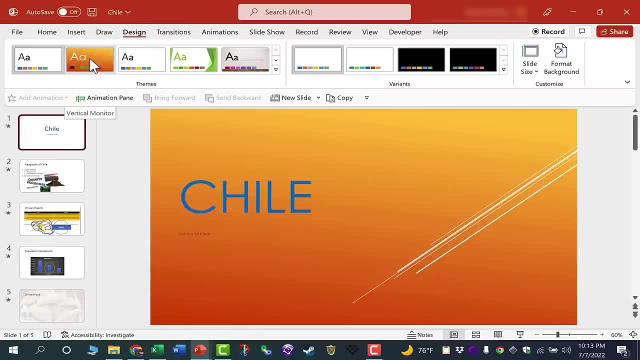 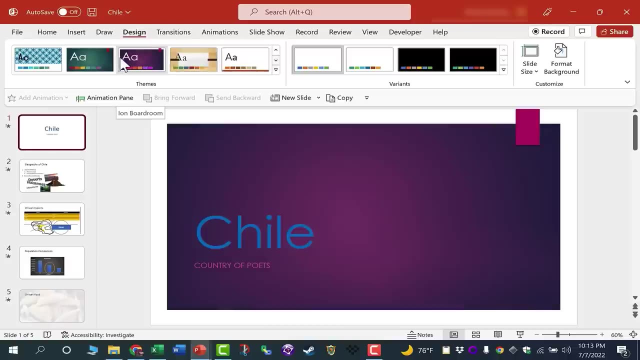 want to show at this time is how to add a theme to your presentation. If I go here to the design tab, notice that there are themes, And I can just put my mouse over a theme to see a preview of how that will look And notice that it changes- not just the color scheme and the background, but it also changes. 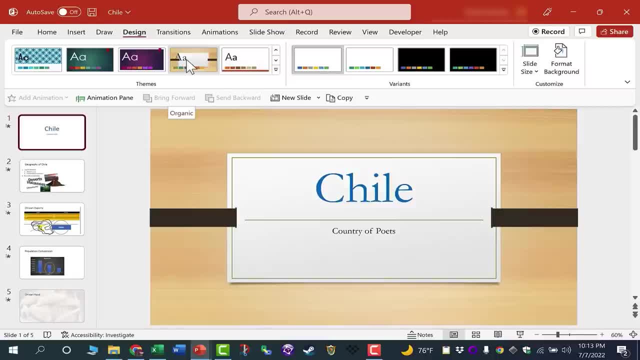 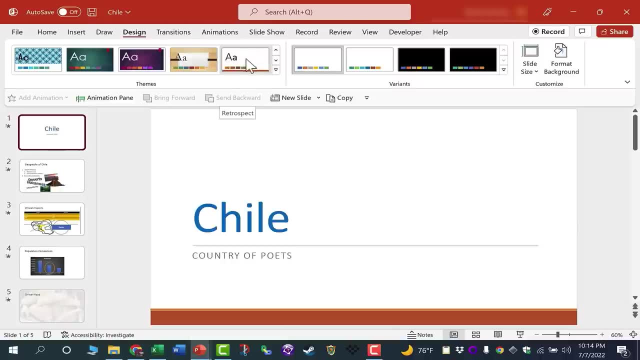 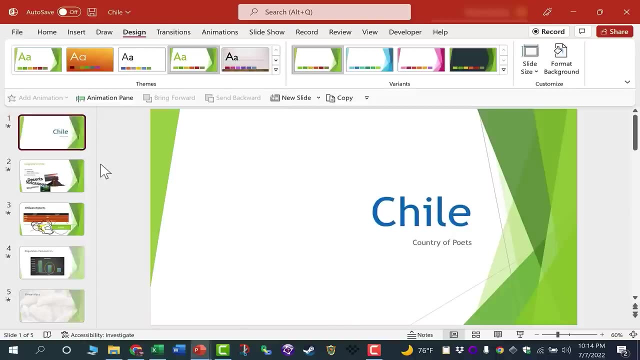 the fonts. It changes in some cases where the text shows up on the slide, So it's definitely important to think this through and make your decision about which theme, if any, you would like to use. You can click this button here to get even more themes, And for now, I think I'll just go with this theme here. 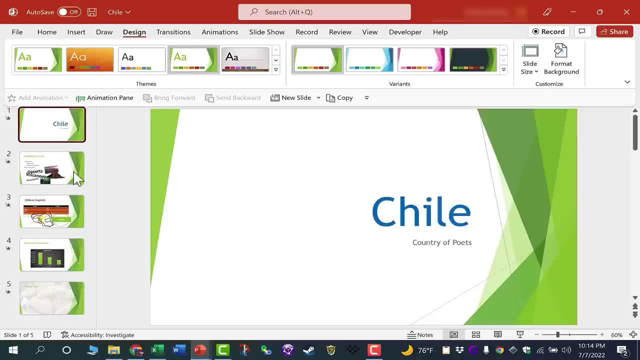 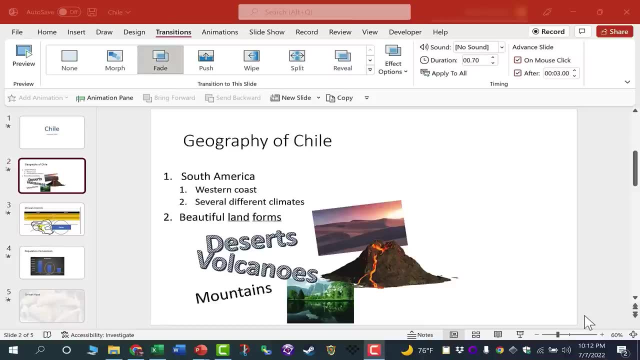 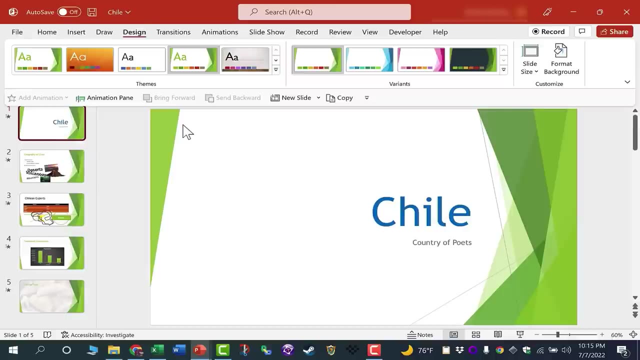 When I click, it adds it not just to the selected slide but to my entire presentation. So in this video we've looked at how to refine our presentations by adding background graphics, if we want to, to a slide, how to add transitions and how to add timing to slides. And then we also 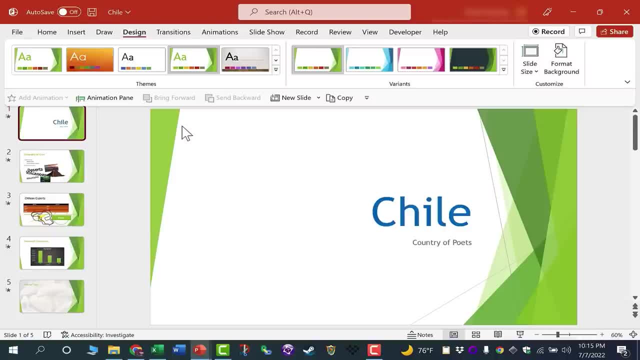 looked at how to add themes to our presentations. In this next segment of PowerPoint, for Beginners Complete Course, we're going to look at print and export options in PowerPoint. Let's say that I'm completely done with this presentation and it's ready to be shared and to be used in the classroom. 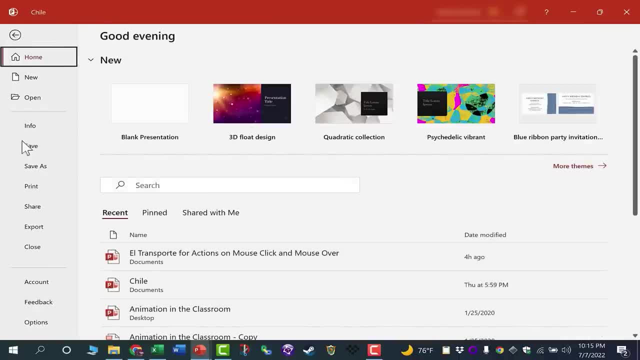 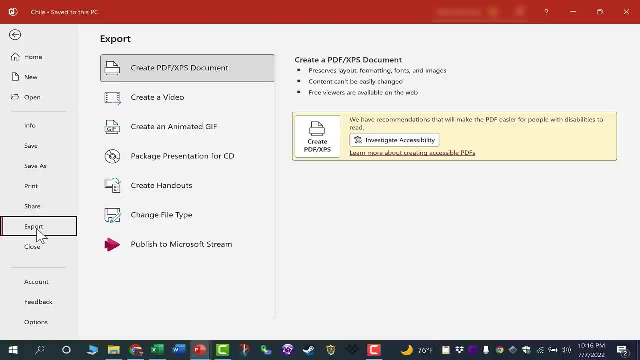 or the boardroom. I can click here file and of course I would want to make sure that I'd saved it. But in addition to that, I also have the ability to export. Now, when you select export, you get some really exciting options. For example: 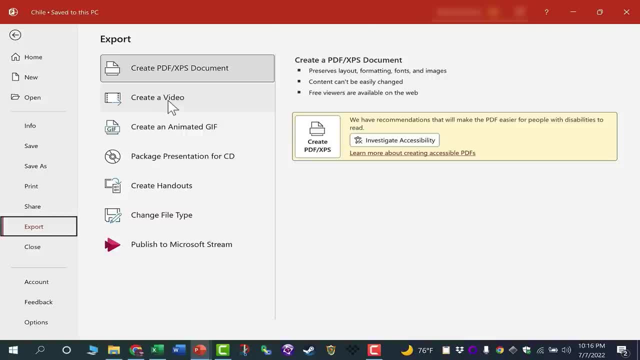 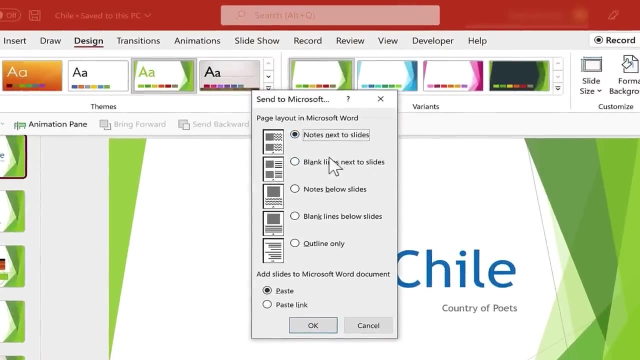 I can create a video based on this presentation that I've created. I could create an animated GIF out of it. I can also export handouts that go with the presentation. Let's try that. I'm going to click here on create handouts and I get to decide. do I want my notes next to the slides? 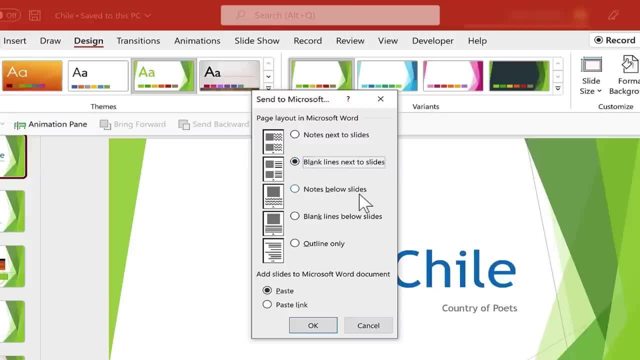 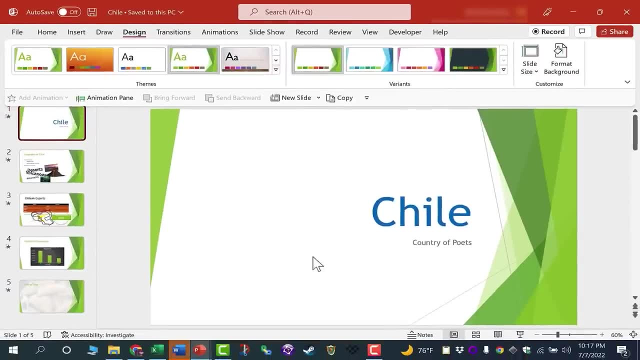 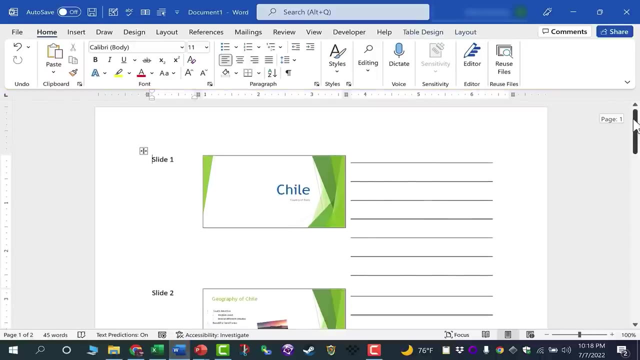 or do I want blank lines next to the slides, notes below the slides, etc. I'm happy with these selections and I'll click OK. And PowerPoint now is opening up Microsoft Word and it's creating handouts based on my slides. Let's switch to Microsoft Word and there I have my handout to. 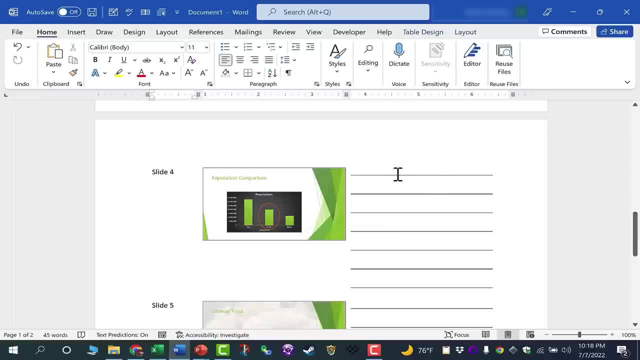 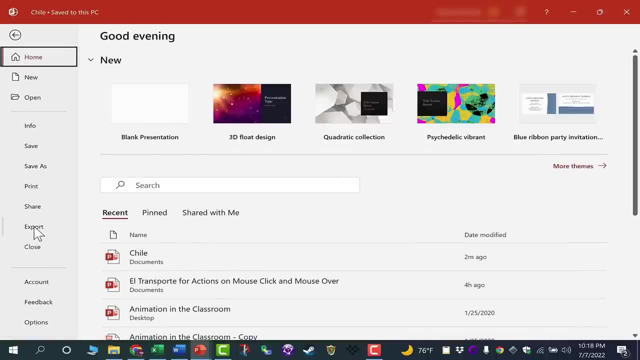 go with my slides. That way my audience can take notes on the provided lines. I'm going to switch back to PowerPoint and let's look at some of the other save, export and share options that we have. I could change the file type of this presentation. I could save it as a PowerPoint. 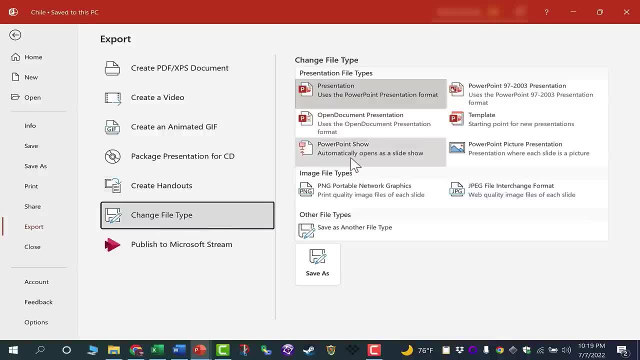 show, which will automatically open as a slideshow. It won't open in edit mode, like you typically see in PowerPoint. I could save it as a template or a picture presentation, and there are other options as well. Now, if I would like to see more options, I can click save as here, or I could click save as: 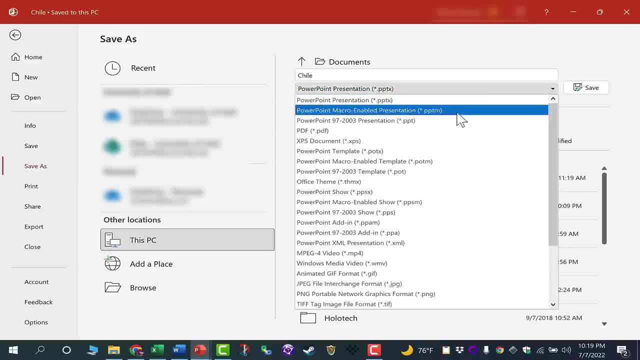 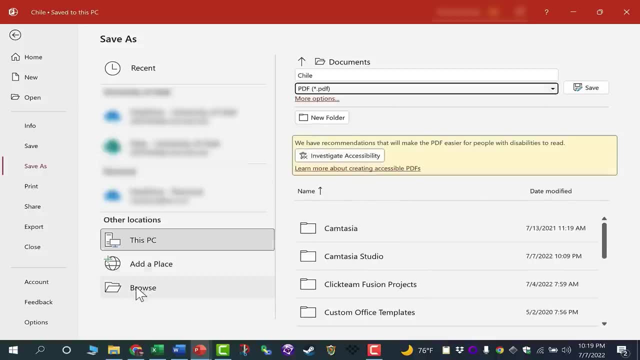 here and then go here to the PowerPoint. I can also save it as a slide show. I can also save it as a PDF. I'm going to go to this dropdown arrow and click and notice that there are many other options to choose from, including one of the most important, which is PDF. I'm going to save it in. 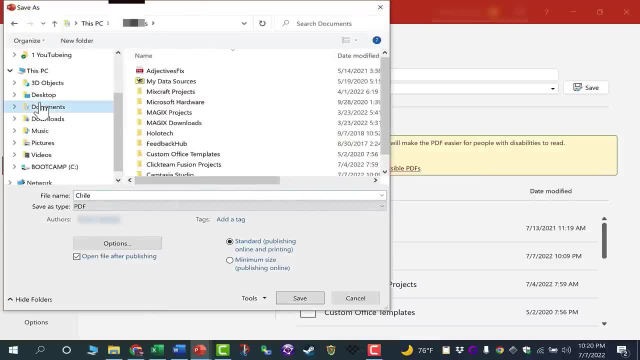 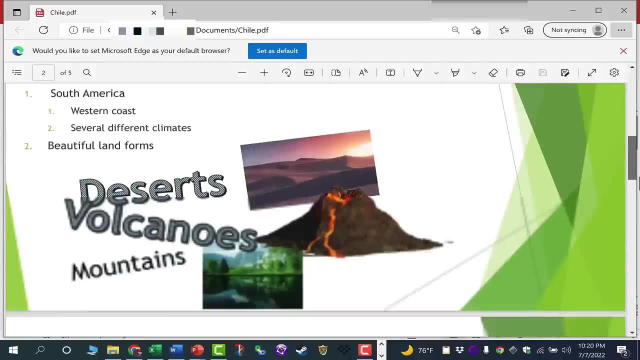 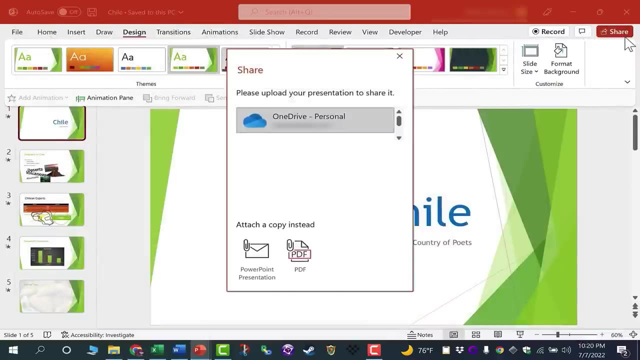 my documents folder, so I'll click browse, choose documents. it's got my file name and I'll click save. So here is my PowerPoint presentation about Chile, but it's in PDF format. I'm going to X out of that because I need to also show you that it is possible to upload this presentation using this. 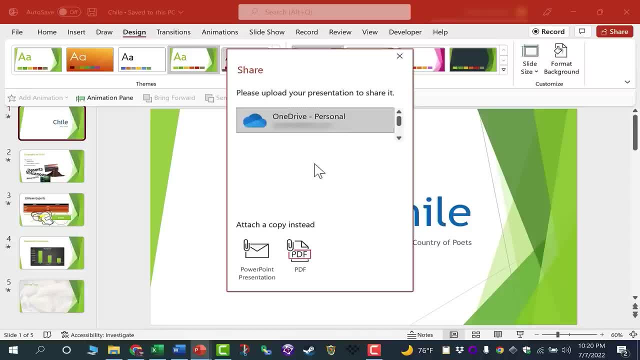 share button and I can upload it into my OneDrive account. Once it's in OneDrive, it becomes extra easy to share with people and to collaborate with people on this presentation. I can also choose to send this presentation as an attachment to an email. 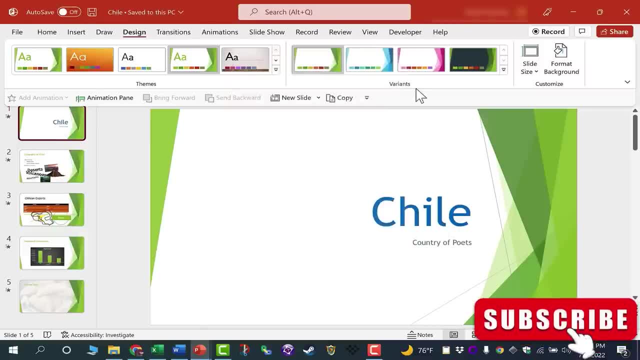 or as a PDF attached to an email. So those are some of the best and most useful print and export options in Microsoft PowerPoint. In this final segment of PowerPoint for Beginners Complete Course, we're going to look at how to deliver a presentation in front of an audience When it's 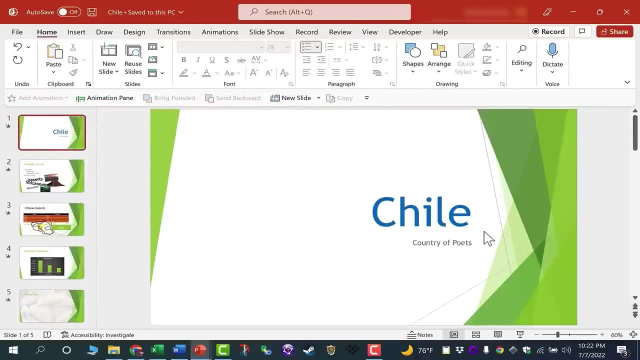 time to present. simply open your presentation and you'll be able to see the presentation in front of the audience. You'll be able to see the presentation as you normally would, and then you can go down here to the lower right corner and click this slideshow button, or you could go to. 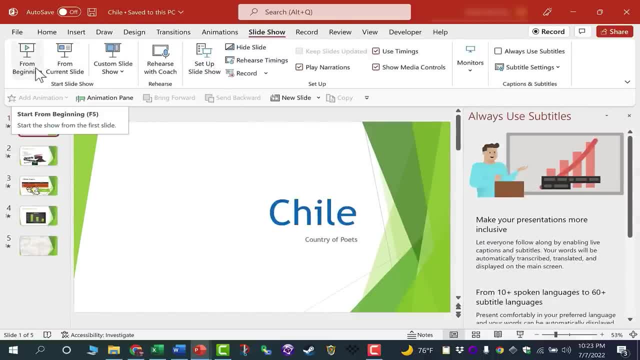 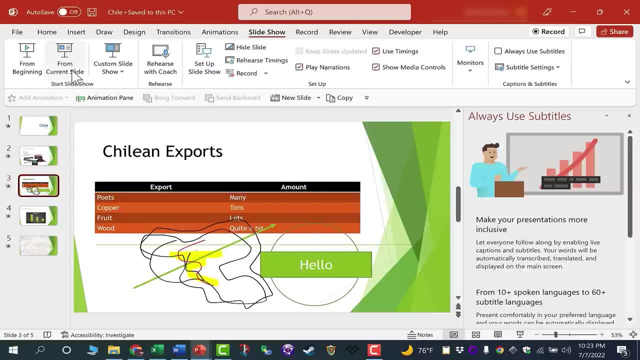 the slideshow tab and choose to run your presentation from the beginning or from the current slide. So, let's say, I'm on slide three and I want to start there. I could simply click from current slide. In this case, though, I want to start from the beginning, so I click there, and here's my 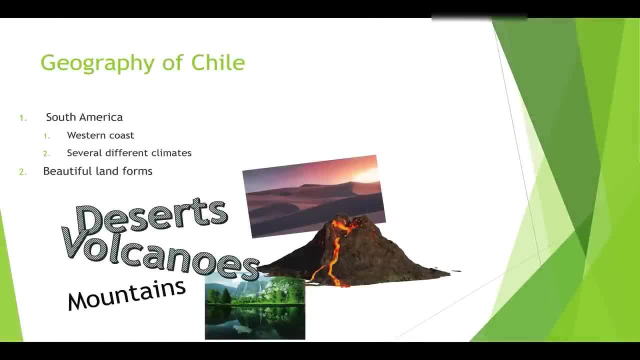 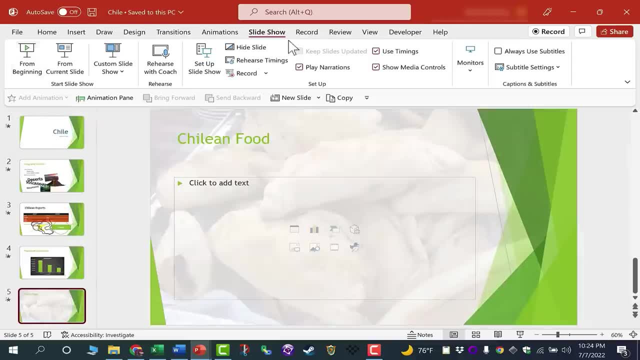 presentation, with its transitions, with the text boxes, the images, the tables, the drawings, the shapes, my chart, my background image and more. There are some other wonderful options here on the slideshow ribbon, including creating a custom slideshow and using Rehearse, with Coach rehearsing. 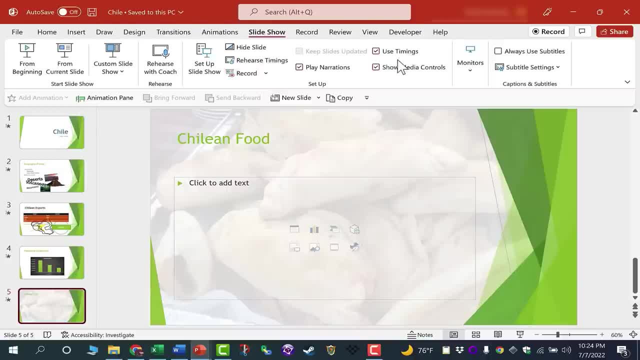 timings recording. There's so much more that we could talk about, but at this point you really have learned all of the information and techniques that you need to use PowerPoint effectively. So what are your next steps if you want to move beyond what we've learned here? The first thing I want